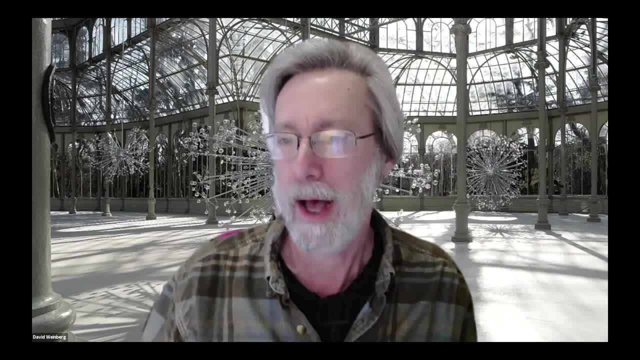 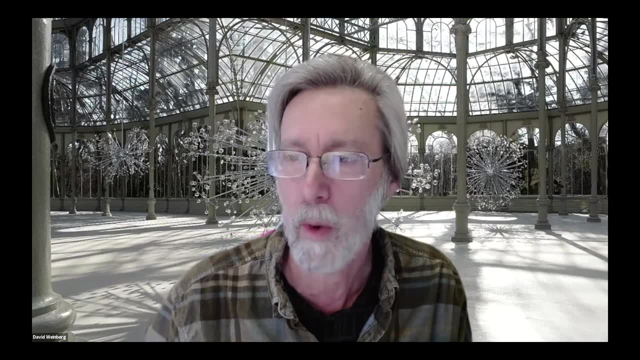 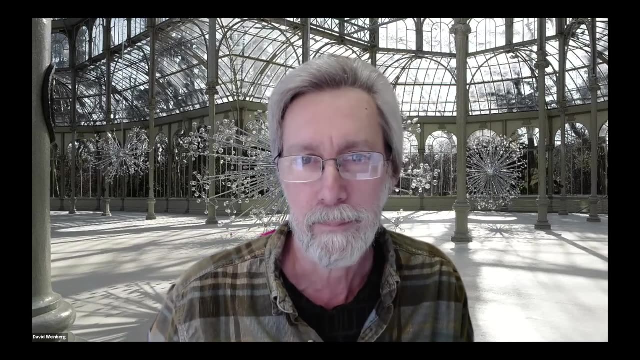 lot through Adam Leroy and the Thanks Project And I can look forward to a great talk. And I'll remind people that if you want to join our follow-up conversation, that will be at 1.30 pm this afternoon And Diederik, take it away. 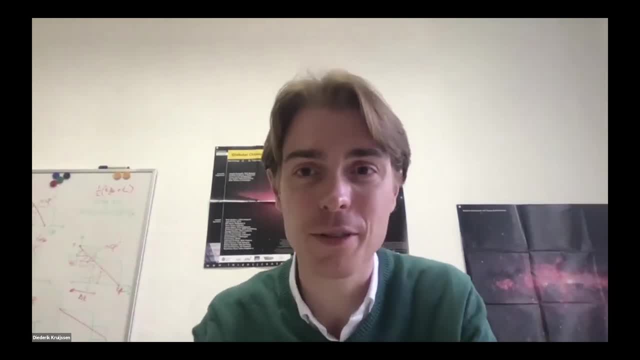 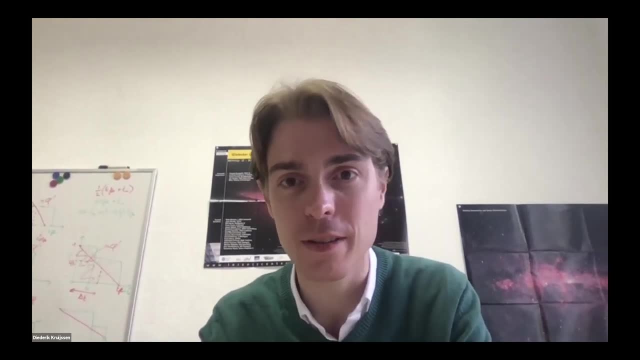 Thank you, David. Thank you very much for your kind and generous introduction And in particular, of course, also for the invitation. It's a little bit embarrassing: I've actually visited Princeton, So for me it's already a major step to do so virtually And hopefully. 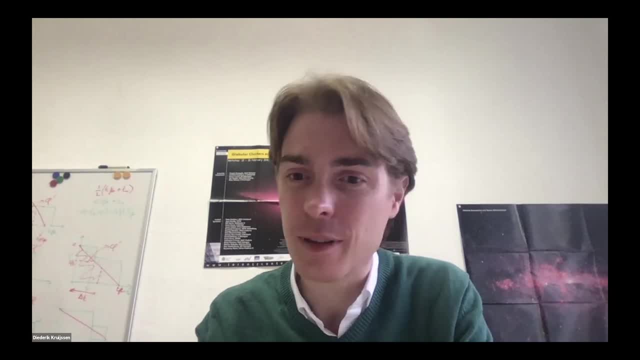 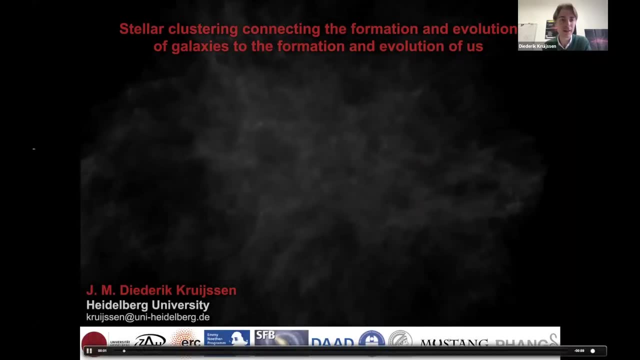 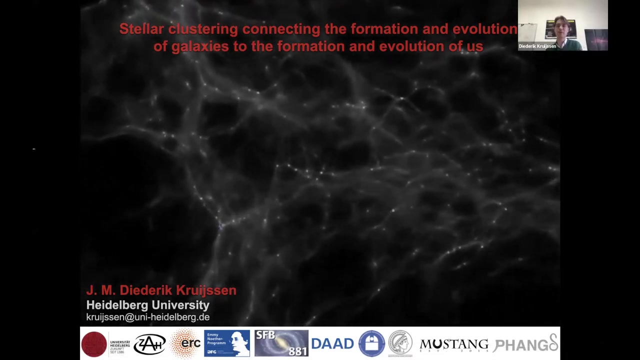 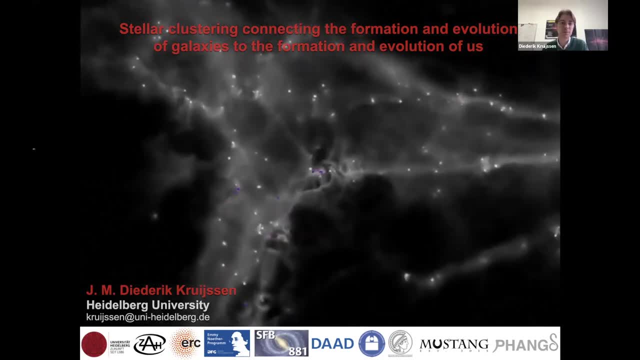 looking at- And I think that's something that we should be looking at, And I think that on the tip of my hat- is that the transition between the solar system and the galaxy has shaped our origins, basically from the formation and evolution of galaxies like the Milky Way. 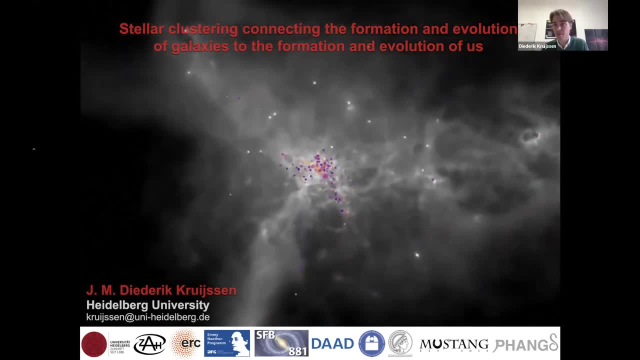 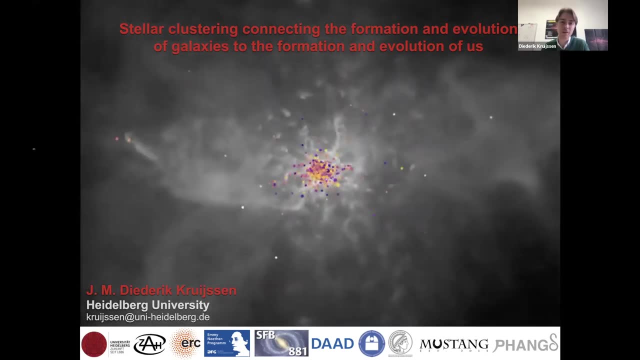 to the formation and evolution of planetary systems like our solar system, And of course that is a somewhat ambitious goal for even a single colloquium. So this is going to be somewhat eclectic, And what it also means is that basically each of the topics I will 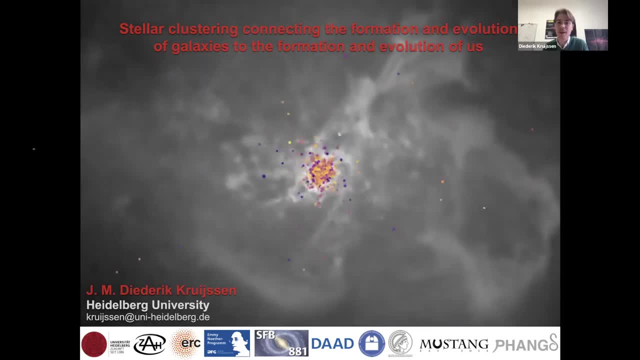 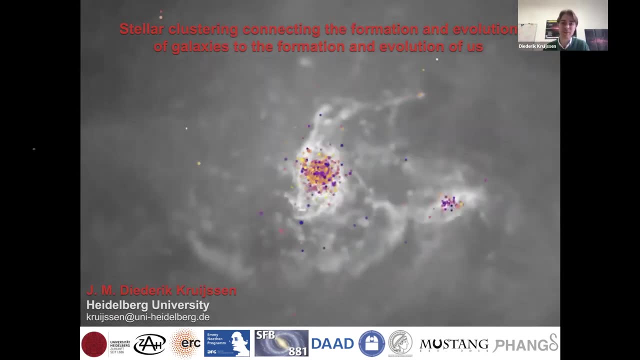 touch on. I could probably have given an individual colloquium on, So there will be a little bit bit of scope at the expense of depth. but I'm very happy to try and deepen the discussion, either during the discussion afterwards or the session we'll have later today. 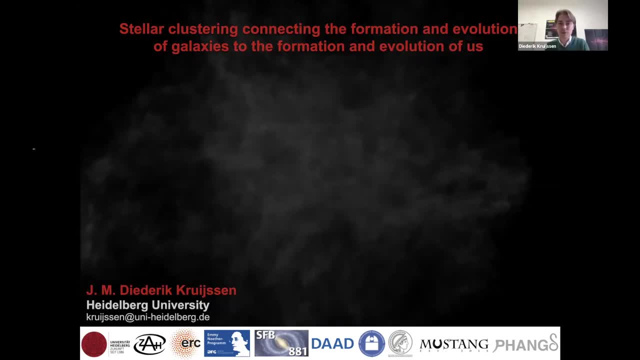 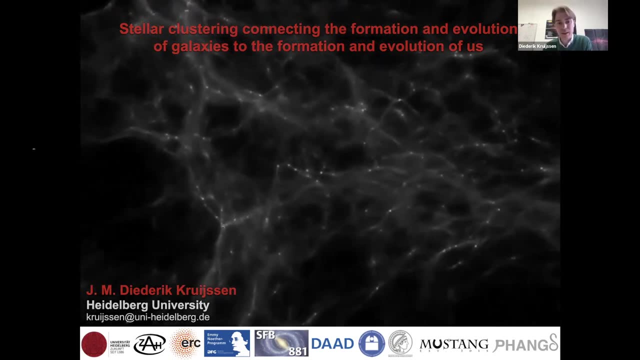 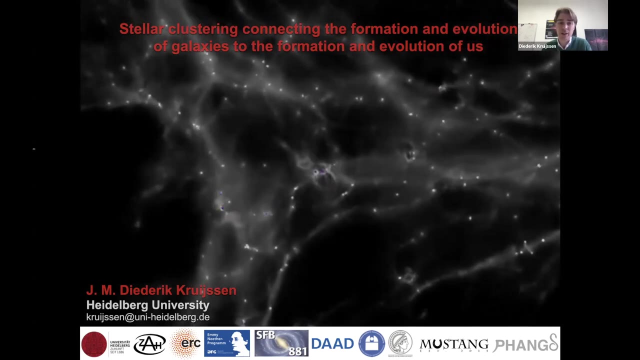 Yeah. so why would you want to try and connect all of these things? Because, in a way, that is what astrophysics does at large, and it might seem overly ambitious to try and do that, but I think it's relevant and there have been a number of recent developments, mostly observationally. 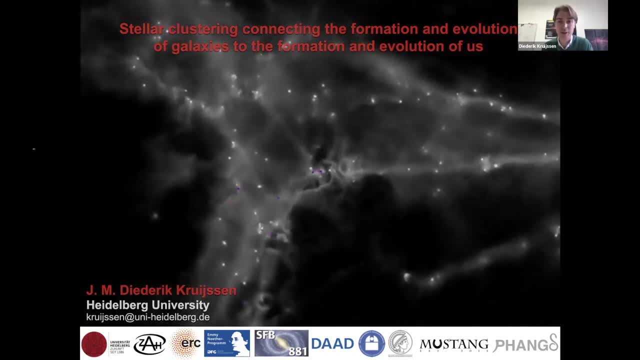 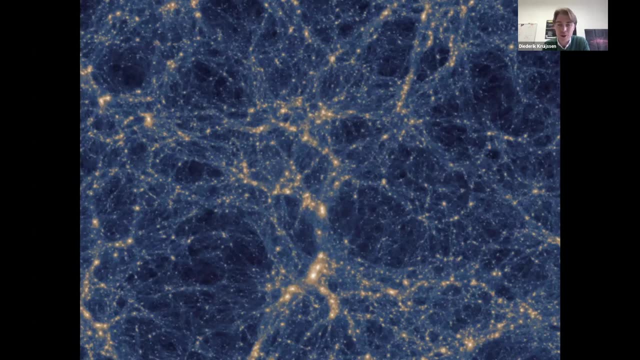 but also computationally, that now allow this, and that's why I'm excited to share that with you today. And the story basically starts when you look at a very large cosmological volume like this. and we've all seen these images, and the way I tend to look at them is actually not just looking 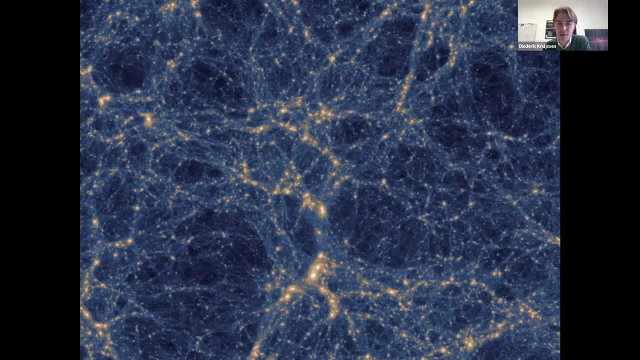 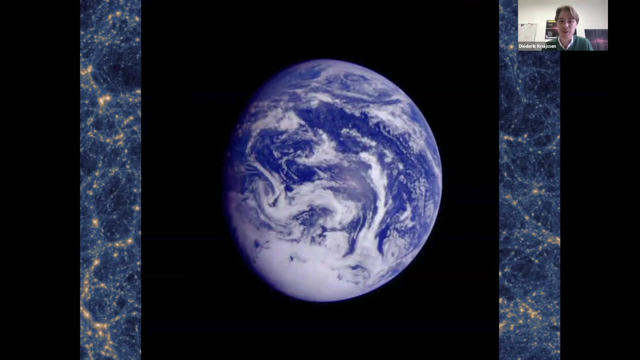 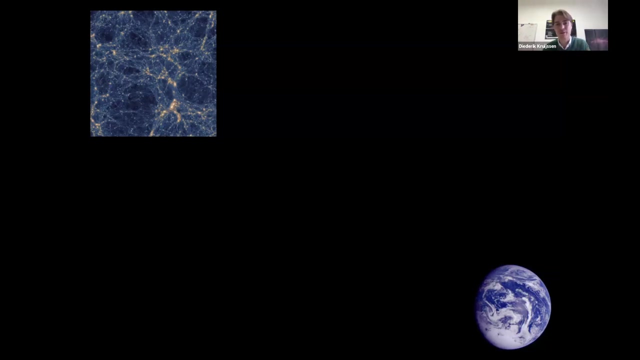 at the dark matter distribution like we do here. This is actually illustrious TNG, but I try to imagine that every pixel here contains countless planets And of course, there's a huge dynamic range in between. In fact, if you do the math and you compare the size scales this enormous sort of gap in between. 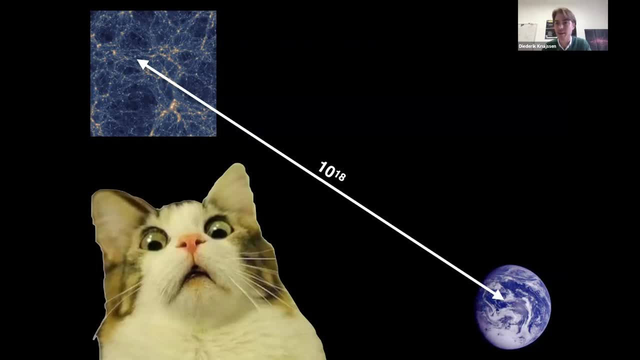 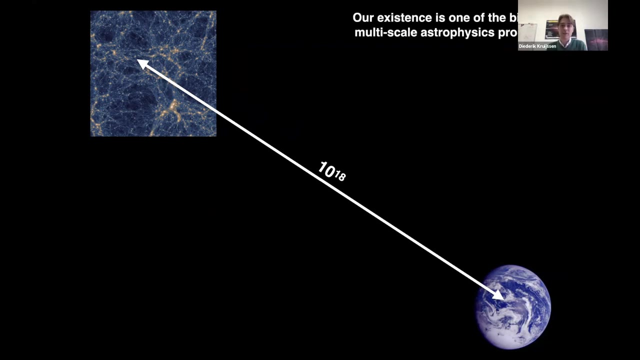 spans 18 orders of magnitude, which is an intimidating scale, an intimidating dynamic range, But thankfully, you know, if we look at the astrophysics at large, we can cut this up into multiple chunks that are actually quite manageable, And that allows us then to start addressing this question. is okay. how do we go from the cosmic web? 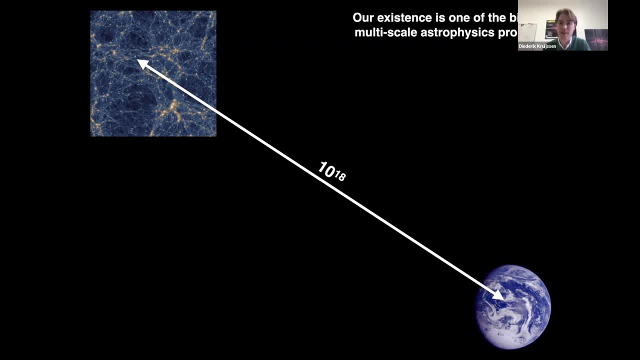 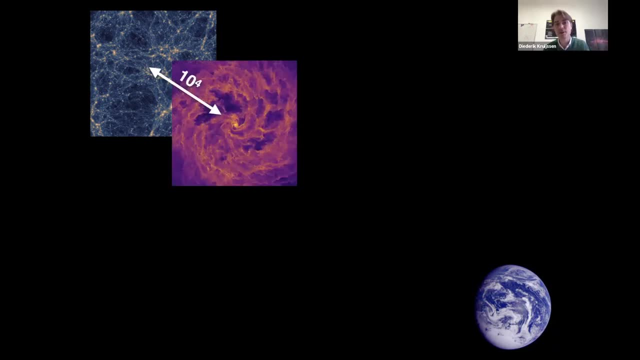 to planets like the Earth, And that gap makes our existence one of the biggest multi-scale astrophysics problems. And you can address that by making small steps. So the first one you can take is basically going from the cosmic web to individual galaxies, And the step made here is of the order 10 to the 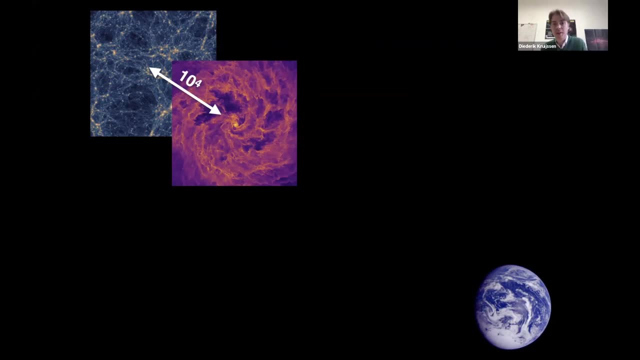 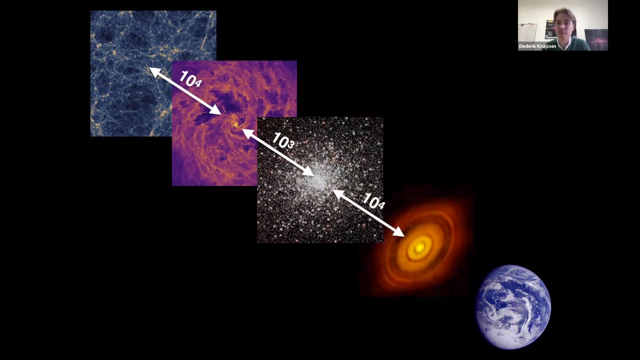 4 in spatial scale. From those galaxies you can take a step further down to individual stellar clusters within those galaxies, which are another factor of a thousand smaller. And then within those stellar clusters, of course, you've got stars which, when they form, have protoplanetary disks around them which are another factor of 10 to the 4 smaller than the cluster itself. 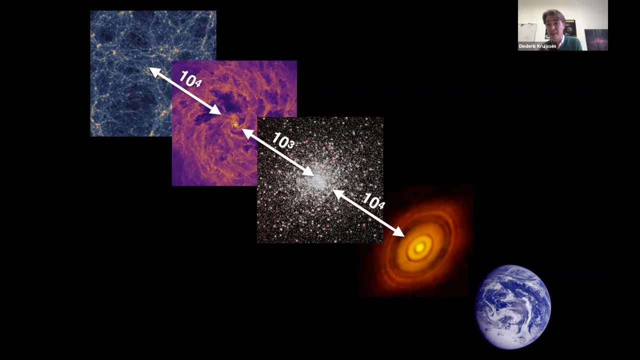 And I don't know about you, but in my mind at this point I'm nearly there. right, I'm nearly at the planet. It turns out there's another 10 to the 7 going from a protoplanetary disk to an Earth-sized planet. 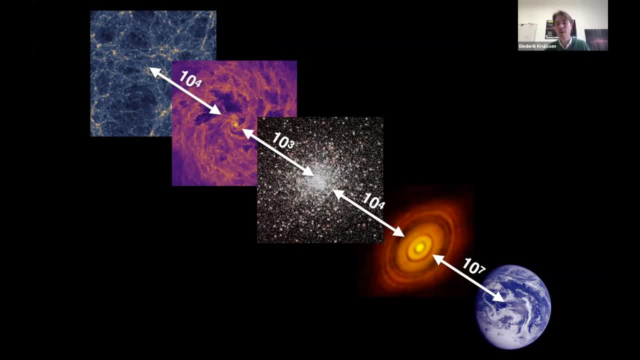 So this is really a vast range of scales, But it turns out they're all connected And the way they are connected is actually revolving around the stellar clustering which I've put in the middle here, And the stellar clustering is essential in many ways. So, towards larger scales, 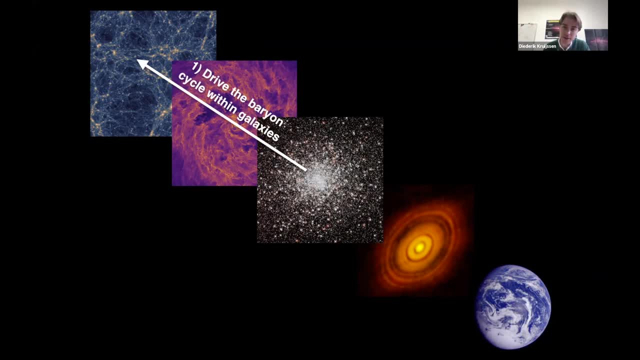 stellar clustering drives the baryon cycle within galaxies. The fact that star formation is clustered and sources of stellar feedback within galaxies are clustered, turns out, is a really critical element of deciding how galaxies grow their mass, both in both in gas and in stars eventually, but then in turn, the long. 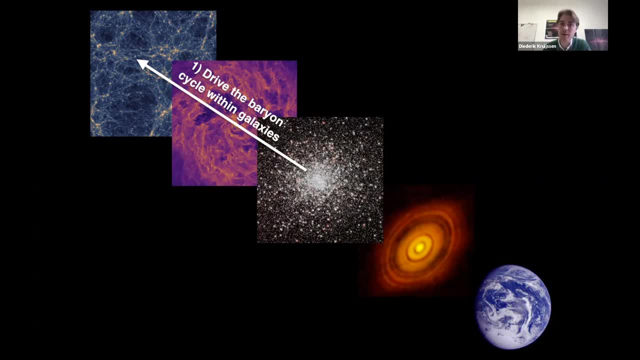 lived relics of stellar clustering. globular clusters allow you to trace galaxy information and assembly because they basically have in, they carry an imprint of what the conditions were of the star formation, the feedback, the galaxy information assembly at the time of their own formation, and i'll talk a little bit about that as well, showing basically how we can learn. 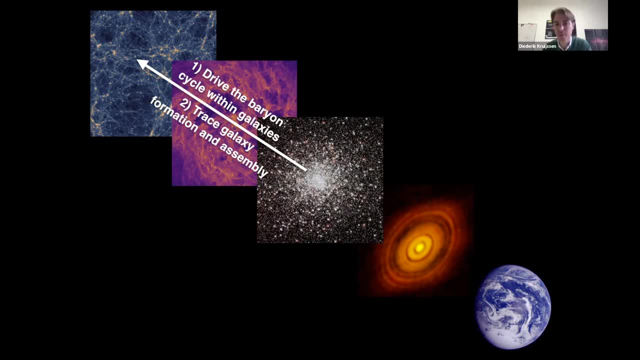 to use that to reconstruct the assembly history of the milky way. now we then start zooming in towards smaller scales. stellar clustering is an important factor in perturbing and destroying protoplanetary disks and, depending on the time scales on which this happens, it can actually leave an imprint on the 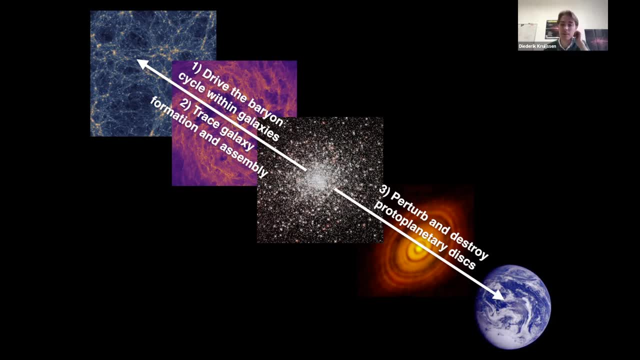 planet formation process in the planet population. and then, finally, what i'll discuss towards the end of the talk, is that stellar clustering actually modifies the properties of the planet population. i think if we bring all of these things together, we start to see a picture in which all of those scales are indeed. 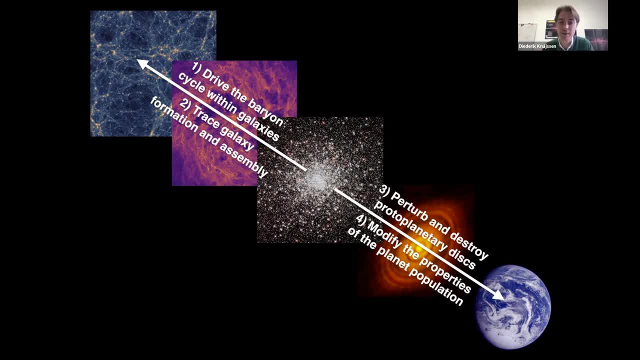 connected and it's an enormous challenge to try and make this tractable, try and make this understandable. so i'll start with the first one. in terms of how does stellar clustering drive the baryon cycle within galaxies? can we somehow try and identify fundamental units within galaxies? 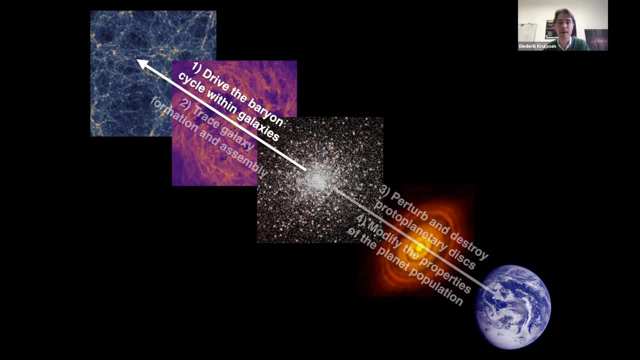 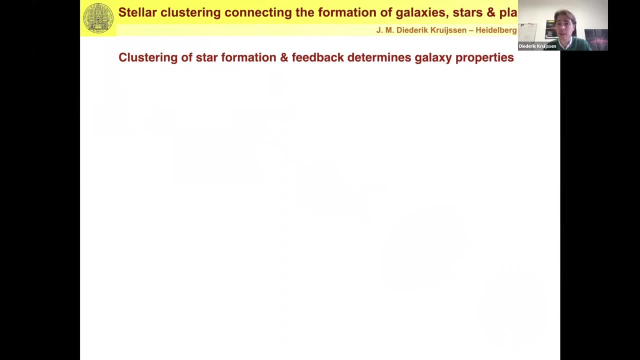 that are sort of the important chunks in driving this baryon cycle, and from the numerical side and numerical simulations. this is actually a very extensively studied problem, so i'll show two examples here of showing how important the the small scale baryonic physics of star formation. 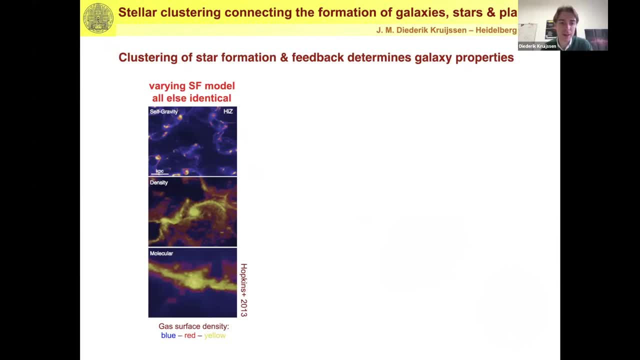 and feedback are- and the first here is here on the left. it's already quite old. there's a study by phil hopkins from 2013 where he simulated exactly the same initial conditions with exactly the same physics, except for the star formation model. so in each of those three panels there, 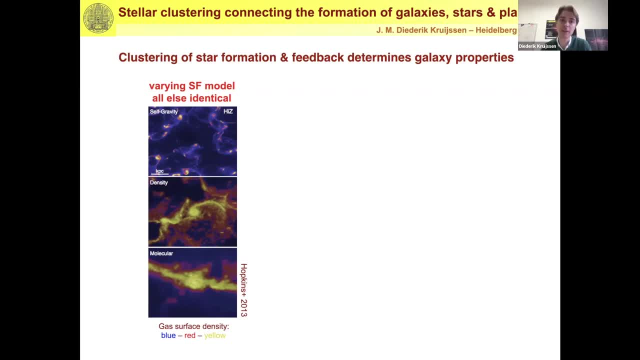 were different conditions that the gas needs to satisfy in order for the star formation model to satisfy in the simulation in order to be converted into stars, in the top panel the gas needs to be self-gravitating. in the middle panel it needs to be above a certain density threshold and in 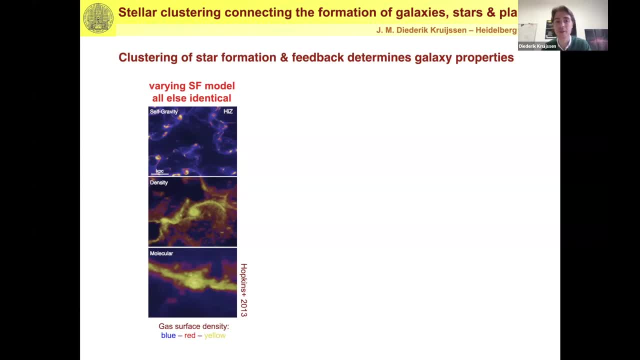 the bottom panel. it needs to be in a molecular state. that's the only difference between these simulations. you'll see that there are qualitative differences in terms of how these galaxies are structured. now, here on the right, i'm showing work by ben keller, who's working with us here. 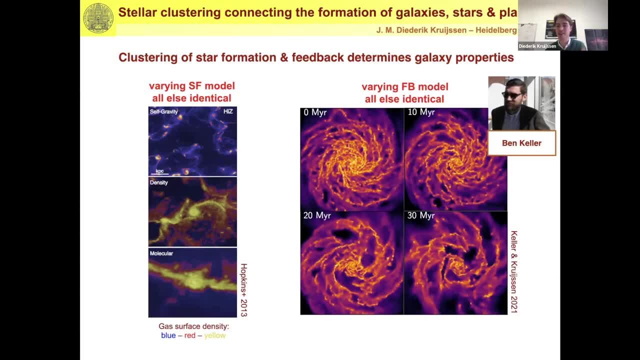 in heidelberg, who's basically been simulating the same galaxy. the only thing that we can do is simulate the same galaxy, but the only thing that we can do is simulate the same galaxy. but the only thing that we can do is simulate the same galaxy, but the only thing that he varied here. 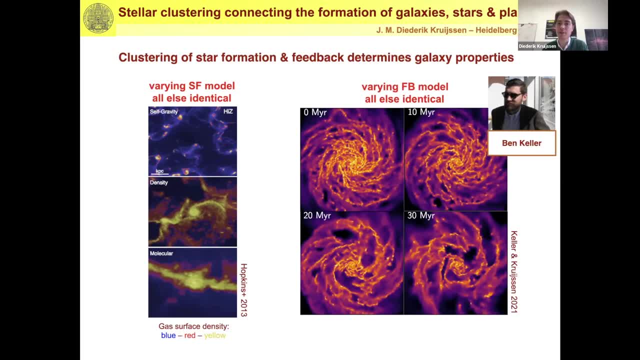 is the supernova delay time. so in the first panel supernovae detonate immediately when a star particle is born, whereas in the bottom right panel they detonate about 30 mega years after the star particle is born. now this is of course it's ad hoc, but it demonstrates how important it is. 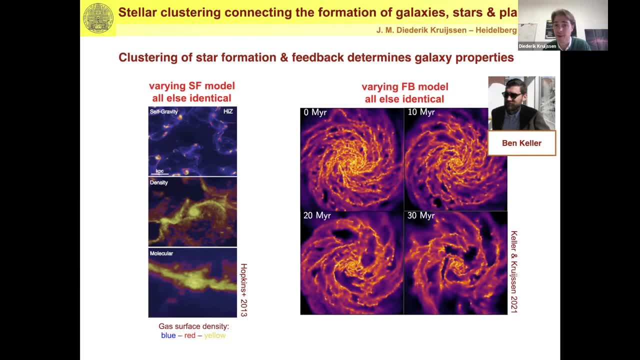 to get the small scale details of stellar feedback right in order to reproduce or in order to get a predictive model for what your galaxy structure should look like, and the reason that this is so important is that many of the choices that are made here actually make a 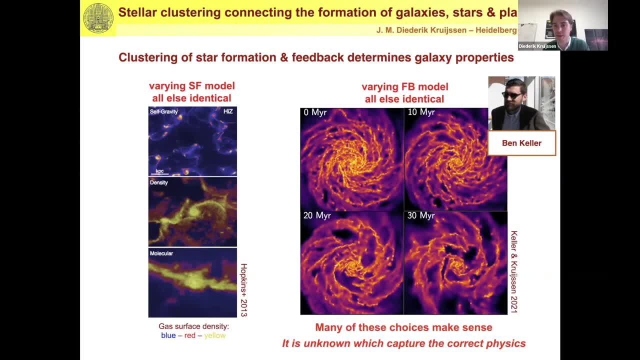 lot of sense, and we don't know which of these captures the correct physics, and that means that, in order to address this, what you need is actually you need empirical answers to these questions. what should we be using in numerical simulations? and this is really a really complex 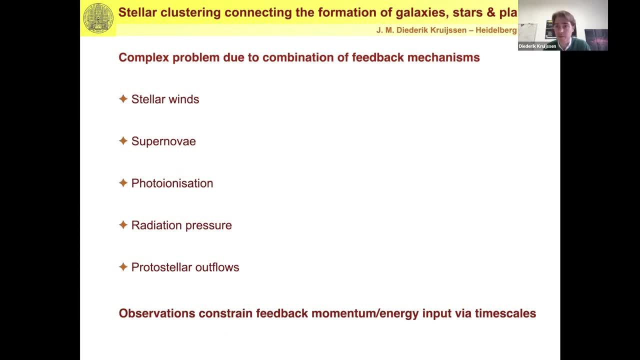 problem because stellar feedback is a combination of a bunch of different mechanisms and, even worse, it's a non-linear combination. so stars exert feedback on their surrounding medium through stellar winds, through supernovae, which i already mentioned, but also through photoionization, photo evaporation, radiation. 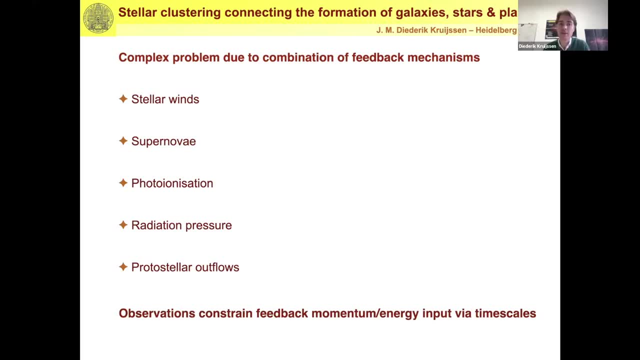 pressure, protostellar outflows and the critical element here is really all of these feedback mechanisms- except maybe supernovae, but for stellar population still act in terms of rates of energy and momentum deposition. so in order to constrain these, what you really need is an observational 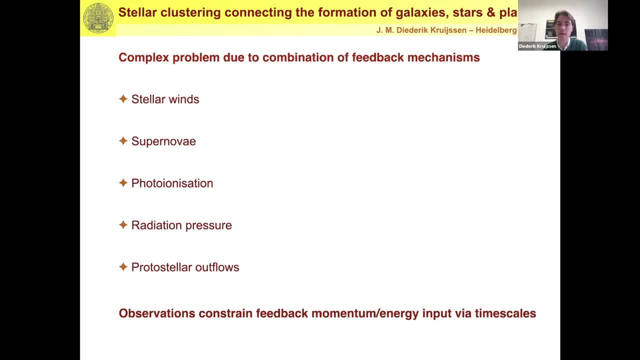 measurement of the time scales on which the stellar feedback affects the surrounding interstellar medium. of course, this is extremely challenging. if we're lucky, we get to live 100 years- not at all the time scales over which these feedback mechanisms act. so you need to use some form of statistical inference to try and understand this. 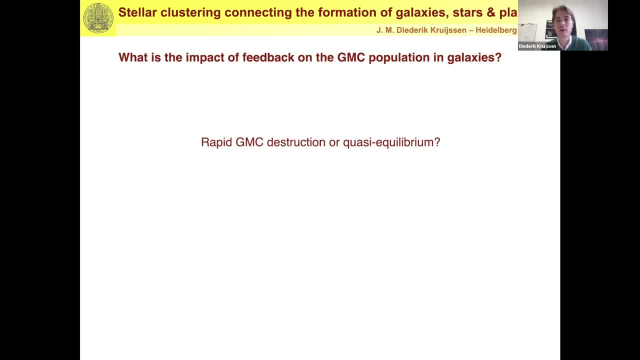 basically, if we reduce this to a very fundamental question, is we want to know what the impact is of stellar feedback on the giant molecular cloud population in galaxies, on interstellar medium, we're effectively reducing the question to: okay, if a giant molecular cloud is forming stars, do these stars, are these able to destroy that molecular cloud quickly? 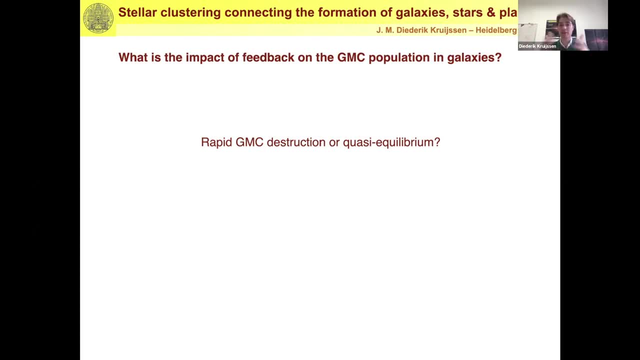 or are they basically just bubbling away? is that molecular cloud sitting there, forming many generations of stars, which would lead to a very quiescent evolution of a galaxy? a galaxy would have a very different morphology, as we saw earlier when we looked at the supernova delay times. 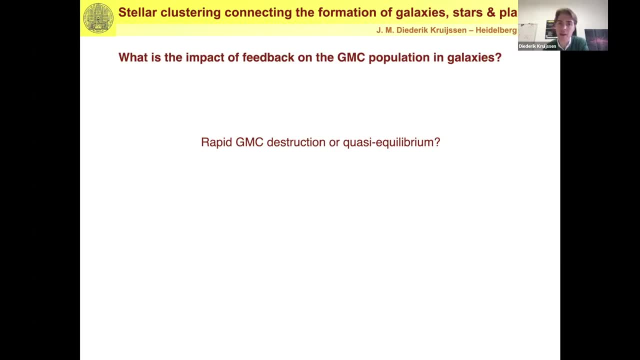 how big that impact is on what a galaxy looks like. so rgmc is destroyed rapidly. or are they in some form of quasi equilibrium between star formation and feedback? now it turns out that this actually the this question, this nice dichotomy leads to two distinct empirical predictions. so 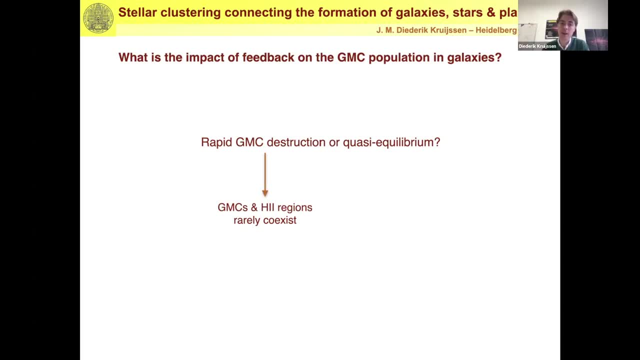 in the first. if molecular clouds are destroyed quickly, the molecular clouds and h2 regions, which is where the young stars are sitting, should rarely coexist. basically, if they're formed at gmc, you get your young stars, the young stars blow up the gmc and all you've got. 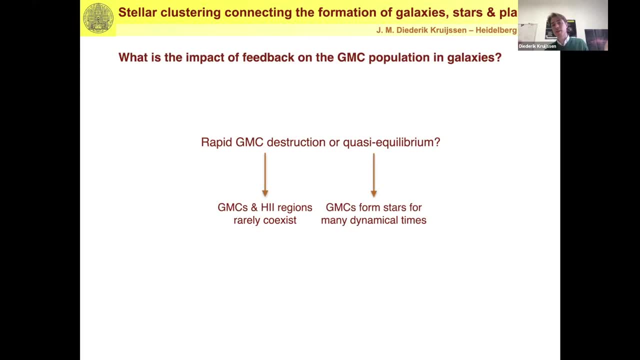 are those young stars. now, if gmc's exist in this sort of quasi equilibrium between star formation and feedback, then gmc's would form stars for many dynamical times and it means you would see molecular clouds and h2 regions in the same spots pretty much all the time. now this is 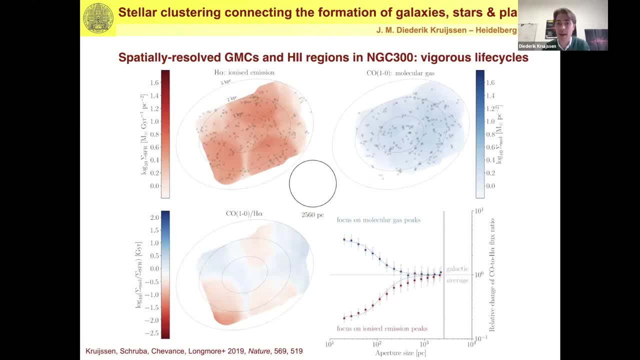 something we can now test with alma, and this is a paper we published about two years ago and i'm about to show. this is a paper we published about two years ago and i'm about to show an observational movie doesn't happen often, so i'm quite excited that. 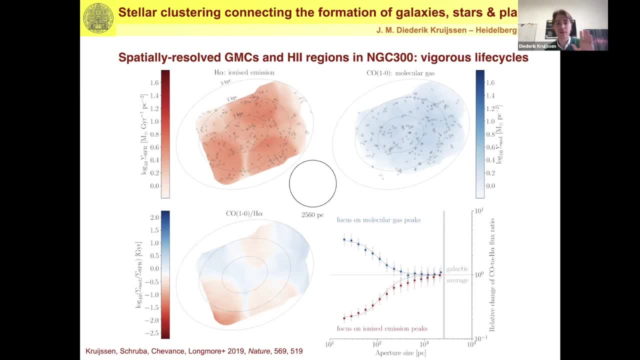 we made an observational movie. in the top left panel you see h alpha emission in nearby galaxy, ngc 300, and h alpha is tracing the young stars, which is massive stellar emission. the top right panel is showing the co. so it's a molecular gas that traces the molecular clouds. 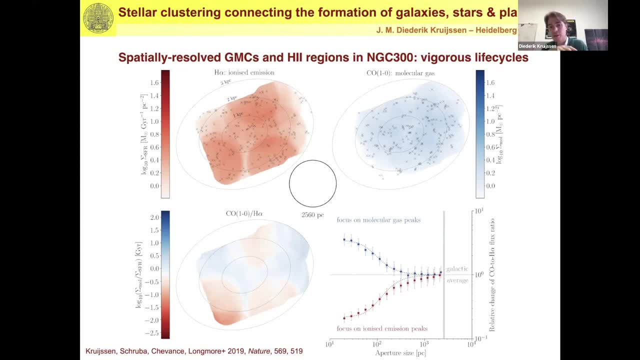 and in the bottom left panel you see the ratio between the two. so it's effectively the gas mass divided by the star formation rate, and the star formation rate is the ratio between the two galaxies and the star formation rate, and the star formation rate is the ratio between the two galaxies and the star formation rate. 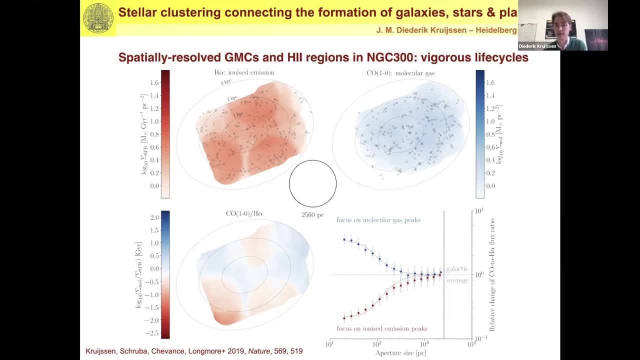 and i'll get back to the bottom right panel in a bit now. at the moment, everything is convolved towards the large scale on which we know that all galaxies have roughly the same ratio between molecular gas mass and star formation rates. the question now is, as we start zooming in, 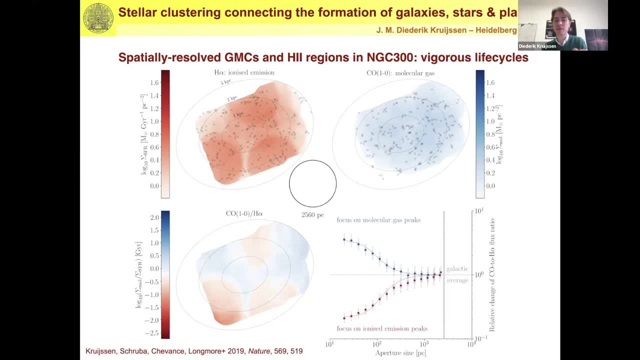 are we going to see h alpha and co emission in the same place or in a different place? because that'll tell us what happens to these life cycles and in the bottom left panel you'll be able to see this as if you're sitting in the same place. it's roughly white. 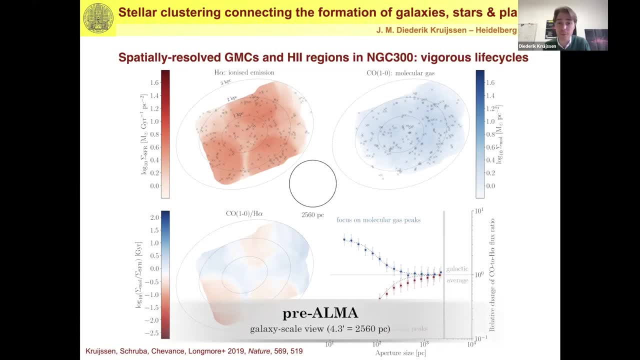 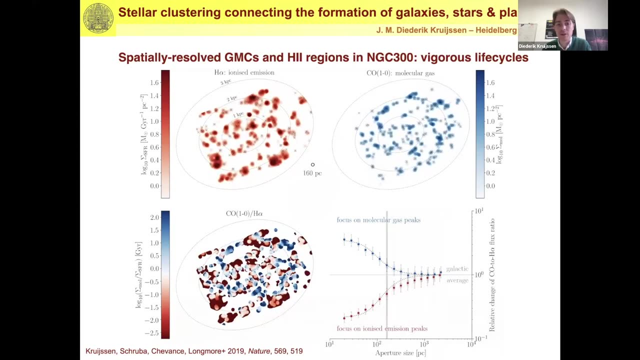 and if it's not in the same place, it's going to be bright red and like bright blue. so now the movie starts playing and we're increasing the resolution and the bottom left panel shows us unambiguously that we get bright blue and bright red regions. 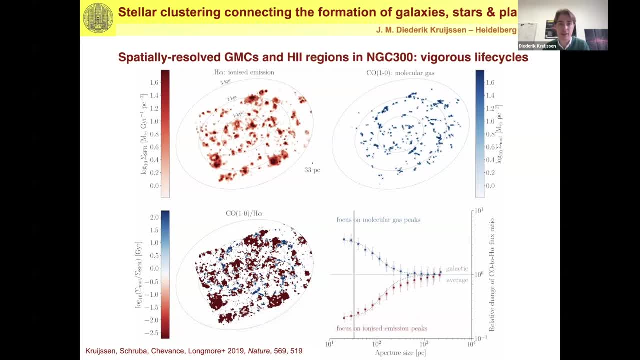 what this means is that the molecular cloud life cycle in this galaxy- here ngc 300- is rapid and that stellar feedback destroys molecular clouds very rapidly- and the bottom right panel is basically another way of of showing that here- as a function of the resolution of the galaxy. 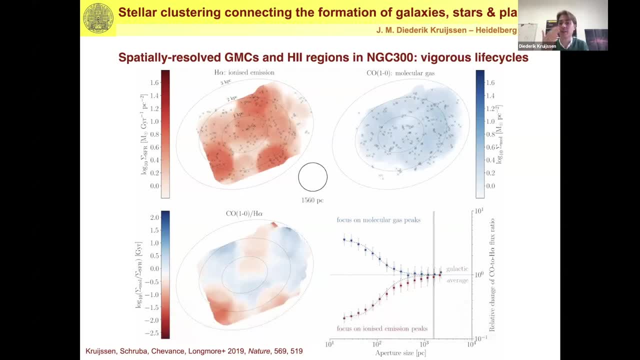 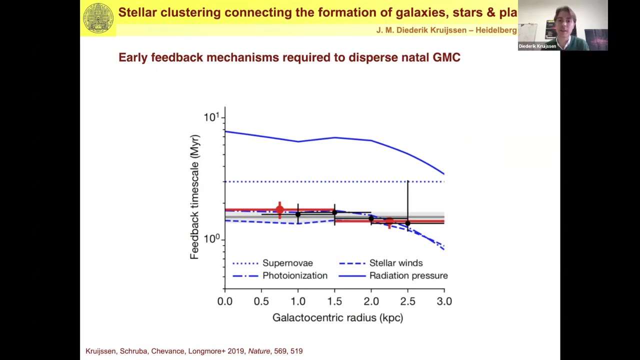 and the bottom right panel shows us how the ratio between the co and h alpha emission, changes between the co and h alpha emission, changes around co peaks and around h alpha peaks. so what we learned to do with this sort of de-correlation between co and h alpha emission? 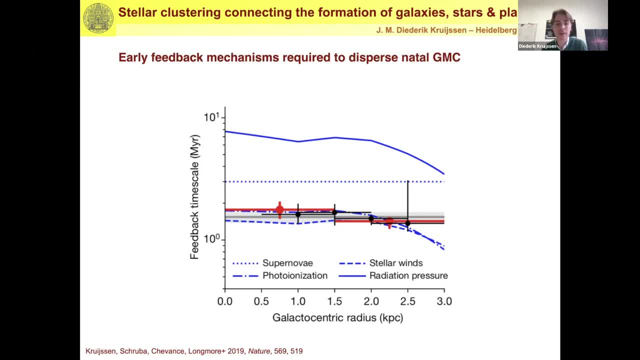 is to actually interpret that in terms of time scales, and i won't get into the details here of how we did that, but you can basically, as a function of the underlying time scales, you can predict how this diagram here in the bottom right how that will look like. so the dotted lines that you 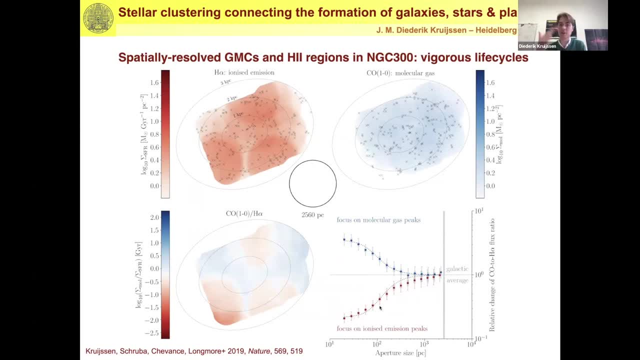 see here are basically our statistical model. that is a function of just the underlying time scales, and that way you can measure how long the co and the h alpha coexist. what that, what that tells us, is: how long do the massive stars need in order to blow up the parent molecular cloud? 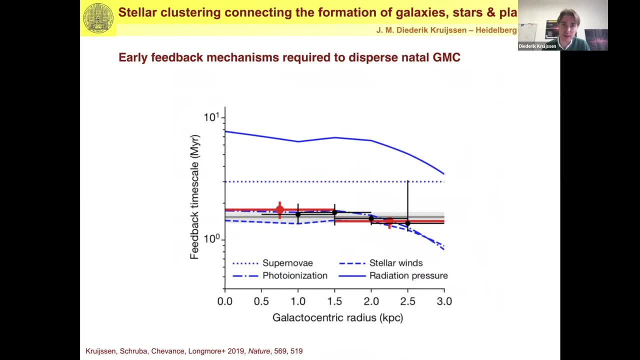 and that time scale is basically what we here call the feedback time scale and that is shown on the y-axis. so the feedback time scale is the time that the massive stars need to disrupt the parent molecular cloud, and the data points here show that measurement as a function of galactic. 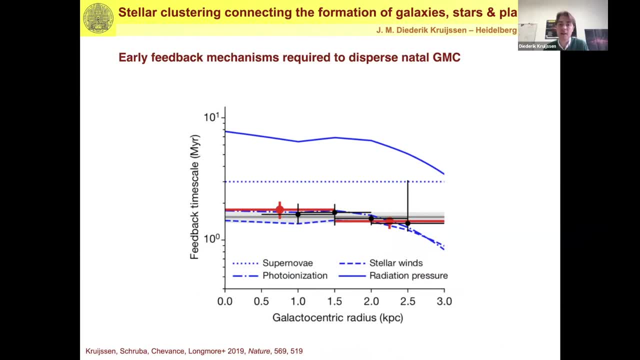 centric radius in this galaxy and you see 300, and it's compared to the analytical predictions that we would make for different feedback mechanisms. now, what we see here is that the time scales we get are short. they're of the order one or two mega years, so massive stars appear and they blow up. 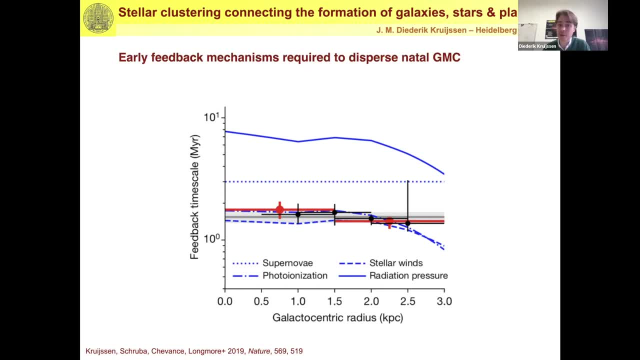 their power and gmc very quickly, and that's what we're trying to do with this diagram here- is to see how long the time scales are going to last, and that's what we're trying to do with this diagram. and that's well before supernovae would have a chance to blow up to affect the parent cloud. so 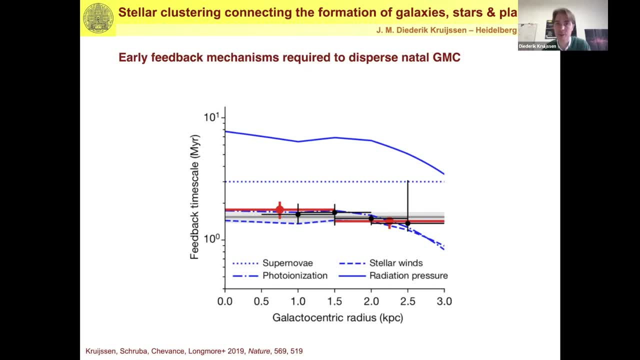 what this means is we need early pre-supernova feedback mechanisms to disperse the giant molecular cloud. in particular, it looks like photoionization and stellar winds are potential candidates for doing this. now, this is for one galaxy. we can now do this with alma, for a large. 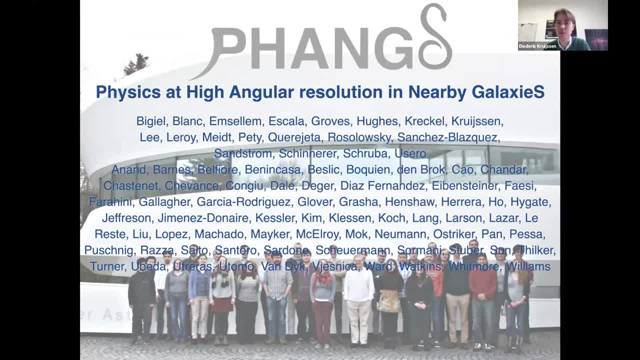 part of the nearby galaxy population. so there's what david mentioned. we're doing this, among others, in collaboration with adam leroy, and we're going to do this with the galaxy population. so we're going to do this with the galaxy population. so we're going to do this with the galaxy population. 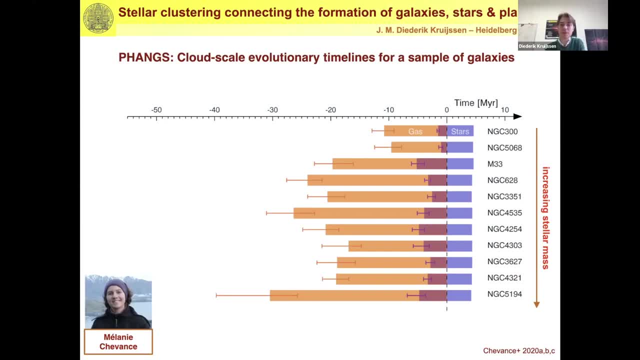 and this is work led by melanie chevron, who is a postdoc here working with us in heidelberg, who's done this for a first set of of the order 10 galaxies, and her phd student, jayon kim, is now doing this for up to 100. and with that we get basically the opportunity of trying to characterize. 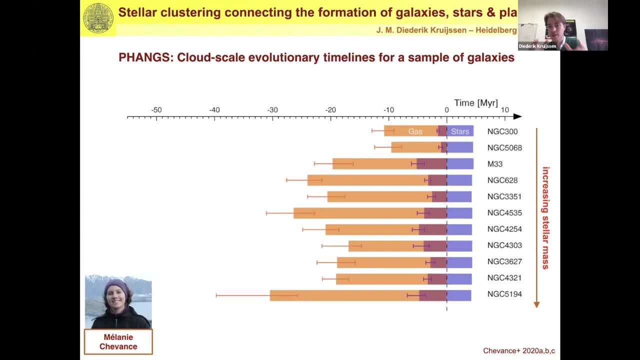 this evolutionary timeline of molecular cloud evolution, star formation and stellar feedback as a function of the environment in the local galaxy population. so it's no longer a problem that we're just a matter of time scale. so it's not an uncertainty of, for example, if we live for for, say, 100 years. 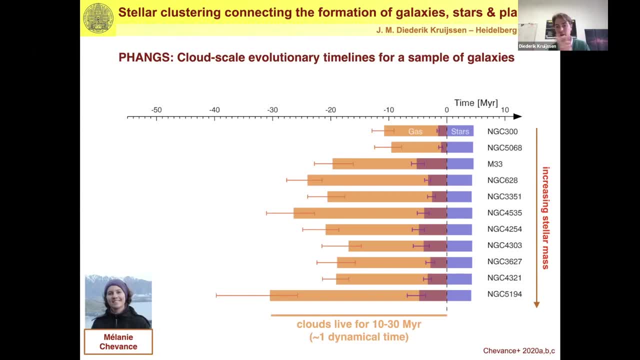 no, we can actually start measuring those timescales statistically, and what we see here is that clouds live for about 10 to 30 mega years. this is not an uncertainty range. you see that the error bars on each measurement are actually considerably smaller. now, this is physical variation between 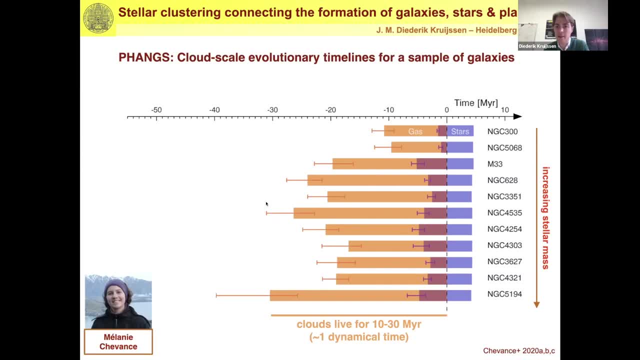 10 and 30 mega years, and this is about one dynamical time of the molecular clouds. something coming up in the chat? Oh yeah, that's right. Jayon is coming to speak in a couple of weeks, That's right. So the clouds have short lifetimes. 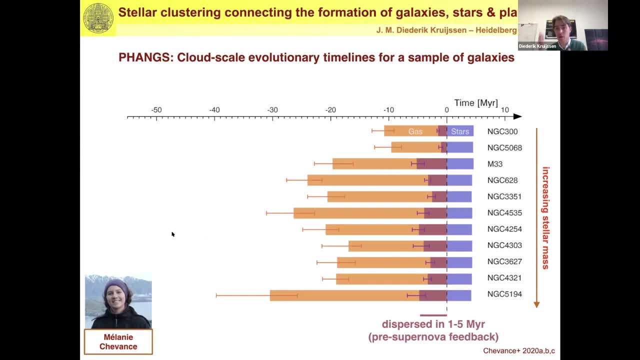 of about one dynamical time And for all of them we pretty much get the same result. as for NGC 300 is they're dispersed very quickly in about one to five mega years, which mostly is pre supernova feedback, especially if you account for a stochastic sampling. 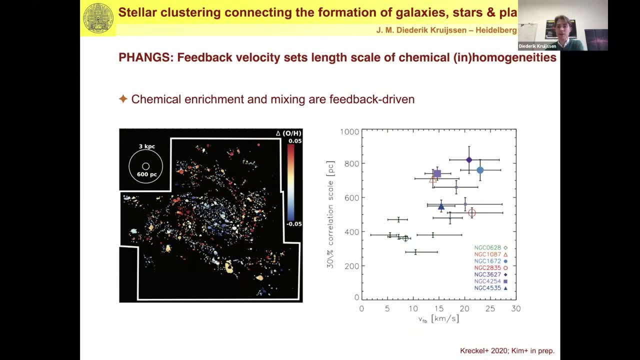 of the initial mass function. Now, interestingly, if we now compliment this with some of the MUSE data we've gathered with FAMS, you can look at how the feedback might impact the chemical enrichment of galaxies, And that is shown here on the left. 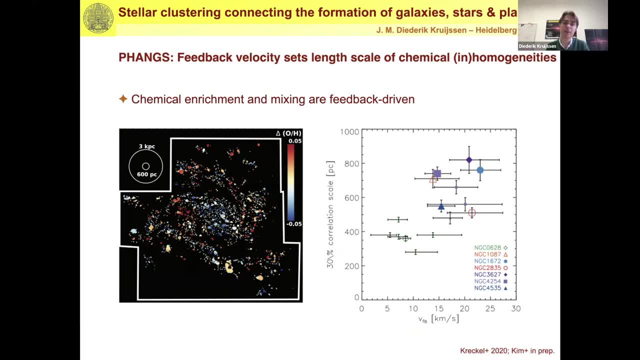 So on the left, we're showing here what is the metallicity differential locally relative to the large scale metallicity gradient within this galaxy, And this is in the ionized medium. So this is done with ionized line tracers And what you see is you see a lot of granularity. 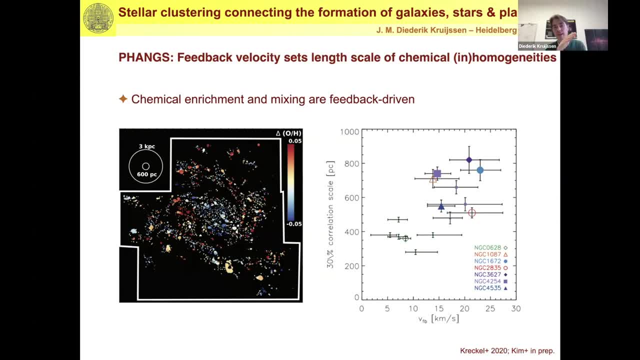 There is a range of different colors And what you can do here is you can calculate what the typical correlation scale is of those chemical inhomogeneity. So what is the scale on which the ionized interstellar medium is found to be inhomogeneous? 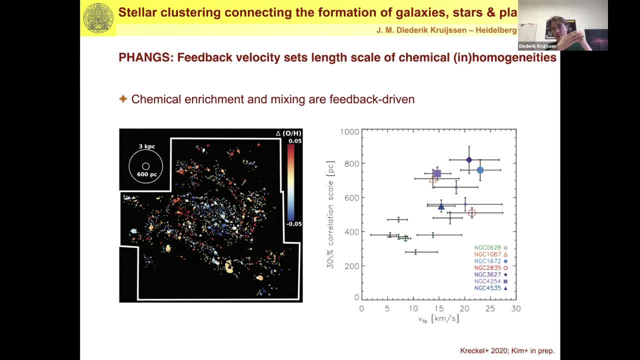 And what we did here is we correlated that with the velocity at which the feedback front is destroying its parent molecular cloud And that velocity you basically get from using the timescale that I showed before And the size of the molecular cloud. That gives you a first order estimate. 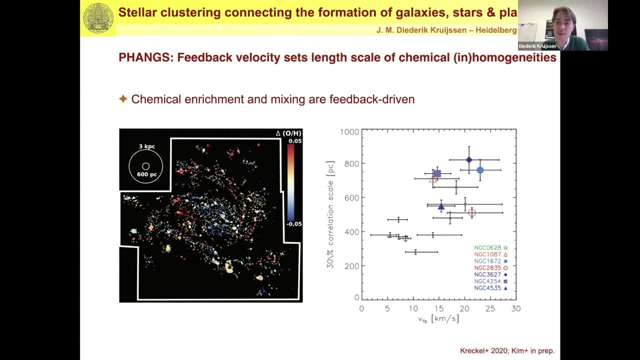 of what the velocity is of the feedback front, And it turns out that these are very nicely positively correlated, And what that suggests is that actually you have higher feedback velocities, Your chemical inhomogeneities are able to extend over a larger spatial scale- than when you have low feedback for a lot of these. 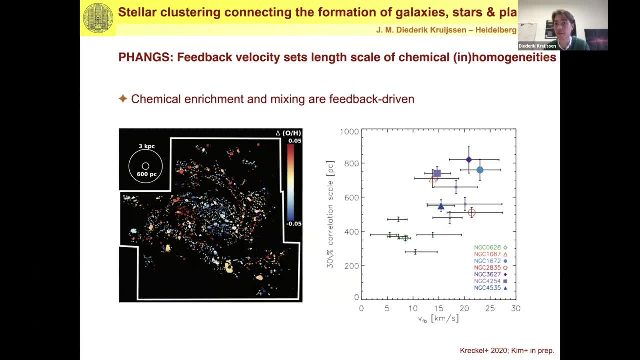 And that suggests that the chemical enrichment and mixing within galaxies are actually feedback driven. They don't come from large scale instabilities or super sub But again, feedback is actually not just driving the lifecycle of the interstellar medium but also its enrichment. 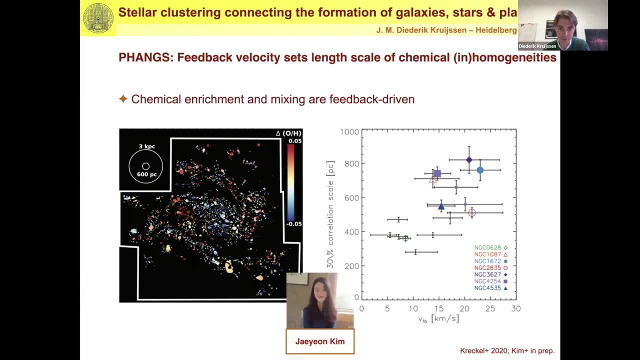 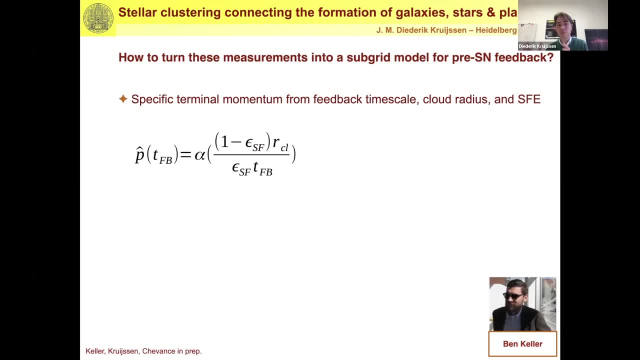 As I said, this is actually a work that you see here on the right, So this is exciting. We have a way of actually trying to solve this, Of solving the problem that we have in numerical simulations of how to model stellar feedback. And, in order to do this, what we need to do: 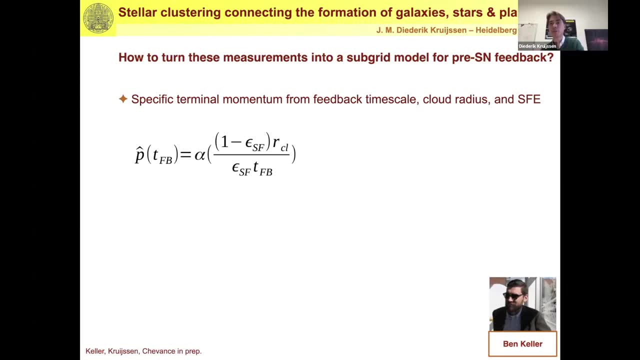 is. we need to take those measurements and turn them into a sub-grid model for early pre-supernova feedback. So we've been working with Ben Keller in trying to do this, and you can do this very simply. If you assume a self-similar feedback model, you can express the terminal. 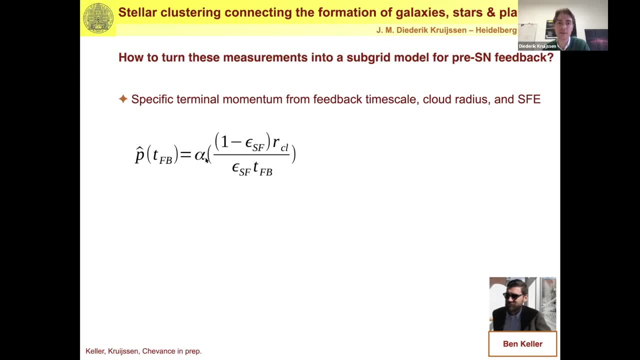 momentum of your feedback bubble, which is the p here on the left, as a function of the time scale, the cloud radius and the integrated star formation efficiency that the cloud achieves. And all of these are quantities that we can now measure. Now, if you calculate this number, 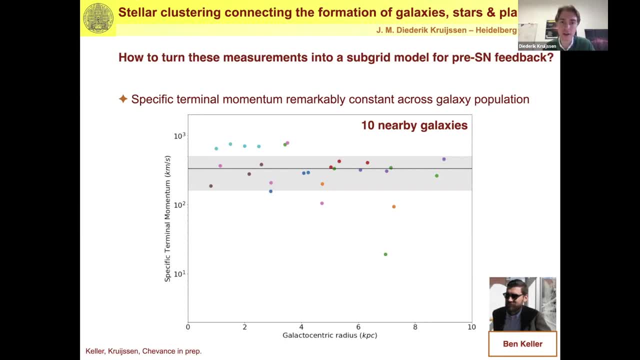 across these 10 nearby galaxies that I just showed for different bins in galactic centric radius. so that's why there are more than 10 data points. you see that this number, this specific terminal momentum, is actually remarkably constant across the galaxy population. 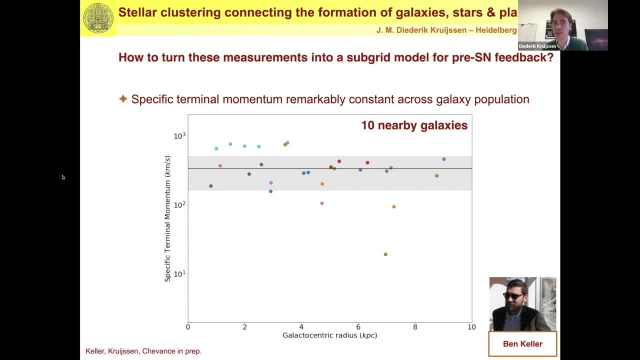 So it might be possible to actually just use a single number at least to simulate nearby universe, local universe, galaxies, to model their early feedback. So individual points on this plot are of what scale? It's not a point per galaxy, but it doesn't look like it. 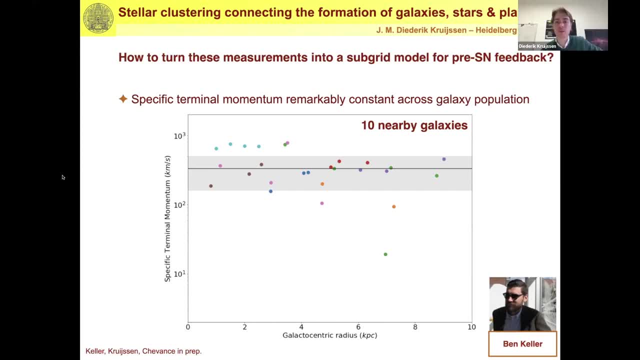 It doesn't look like it's a point per cloud. No, that's right. So, because it's a statistical methodology that we use, we need to have of the order of 50 clouds in H2 regions per sort of spatial chunk for bin. 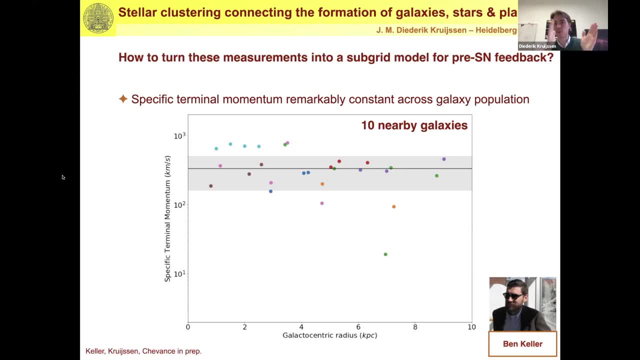 So we use radial rings that are optimized in width to ensure a sufficiently large number statistically, which then leads to of the order two kiloparsec. width of those radial rings, one or two kiloparsec. And what is interesting here? 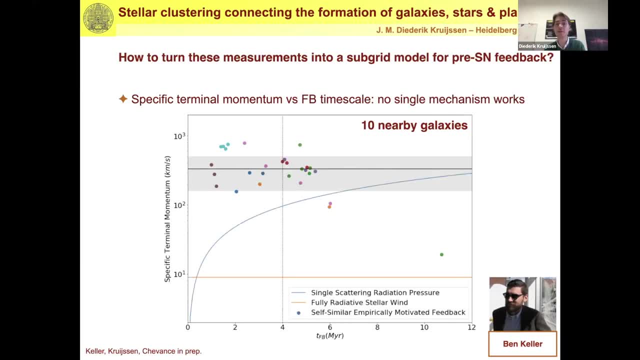 If you were to compare this to what you would predict for individual feedback mechanisms. so here shown now, as a function of the feedback time scale, what is the specific terminal momentum that you would get. it turns out there is no single feedback mechanism that you can use to. 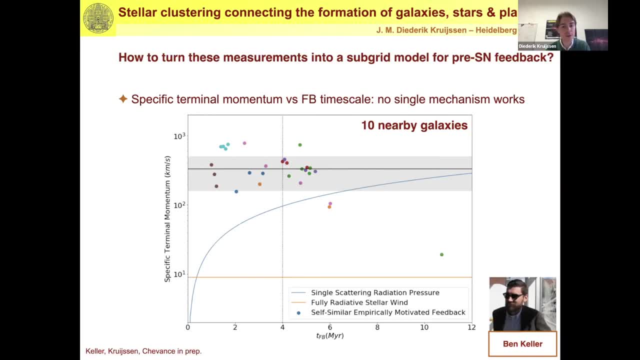 predict the observation. So if we just use radiation pressure, we would expect the terminal momentum to just increase with the feedback time scale. If we were to use a fully radiative stellar wind, we would expect it to be constant but much lower. And even if we were to 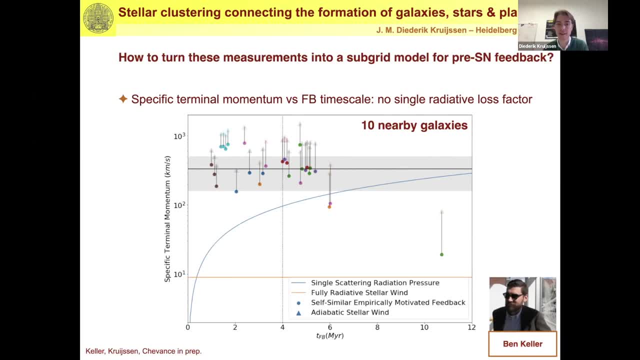 correct our observations for basically the radiative losses you would get in an adiabatic stellar wind, it turns out there is no way we can correct the data points to somehow be consistent with the stellar wind. So the only way of solving this non-linear interplay between all of those 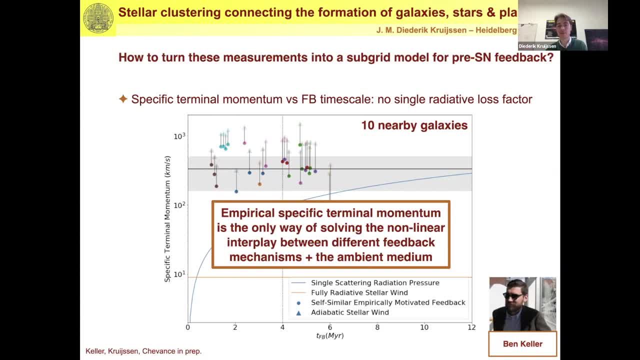 different feedback mechanisms and the ambient medium that seems to be taking place in nearby galaxies. the only way of solving this is by using this empirical, measured specific terminal momentum. But we can do that now, right, So we can take this. so this is the terminal momentum. this is what you get at the end. 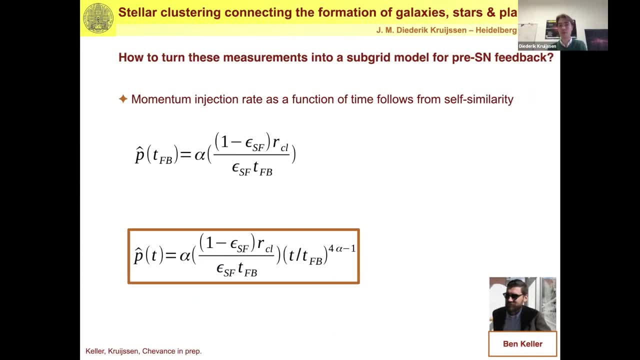 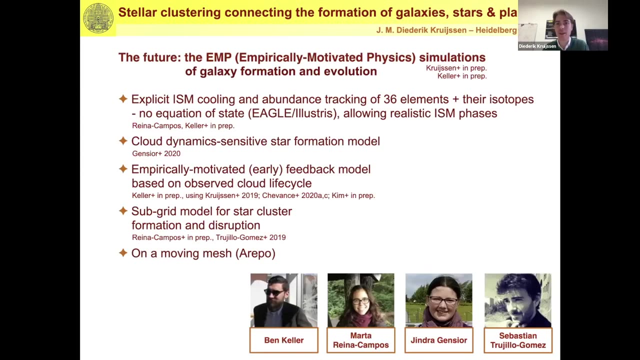 but if you assume self-similarity, you can basically write this down as a momentum injection rate. So, for every time step, okay, what is the amount of momentum that I input in my surrounding medium? And that is what we're doing now in the EMP simulations. EMP stands for empirically. 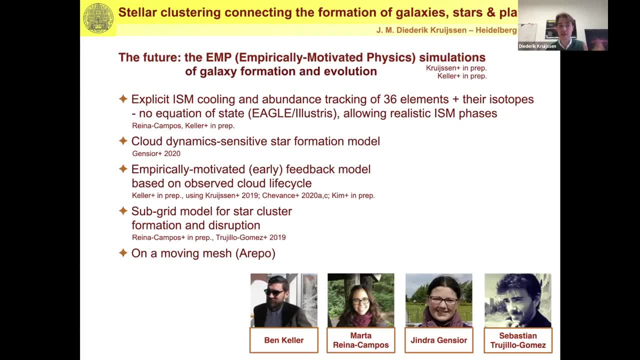 motivated physics And in those simulations they're performed using a repo. we're using combining a bunch of different data sets. So we have explicit ISM cooling a cold interstellar medium. We track the abundances of 36 chemical elements and their isotopes. We have a star formation model that's sensitive to. 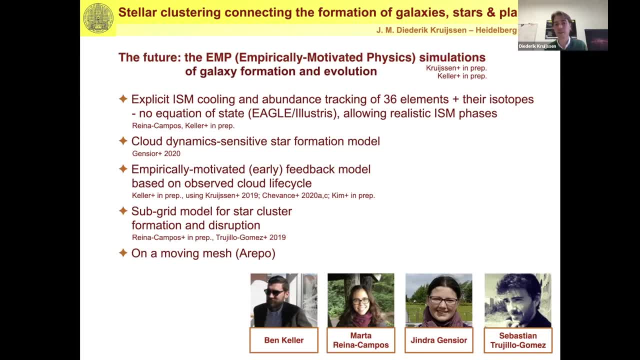 cloud dynamics And, most importantly, we have this empirically motivated early feedback model that I just showed. So it's basically we're putting in the right answer of the observed cloud life cycle and then ask: do we get out reasonable galaxies? And in addition, we have 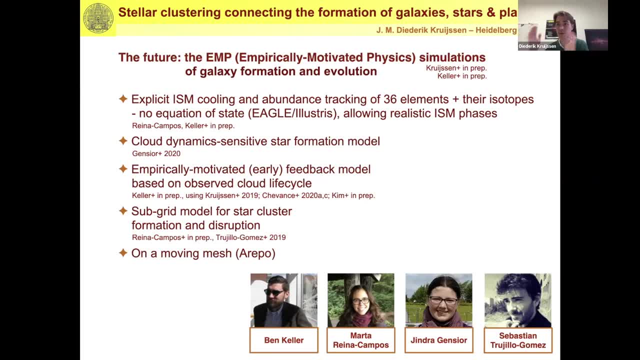 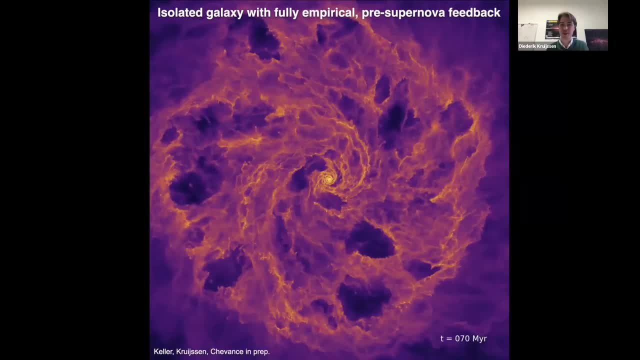 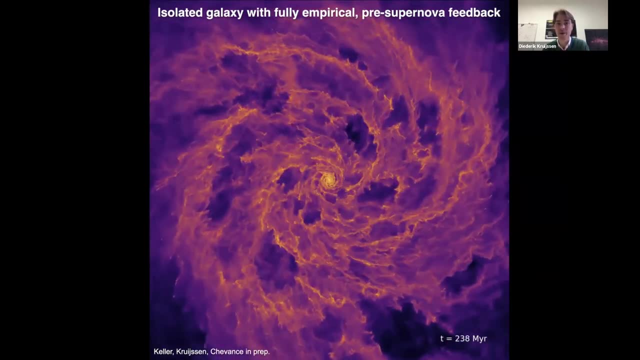 a sub grid model for star cluster formation and disruption, which I will touch on next in this talk, And I hope the movie works on Zoom, because that's always a big question if it is not stuttering. but this is a galaxy simulation, an isolated galaxy, where we have this fully empirical. 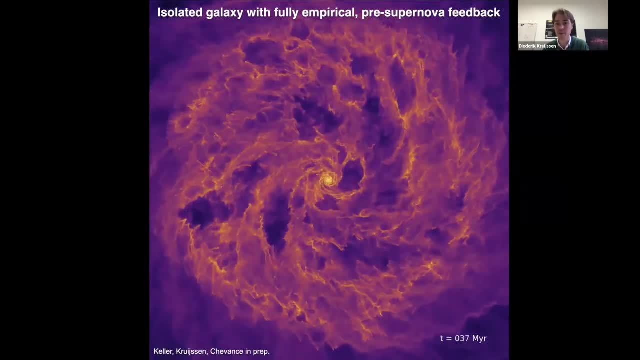 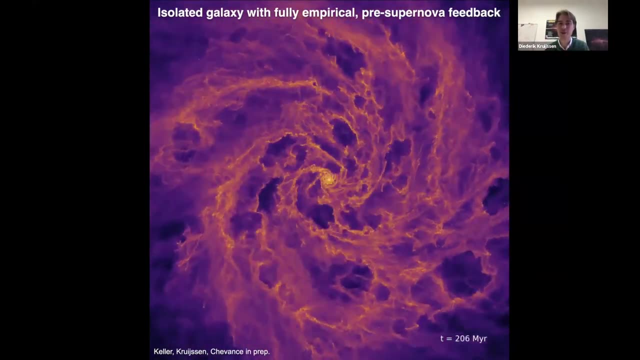 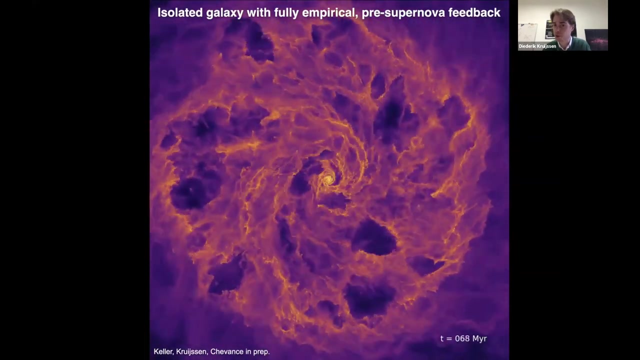 pre-supernova feedback running. So basically all of the structure you see here is shaped by that. Now I don't have many quantitative results yet because this is hot off the press, But one thing we've noticed already looking at this simulation is that the overall star formation 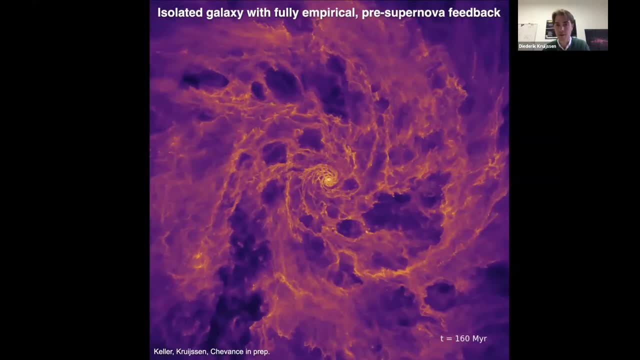 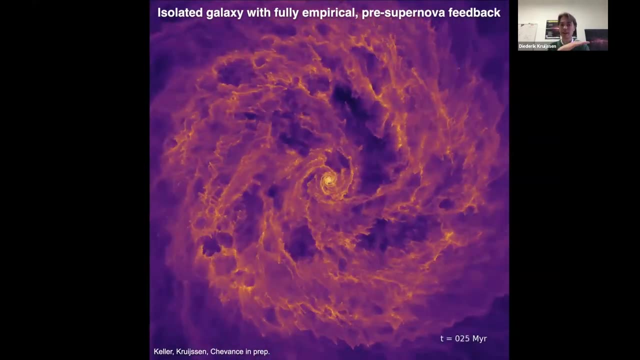 is very strong and it's also very stable. So very stable, very stable, And it's not going to change much. But the outflow history from this galaxy is radically different than when you're using, say, supernova feedback, as is typical in cosmological simulations. We 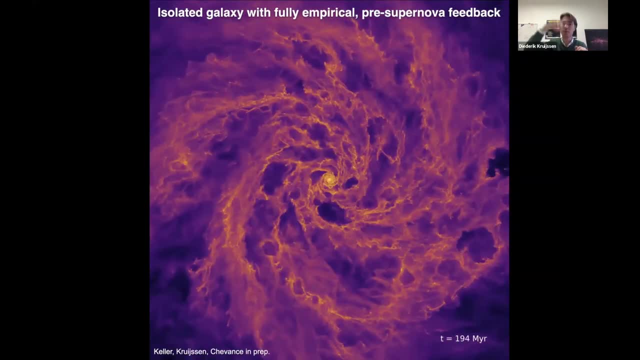 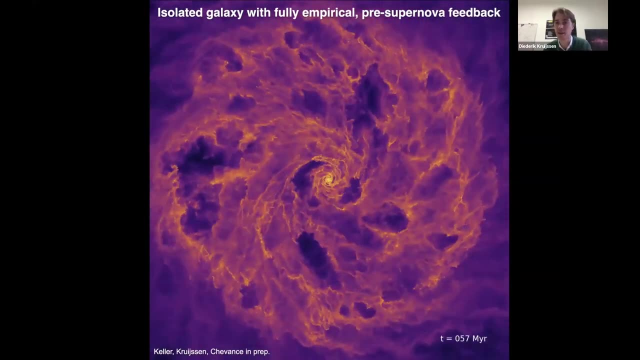 basically get a much smoother and more sort of systematically sustained outflow. that's much lower than the bursty, spiky outflows that you would get if you only had supernova feedback. So that's a really very concrete, interesting result that we see immediately looking at this simulation. 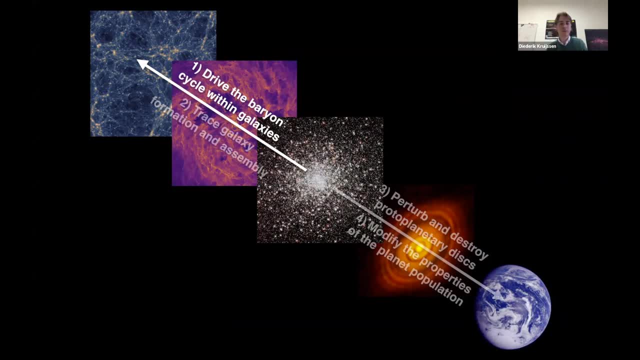 can sort of deconstruct galaxies into individual building blocks that drive the baryon cycle within galaxies and that that clustered nature of the stars, as they are born and and their lifetimes, is really important in determining the structure of galaxies and therefore how they end up forming and evolving over cosmic history. now, as i mentioned some of the structures that 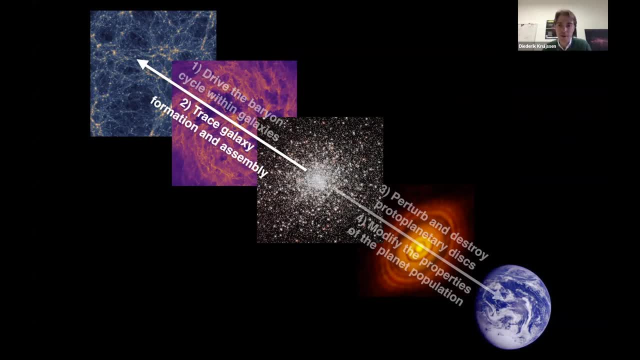 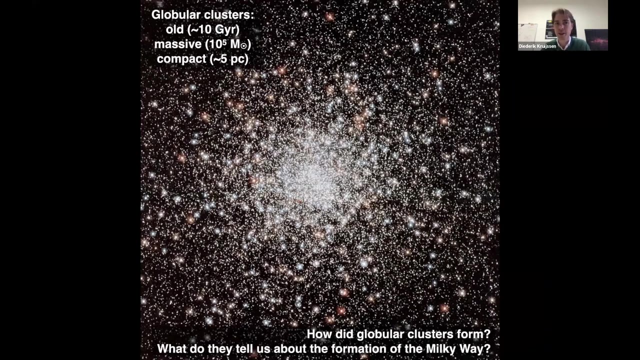 form in these star formation events manage to survive for nearly a hubble time, and those structures are globular clusters and in recent years we've learned to use these to actually try and trace and reconstruct galaxy formation and assembly. now globular clusters are pretty unique objects because they're old- they're as old as the oldest galaxies- but they don't contain dark matter. 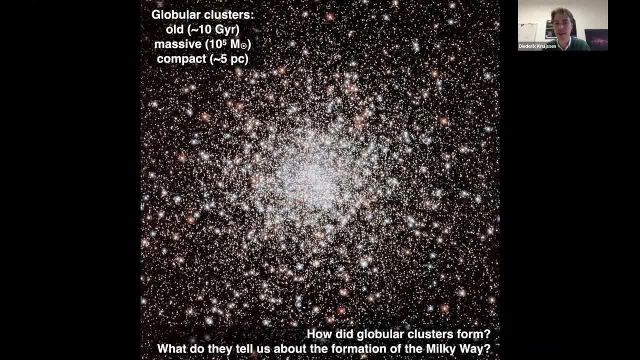 they're massive- of the order 10 to the 5 solar masses- and they're remarkably compact. they're probably the most compact stellar systems that we know of now. the key questions that we've been trying to focus on here is: first is: how did globular clusters form? 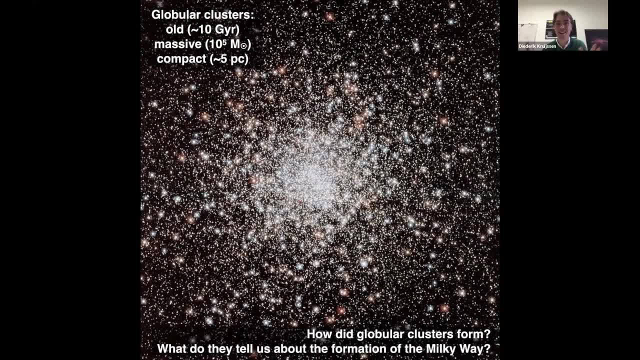 because it's very hard to witness their formation directly. uh, at that redshift of three at the current resolution right, is something that maybe, with james webb and 30 meters class telescopes, will be possible, and it's something we're actively working towards now. but the most important question, 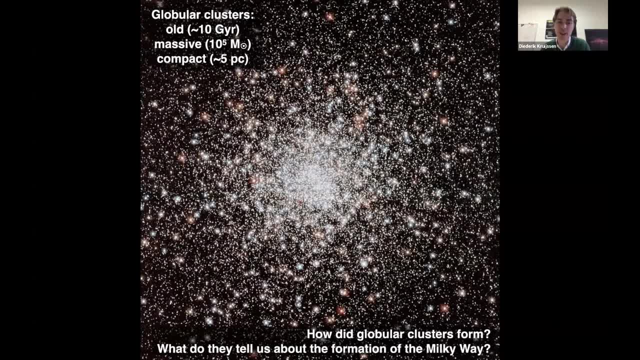 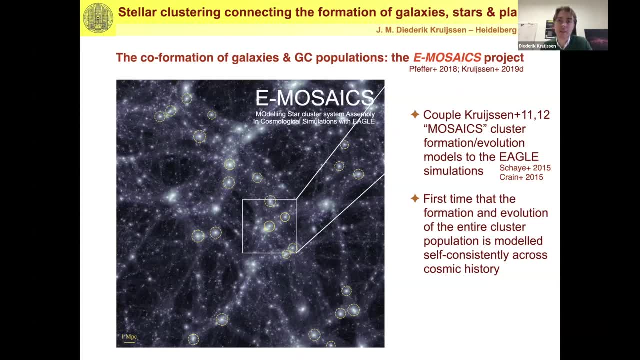 is that, once you've got a reasonable working model for globular cluster formation, is what do they tell us about the formation and assembly history of the milky way? and this is what we've been trying to address with the e-mosaics project. so e-mosaics is a project where we basically at first took the 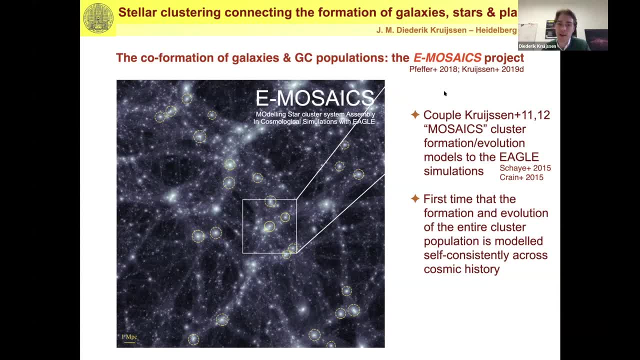 large eagle cosmological volume and did a re-simulation of a volume limited sample of milky way mass galaxies, where we couple the eagle galaxy formation model to the mosaics cluster formation evolution model that basically models the formation and dynamical disruption of stellar clusters depending on the local conditions within the galaxies that we see in the galaxy. 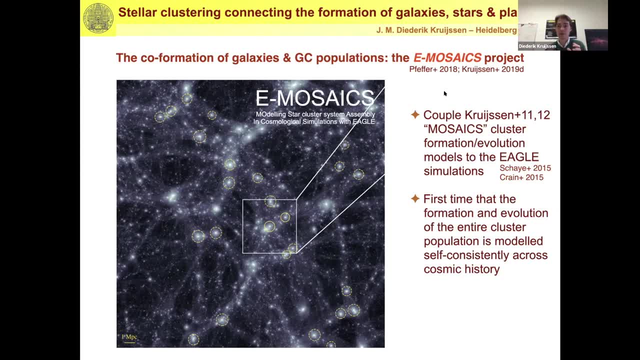 and that's what we're trying to simulate, and that's important because it allows us to model self-consistently, basically how the clusters evolve within those galaxies across cosmic history and basically make a comprehensive model of how the globular cluster population might have arisen. and the working hypothesis that we used here is basically: 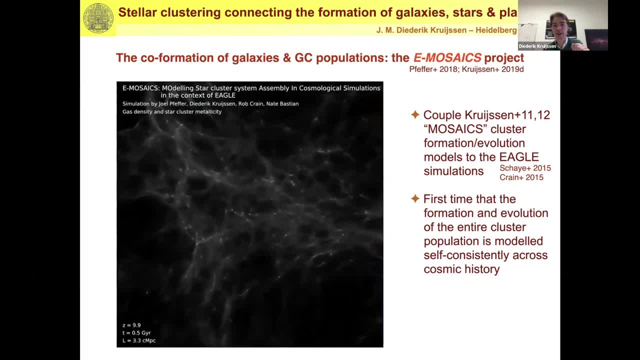 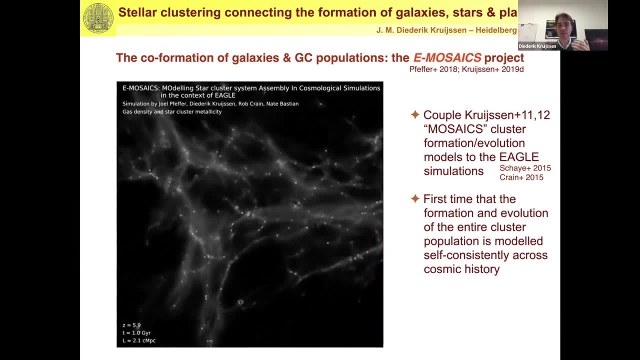 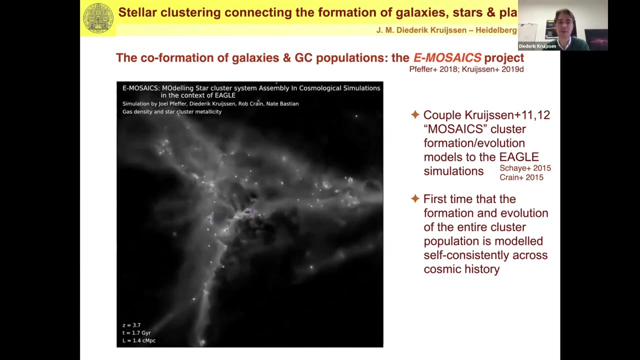 could we try to reproduce the young cluster population that we see in nearby galaxies and the old globular cluster population that formed at high redshift with the same model, so not distinguishing between them, but basically just using the same model to see if globular clusters are the relics of normal star formation and high richard? so this is a simulation. 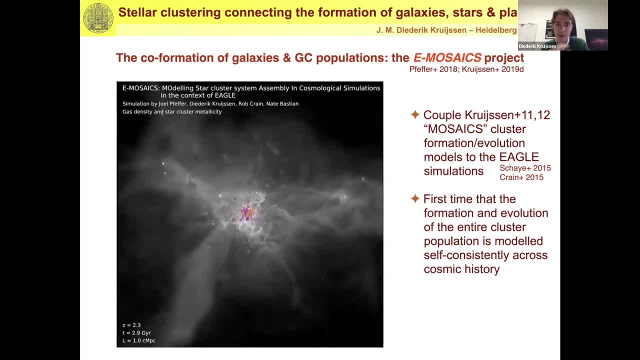 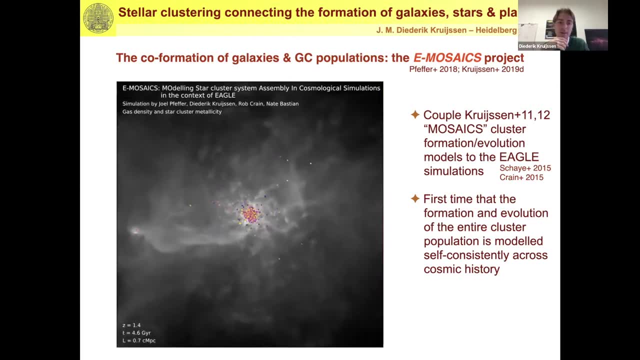 it's one of the emosaic simulations. uh, what you see here in gray is the gas, and the colored dots that you see here are the stellar clusters that are forming as the simulation is going, and, uh, they're color-coded here by the metallicities actually, so the bluish ones are the most metal. 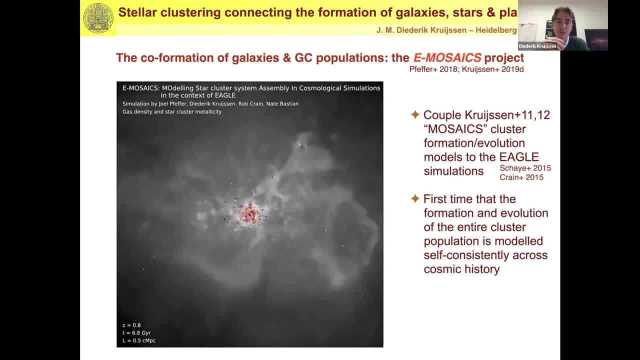 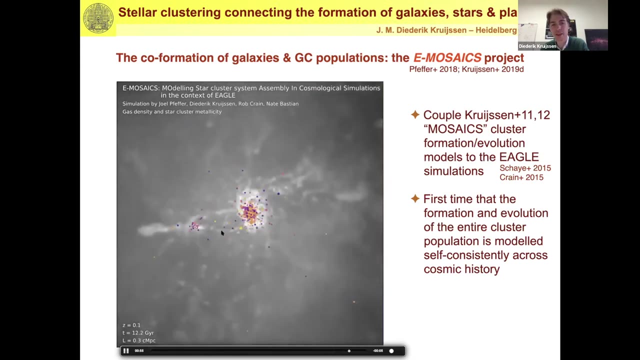 poor. and then, as the colors get more, uh, vibrant, metallicity goes up and what you see here is a galaxy. uh, merging is bringing in its own globular cluster population. so we see we have both in-situ globular clusters that formed in the main progenitor, but also ex-situ ones that are being accreted here and are populating the 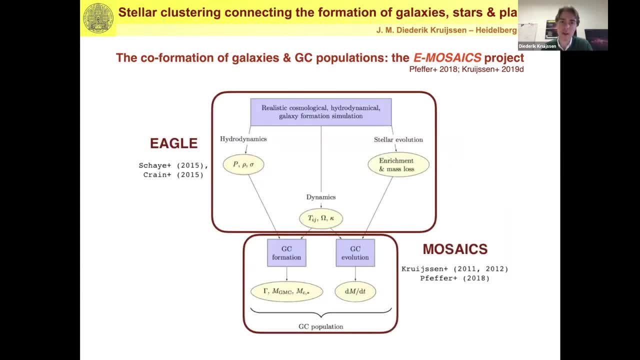 halo of the central galaxy. so this is a short summary of what we do. so we use basically the hydrodynamics, the solar evolution and the dynamics from from eagle and then mosaics, and we also use the hydrodynamics, so the local gas conditions and the local dynamics, to motivate. 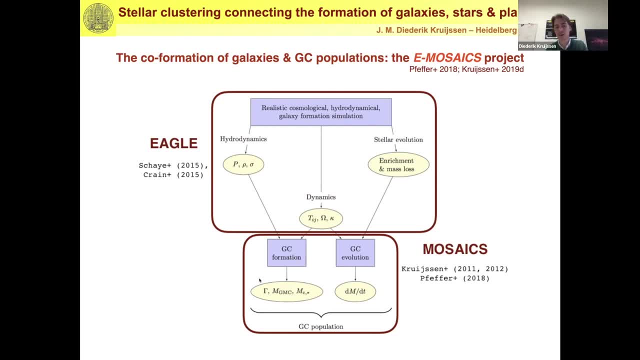 the globular cluster, the stellar cluster formation. so we have models describing what the fraction is for star formation occurring in in bounds that are clusters. we have a model for the initial cluster mass function, the maximum cluster mass, and then we also use the dynamics and the stellar evolution. 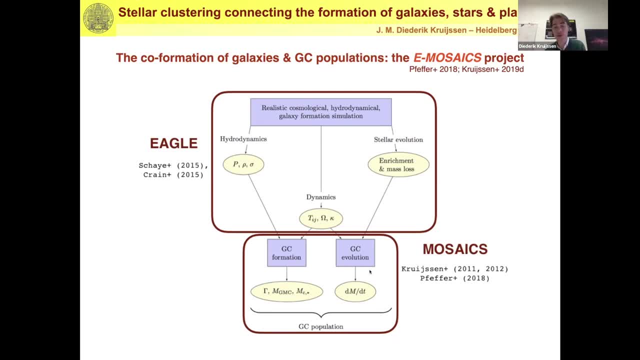 to motivate the stellar cluster evolution. so how much mass the clusters lose due to stellar evolution and how much mass the clusters lose due to body relaxation within the cluster and tidal shocks from passing substructure as they're orbiting their host galaxy? can i ask so in your lower left ellipse? 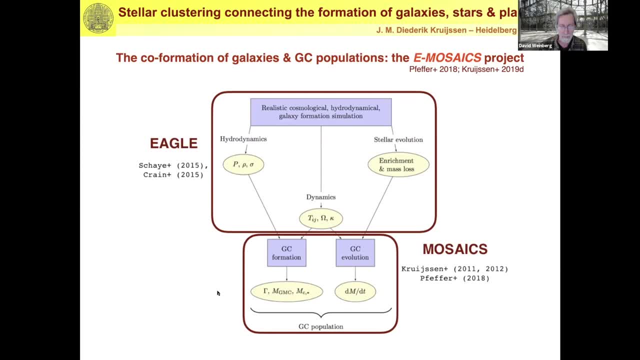 there, gamma, mg, mc, mc, star, though those are model parameters, they're not things you're trying to compute from. no, so we cannot resolve in order to resolve the cluster formation efficiency. uh, you would need to technically resolve the imf in order to resolve the cluster formation of the imf, which means a computational dynamic range. 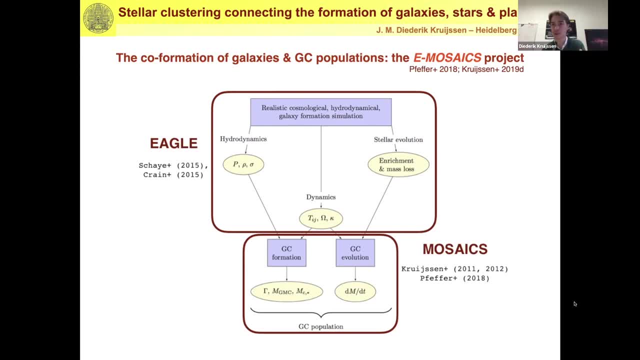 problem. that is presently not possible. so we have basically with an analytical subgrid model that says: okay, as a function of galaxy, local galaxy properties, this is what we would expect. we'll predict for the cluster, information efficiency and uh, these are models that have been like each. 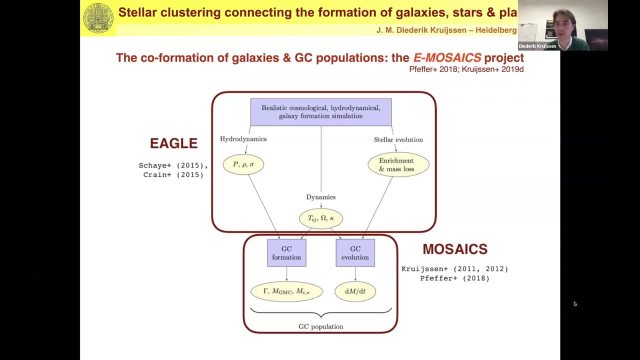 of these subgrade models themselves has been tested against observations in dozens of papers, so we have some confidence that these are reasonable starting points. it's basically what we know of cluster information in the local universe, and then the question is if we apply that to the evolving cosmic conditions. 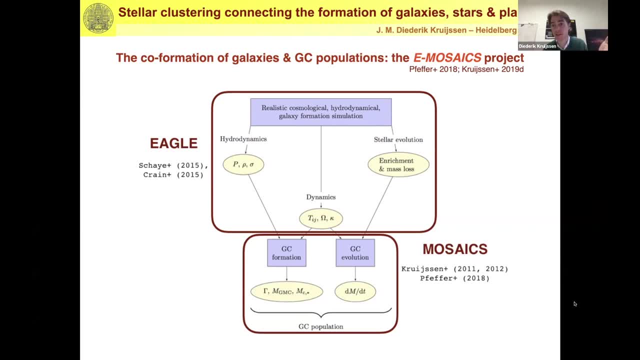 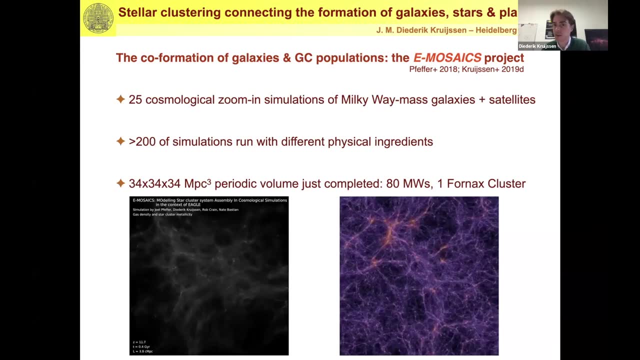 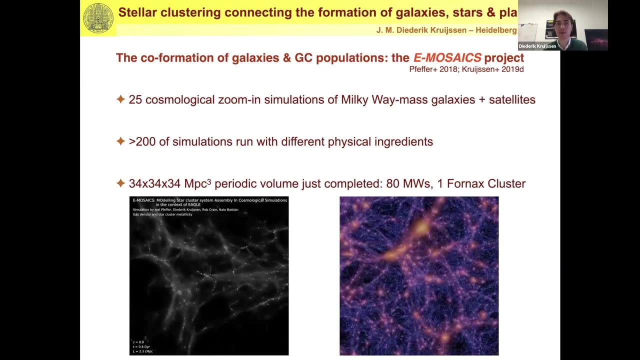 do we get out global clusters? okay, and that's that's the question. so, as i mentioned this, for at first we had 25 cosmological zoom in simulations with multi-way mass galaxies and their satellites. um, this is sort of the definitive set, but then, in addition, we ran hundreds of simulations varying those subgrids in order to determine. 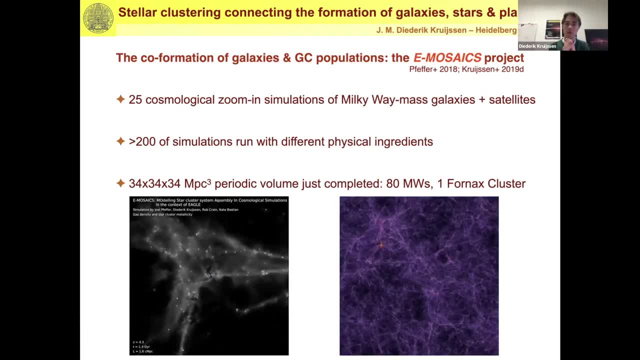 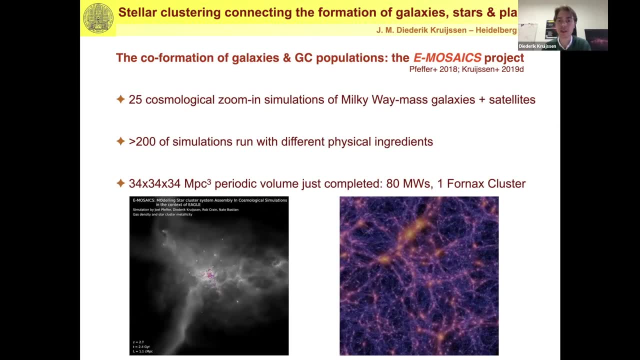 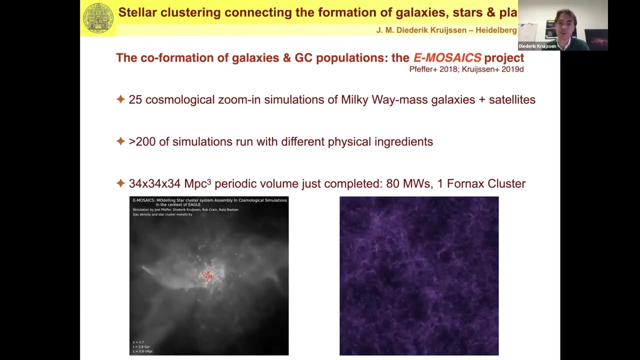 what those subgrade models were and that's what we could rely on. we had a number of subgrid models trying to see exactly what we could rely on, what had an impact on the on, on the cluster populations, what didn't, where the uncertainties are, and so on, to really convince ourselves of the elements. 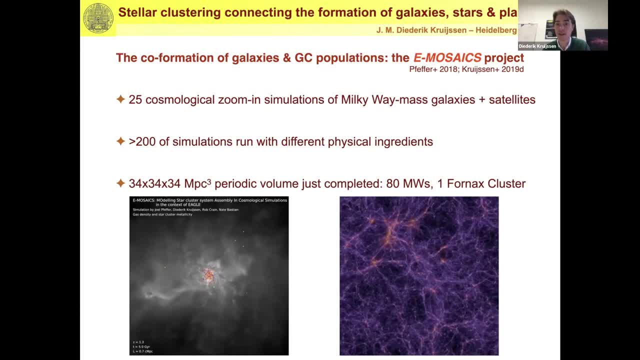 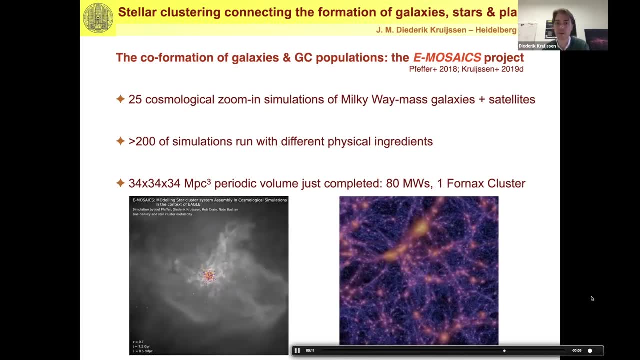 we could trust and elements we could not trust. and once we had completed those, we then in addition completed a 34 mega parsec volume, which you see here on the bottom right, which now has a very large population of multi-way mass galaxies and goes all the way up to a foreign. 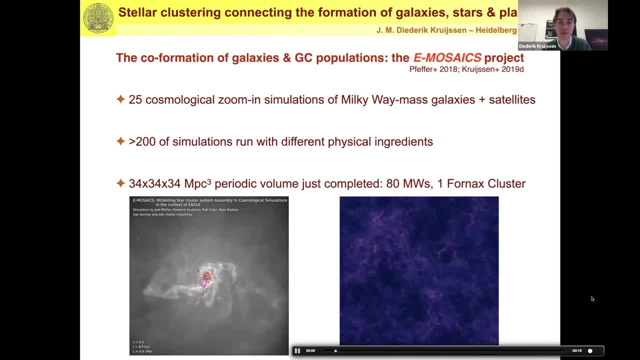 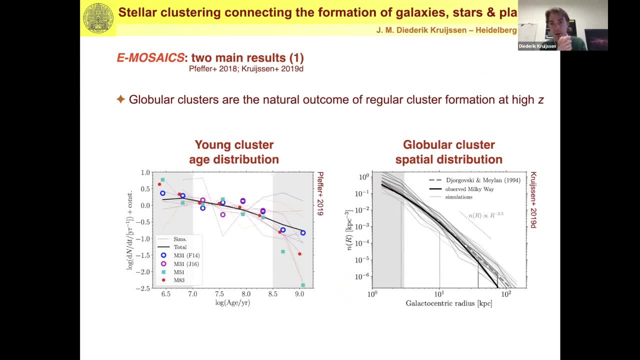 So we've not done a lot of science with that, but it's very exciting that we can now start working with that, And there were two main results coming out of the mosaics. First is- and I will only show one slide on this- 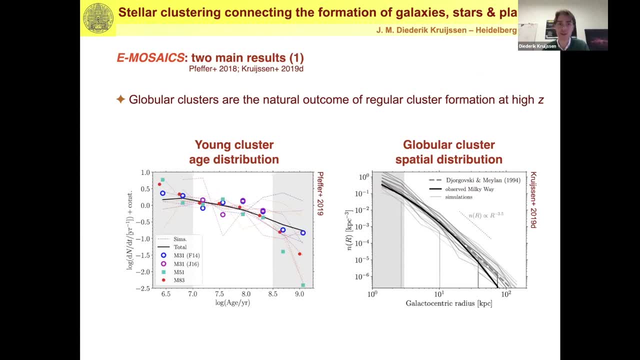 is that indeed we can reproduce both young cluster populations and globular clusters with the same star cluster model, And I'm showing two examples here. So on the left we see the age distribution of young clusters where the simulations have a median. here is the black dashed line. 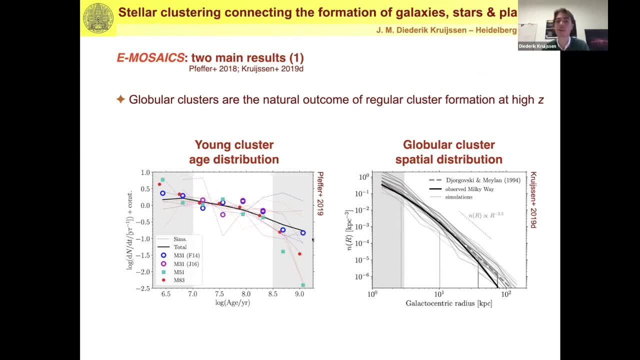 And then observations are the symbols: typical age distributions in nearby galaxies, And you see that we actually do a decent job in reproducing the rough slope that that age distribution has, which means that we have a reasonable treatment of cluster disruption. Now, in addition, what you see here on the right, 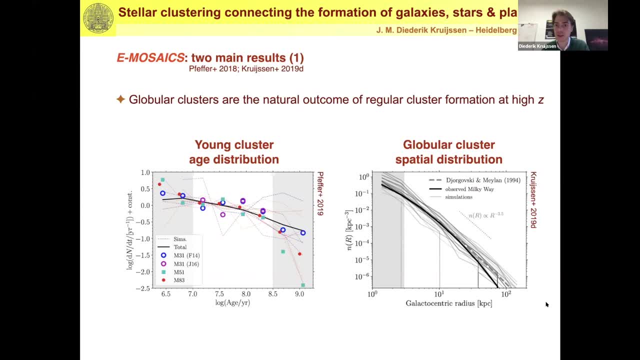 is one of the many observables that we compared to the globular cluster population. As we're in black, you see the observed spatial distribution of globular clusters around the Milky Way, And then, in light gray, you see the globular clusters around the Milky Way. 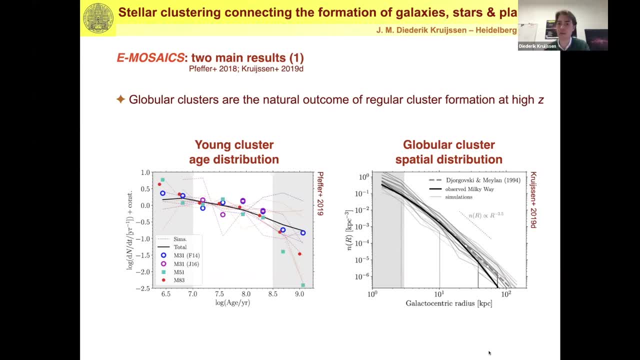 And you can see all of these simulated spatial profiles. for a 25 zoom in simulation again follow very similar spatial profiles. Now, as I mentioned, these are just two observables. We've done many, But I'd like to focus on the second question. 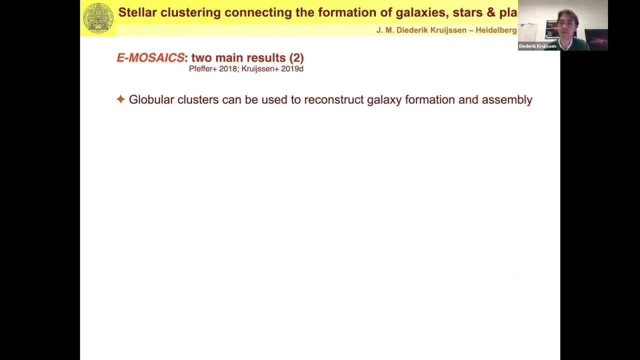 that I asked, which is how can we use globular clusters to reconstruct galaxy formation in assembly And historically in the Milky Way? this type of work is really focused strongly on the age metallicity, distribution of globular clusters. So here on the y-axis, we've got metallicity. 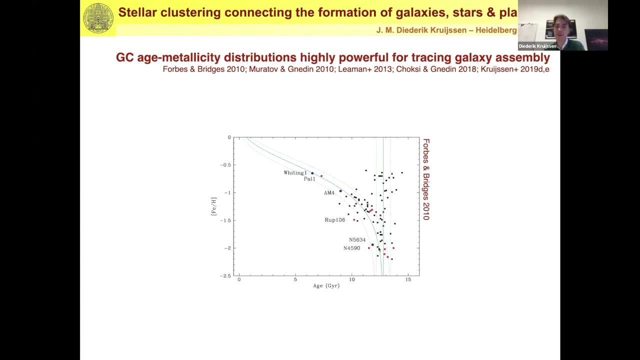 And we've got the age. And on the x-axis, we've got the age. You get this very characteristic sort of forked shape with a y-shape where you have a relatively vertical branch here and then a branch coming off. 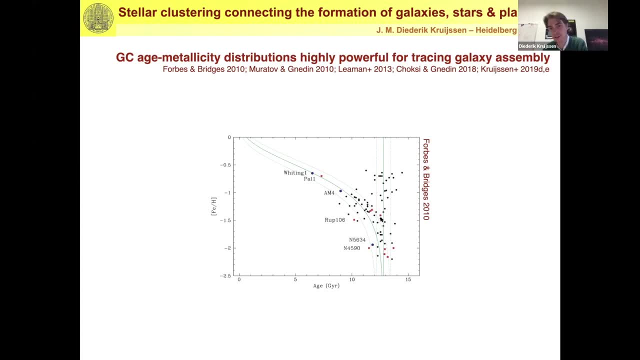 And for reasons that will become clear in about one slide. this is what I'd like to call the main branch And this is what I like to call the satellite branch, And in NEMA's eggs we can figure out very directly why that is. 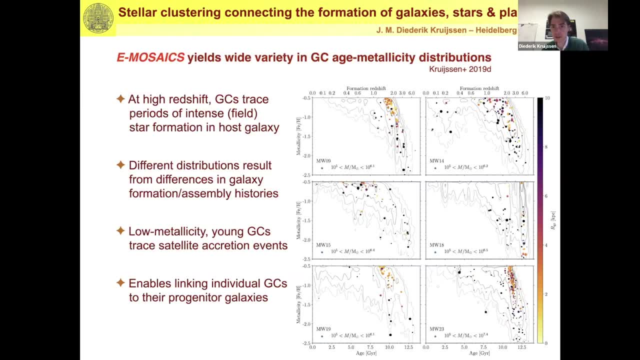 So here I'm showing six different age metallicity distributions for six different Milky Way mass galaxies of the globular clusters in NEMA's eggs. So the symbols here are the globular clusters color-coded by their galactic intergradiance. 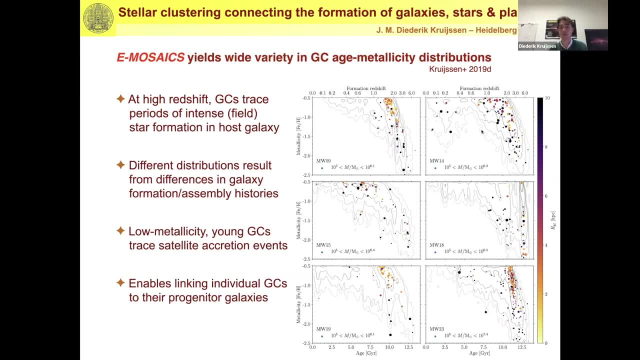 And the contours here are the field stars within the same galaxy. So it's basically the star formation history and the enrichment history of the host galaxy. And what we see here is that, by and large, the globular clusters trace periods of intense field star. 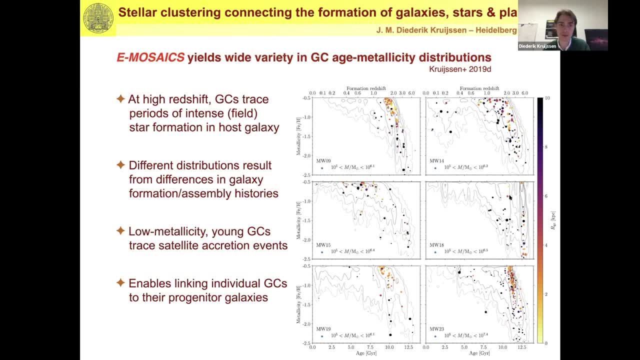 formation. Whenever there is a lot of contours, you tend to get globular clusters too, But of course all of those distributions have roughly the same trends as in metallicity goes up as these galaxies evolve. But in addition we actually see distinct differences. 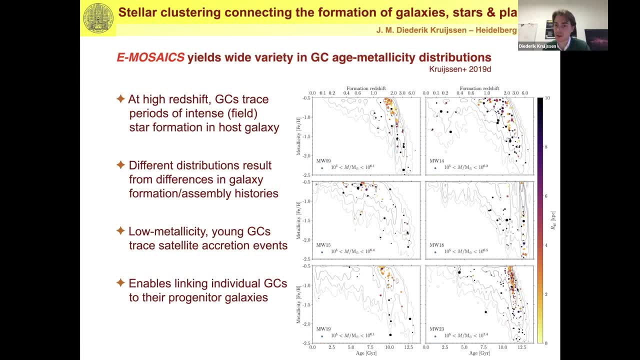 Some of them are very gradual, like this one, whereas other ones are quite steep, like here, And these differences actually result from differences in the galaxy formation and assembly histories And already what I indicated on the previous slide. if you get low metallicity, young globular clusters, 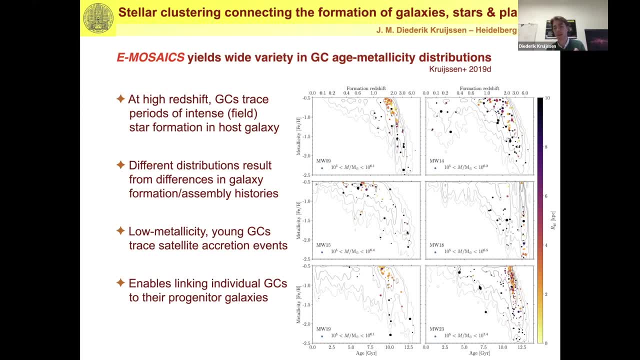 these formed in lower-mass galaxies because lower-mass galaxies chemically enrich more slowly. So these basically trace accretion events. You can be pretty confident that those globular clusters are ex situ and the ones that shoot up very quickly here. 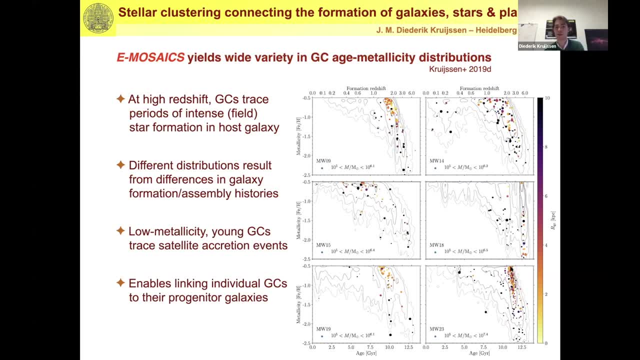 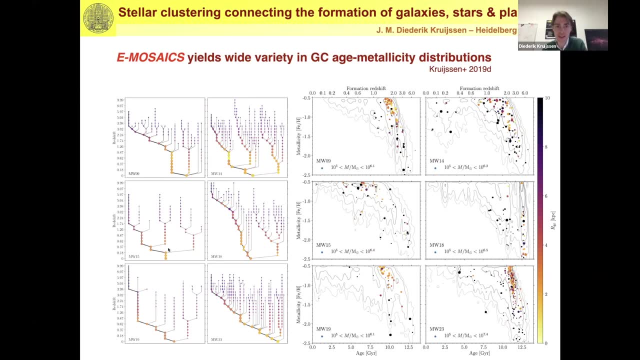 to high metallicities are in situ, And what that allows us to do is link individual globular clusters to their progenitor galaxies. Now here, just for comparison, here are the merger trees of the same galaxies And you can see very directly what I just mentioned. 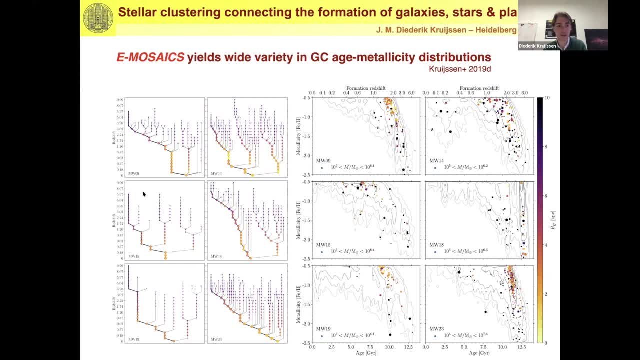 This gradual H-metallicity distribution has, in fact, a lot of interest And you can see that the H-metallicity distribution has a very quiescent merger history, whereas this very steep H-metallicity distribution has a very intense merger history with lots of mergers. 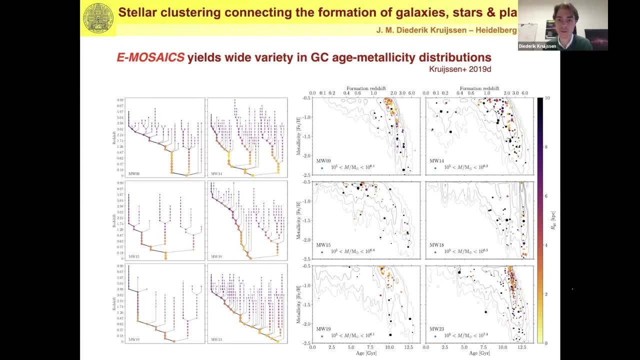 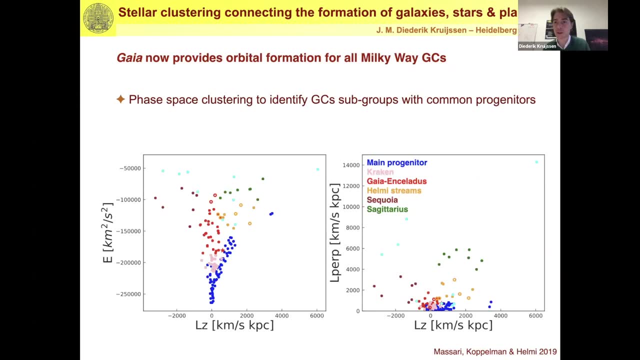 So you can really start to use this type of demographic to learn about how the parent galaxy formed. Now, with Gaia and the Milky Way, we don't just have ages and metallicities, We also have kinematics, And a lot of groups have actually started. 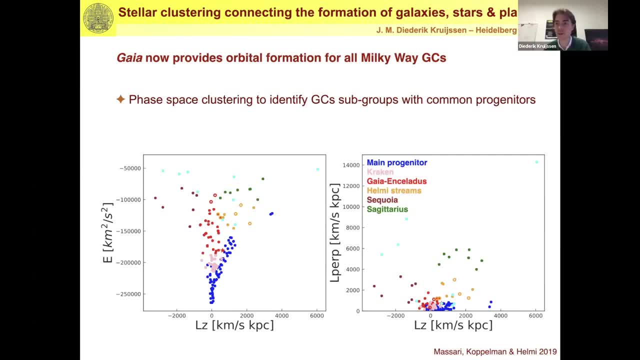 to group globular clusters in orbital space, And that's what Helmer was involved in two years ago And basically what Massari, Helmer and Amina did was to try and group these globular clusters such that they could be connected to individual merger events. 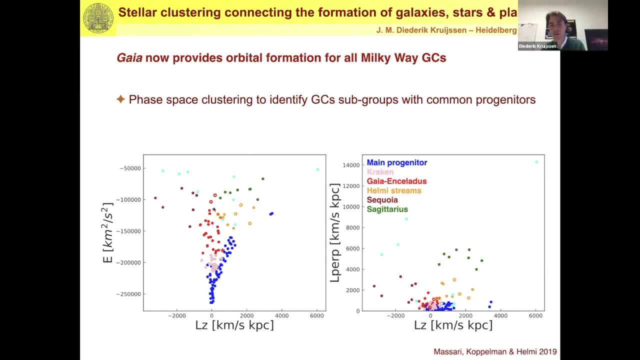 that the Milky Way experienced. Now what we've tried to do with e-mosaics is connect those groups of globular clusters to similar groups of globular clusters that we saw in the simulation. To that we've tried to do a lot of things. 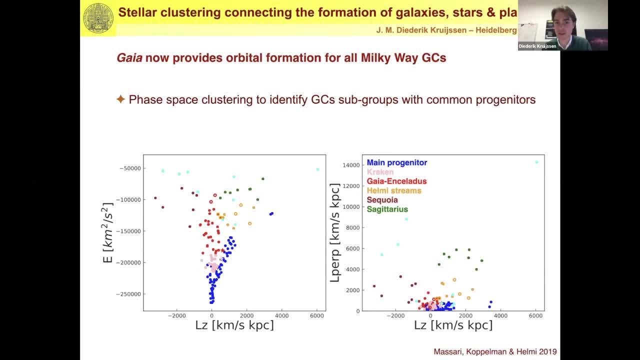 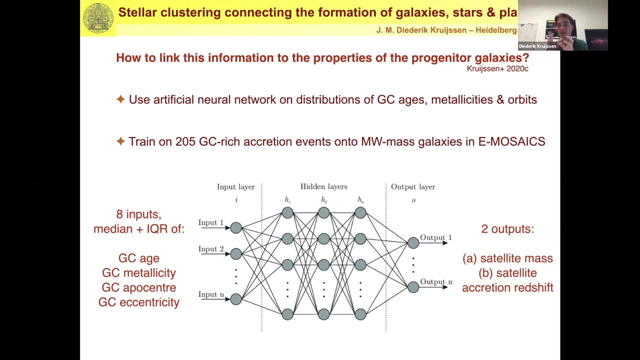 We've tried to find out what the properties of the progenitor galaxies were, And the way we did that is we used a neural network to link the globular cluster, ages, metallicities and orbits of these groups that are thought to have come from the same progenitor. 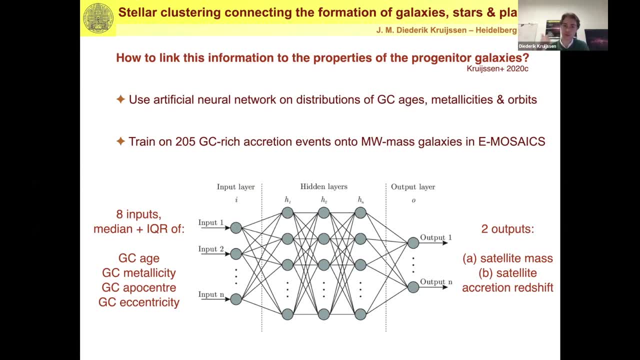 to the mass of the progenitor satellite galaxy and the redshift at which it merged with the central. So we basically took all globular cluster ridge accretion events from e-mosaics to train the network to connect globular cluster properties, cluster properties to these galaxy observables. 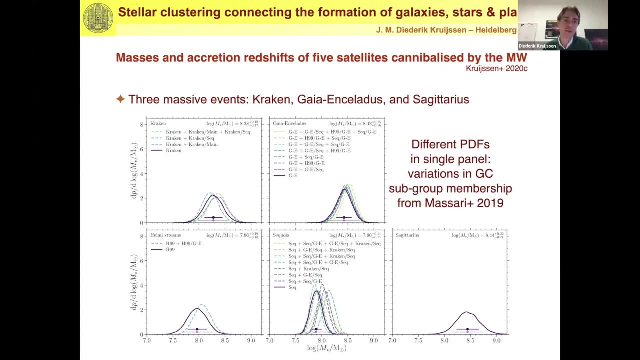 And by doing that and varying the hyper parameters of the neural network we would get probability distribution functions on exactly these quantities. So I'm showing here for five accretion events where Massari and collaborators were able to group those global clusters, for those five 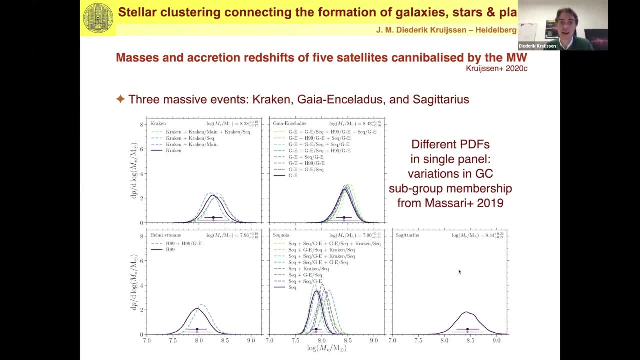 accretion events. We analyzed global clusters this way and measured that way or predicted, the masses of the galaxies that they came from, And we found that there were three massive accretion events. The first here is what we called Kraken, then Gaia Enceladus, which is 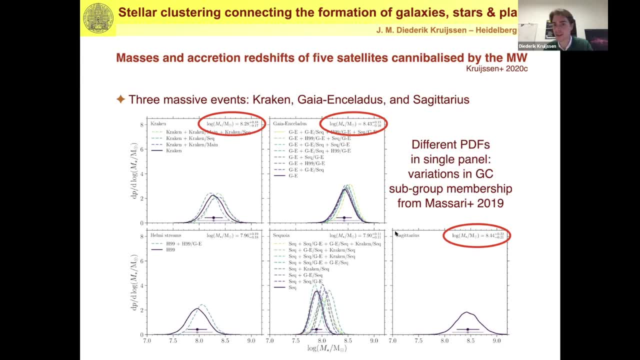 the famous one that, again, Helmer was involved in, and then Sagittarius, which is the one that is already known since 1994.. We found that all of these accretion events of masses, of several 10 to the 8 solar masses, but 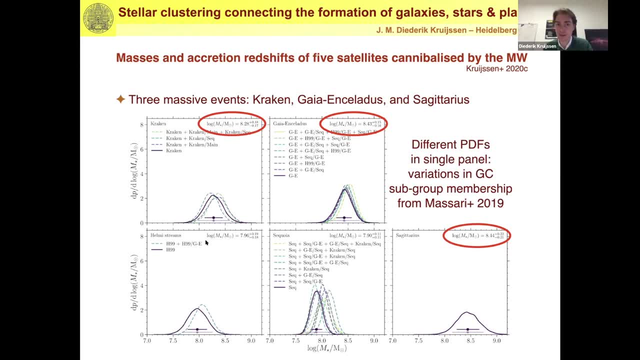 roughly similar and the two other accretion events that we look at here, so the progenitor of the Helmi stream, For instance Sequoia, were likely much less massive or considerably less massive, a factor of a few. But what is interesting is that those 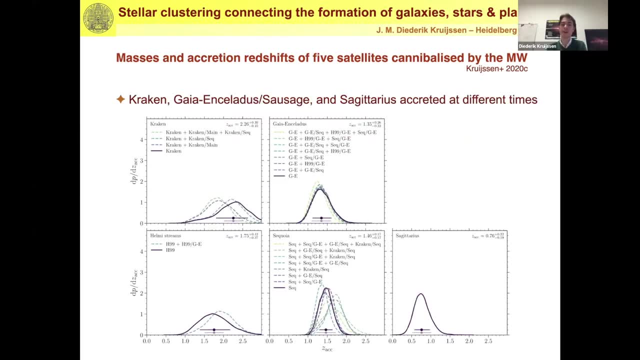 different galaxies actually merged with the Milky Way at very different accretion redshifts. So what we see here is that Kraken was an early merger, Gaia, Enceladus, an intermediate merger, and Sagittarius. of course, we still see the debris. 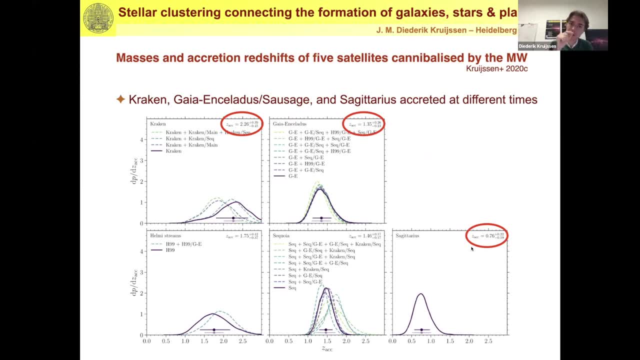 is a very recent merger And it turns out. if we look at the neural network, we can of course, figure out where that difference in redshifts comes from. It is basically It's a combination of the galaxy mass and the binding energy. 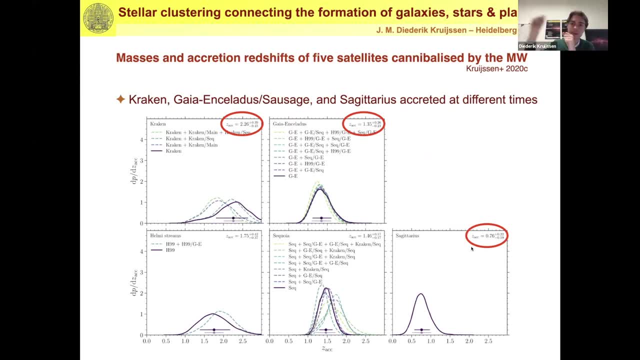 These two are related because, basically, if you, if you have similar mass galaxies and they have different binding energies, it means they must have accreted at the time that the Milky Way had a different mass And, in addition, we, of course, we have the age. 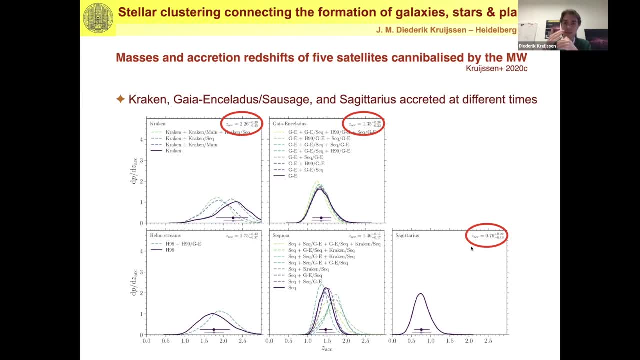 metallicity information, which tells us something about how quickly these satellites enriched and therefore how massive they were. And in combination you can- basically you can- solve the mass accretion, redshift, degeneracy Now, Despite the fact that they all have the same mass. 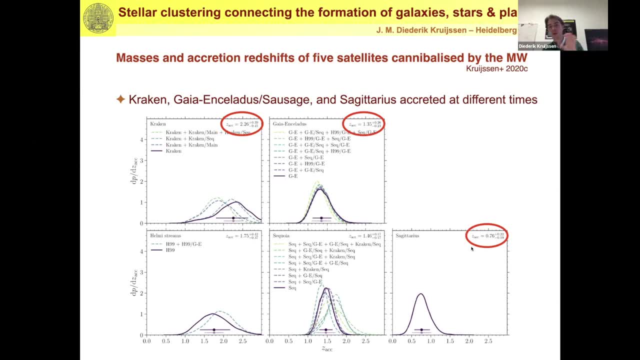 we see that they created a very different redshifts and that means that the Milky Way had very different masses during each of those mergers. And if we combine that information we find that we can calculate the merger mass ratio of each of those. 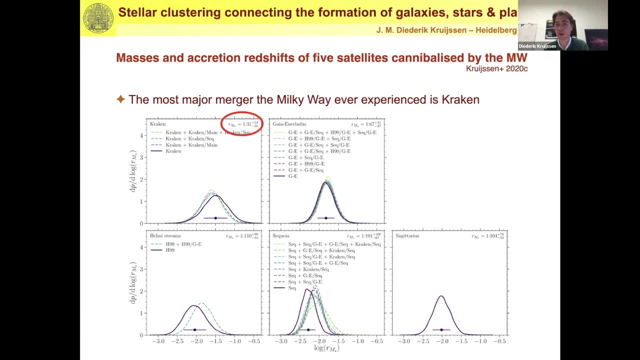 And we find that Kraken was basically the most major merger that the Milky Way experienced. It's still a minor merger, It's very small, only one to 30, but the most major And we also find this way that the Milky Way didn't. 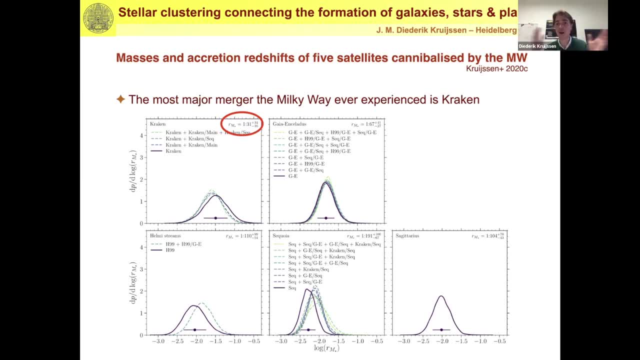 have any major mergers since Richard four, Which is a very long time to have such a quiescent life, But maybe that's why we exist. Maybe that's why we exist And that's what the second part of this talk touches. 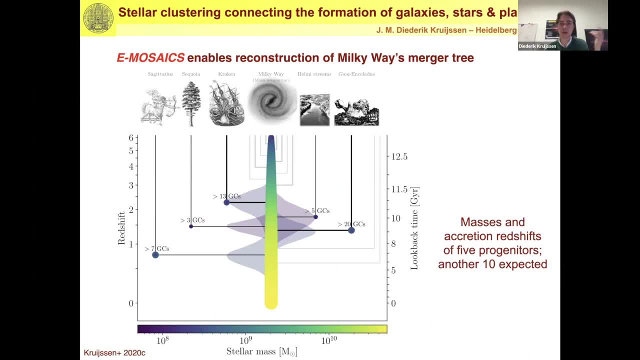 So, putting those results together, This is what a rough sketch of the Milky Way merger tree would look like. So we have those five galaxies that we can now characterize in some detail. Then, based on the number of global clusters that the Milky Way has, 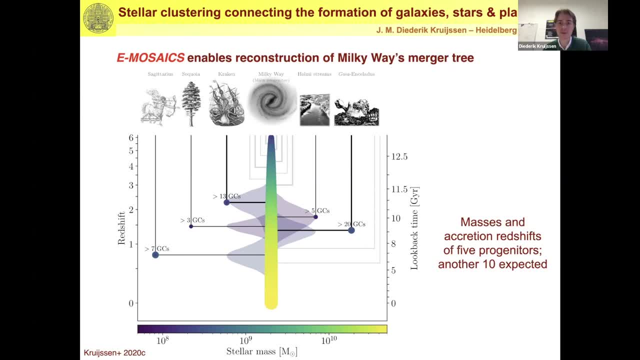 we expect another 10 mergers with masses more than 10. And that's what we're looking for, With masses more than 5 million: solar masses and stars, And, of course, that debris is not known yet, So we still need to find those. 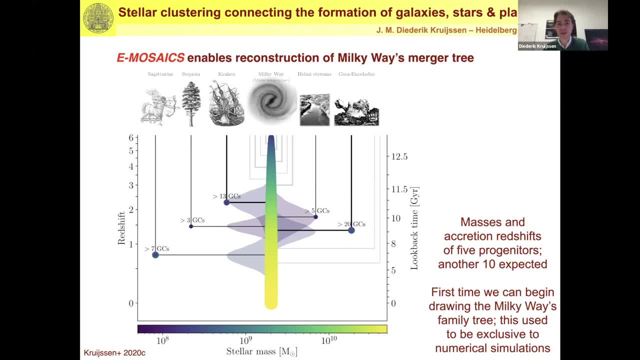 But it's the first time we can start drawing this merger tree And I think that's really exciting because, you know, for me as a simulator by nature, and nurture kind of this is something I used to do for simulations, Doing it for the Milky Way. I think it's a lot of fun. 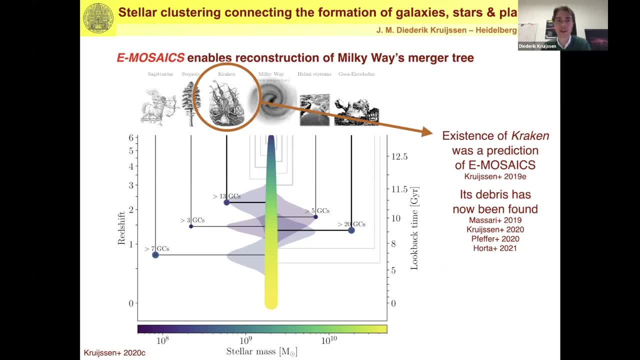 One of the really interesting results coming out of E-Mosaics is that we actually predicted the existence of Kraken based on the globular clusters, And Massari then found that group of globular clusters in the galactic halo And Horta and collaborators now have found actually. 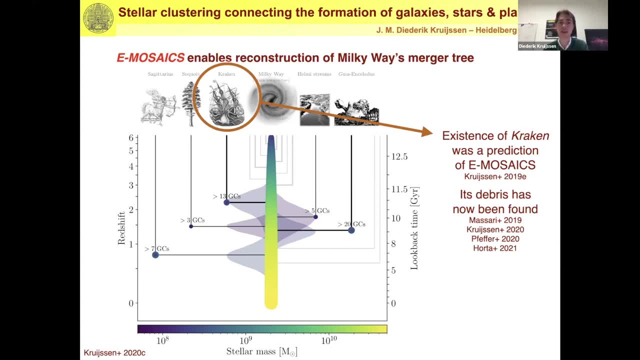 the stellar debris as well which is part of the bulge. So Kraken, basically the core of Kraken, made it in quite far into the Milky Way And that's very encouraging because it means that apparently we can be, we can have some confidence about the predictive power. 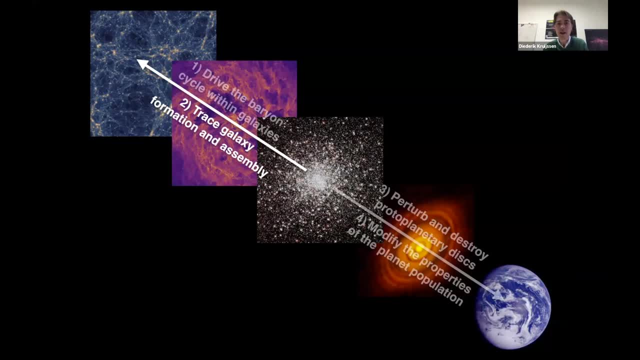 of the simulations. Okay, So that, for me, concludes the part of looking up towards larger scales. Now I would like to spend a little bit of time zooming in and seeing. okay, how does stellar clustering actually affect the properties of planetary protoplanetary disks during planet formation? 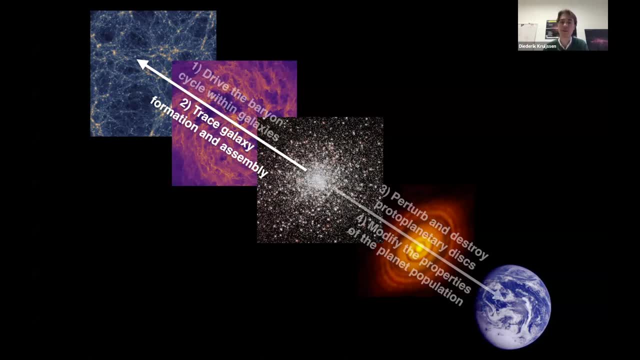 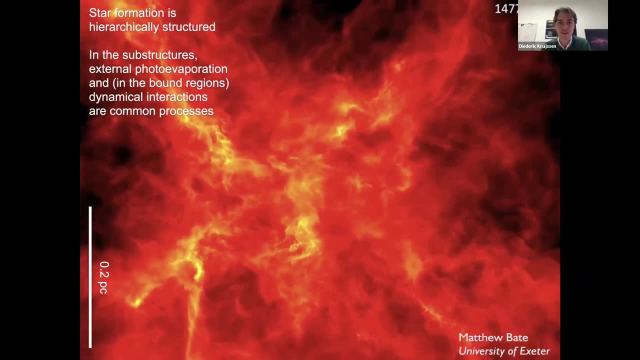 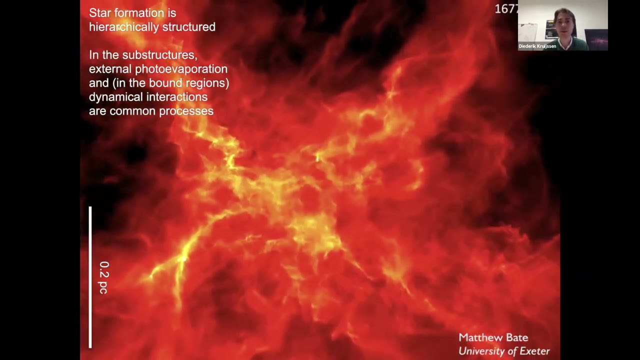 And how might it modify the properties of the planet population as we zoom in Now, as we, I think, have known for decades? at this point, star formation is hierarchically structured. If we look at the molecular clouds in the solar neighborhood. 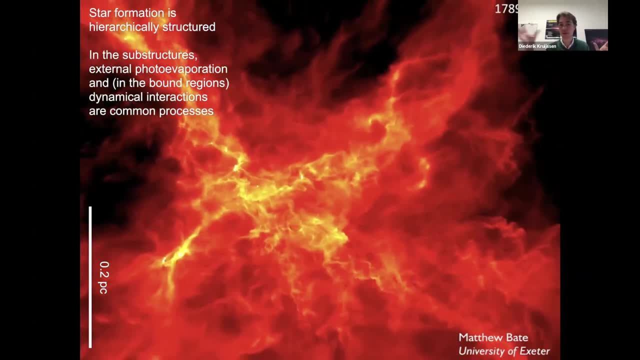 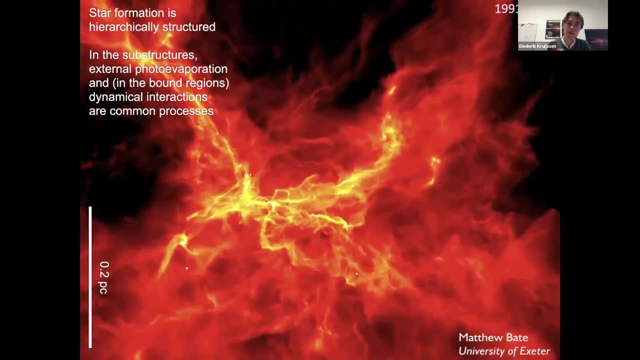 we see these very nice hierarchical structures And also in simulations, of course. these are well known, So I'm showing here the simulation by Matthew Bates. And in the dense substructures that you form this way, external photo evaporation by nearby massive stars. 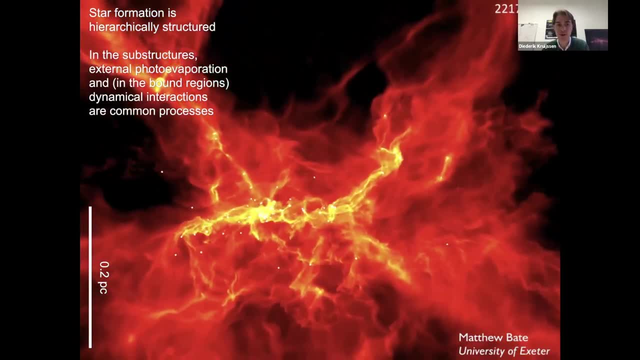 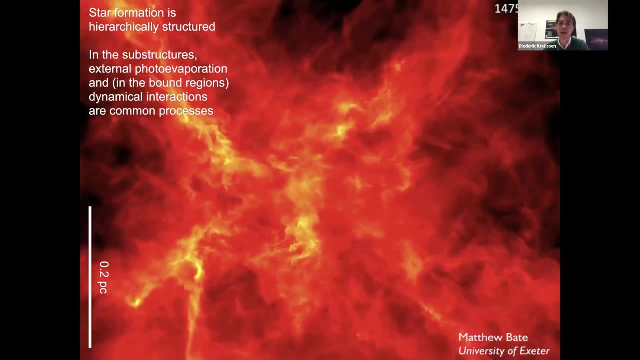 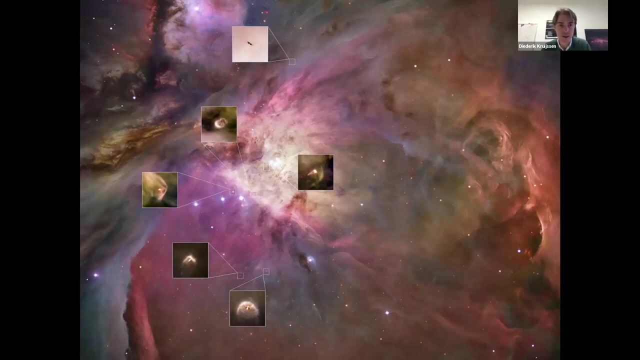 and also dynamical interactions between the stars are really common processes. In the simulation you actually see several of the stars being ejected dynamically. Now, observationally, we've known this for a while too, since the mid-90s. So this is a picture of the Orion Nebula Cluster taken with HST. 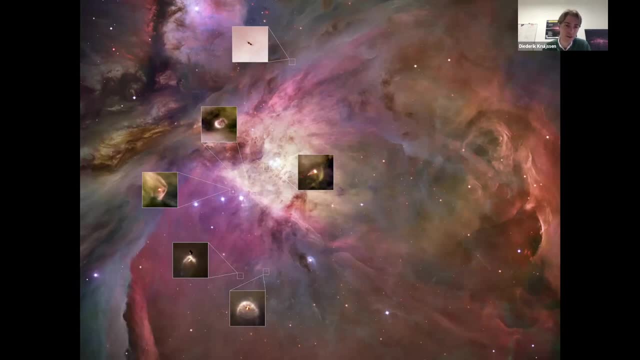 And in the mid-90s Odell and collaborators found these very nice protoplanetary disks that were irradiated by the nearby massive stars And the ionization fronts are really pronounced right, So you can see that the disks are actually being photo evaporated. 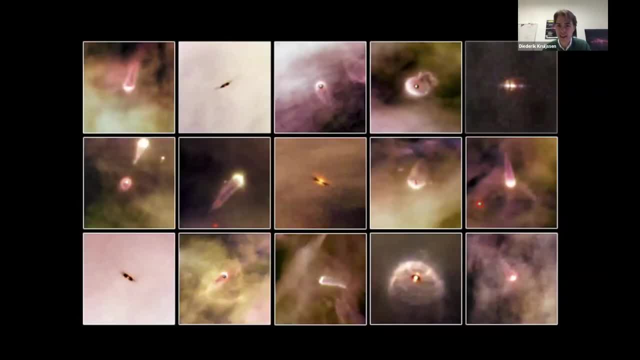 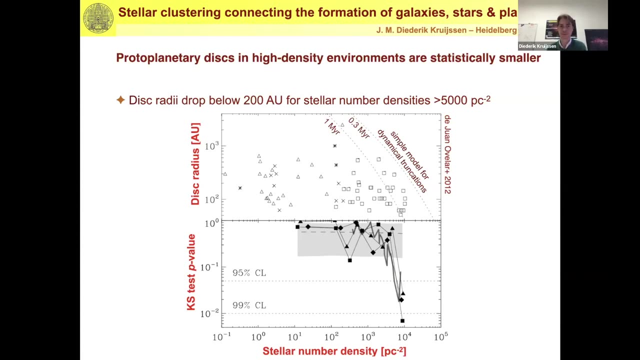 by these nearby massive stars And there was this entire zoo of protoplanetary disks with different morphologies due to this external irradiation. Now, interestingly, there are actually quantitative statistical differences between protoplanetary disks residing in different environments, And this is actually- this is the paper through which I kind of got interested. 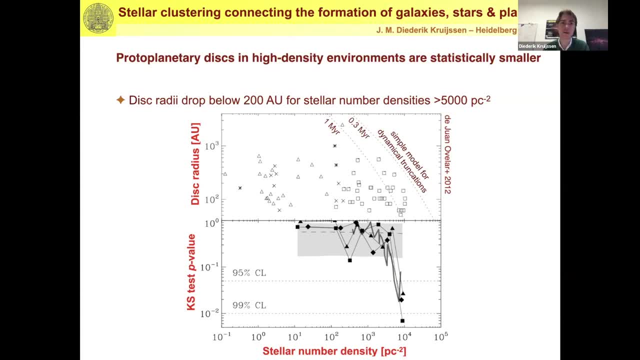 in this field. It was already from nearly a decade ago, But this is basically at the time was a literature paper and a literature compilation of known protoplanetary disk sizes, which are plotted here as a function of the projected stellar number: density. 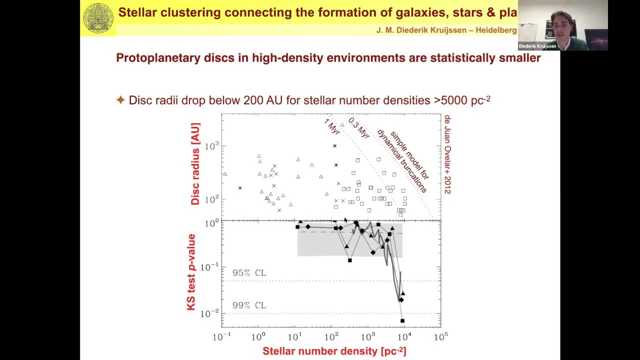 And then basically trying to compare the disk radius distribution as a function of that stellar number, density, and running statistical tests between all those bins to see if there was maybe a transition towards the high density end, And indeed it was at marginal significance at the time. 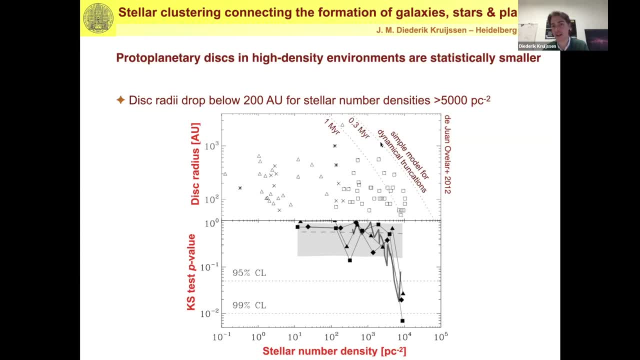 but we found the signal that the disk radius distribution was truncated at large radii once you started to get to those really high density environments. So these are all Orion Nebula Cluster disks, by the way, So there were no disks larger than 200 AU. 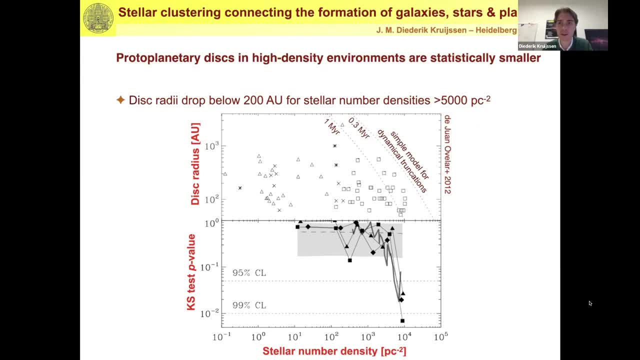 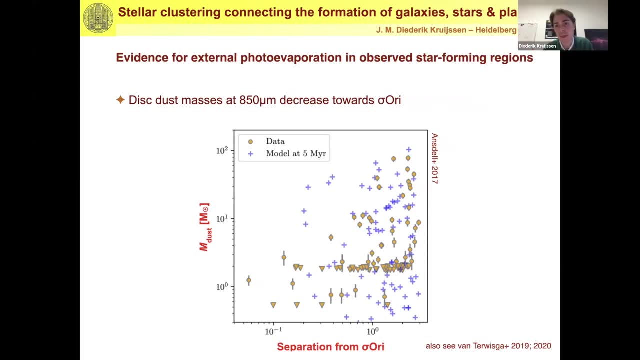 once you got above about 5,000 stars per square parsec. Now, in the years after it turns out actually, people started to measure disk masses with ALMA And this result kind of persisted. So this is now showing the dust mass of protoplanetary disks in Orion. 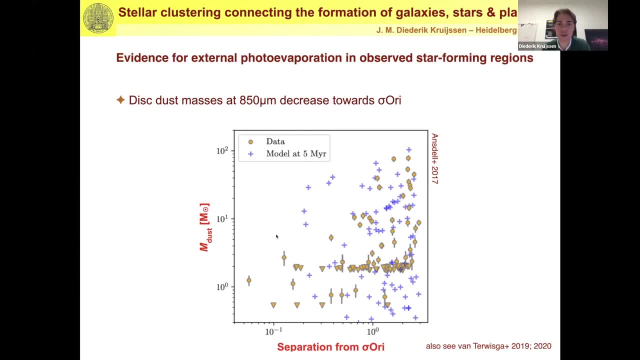 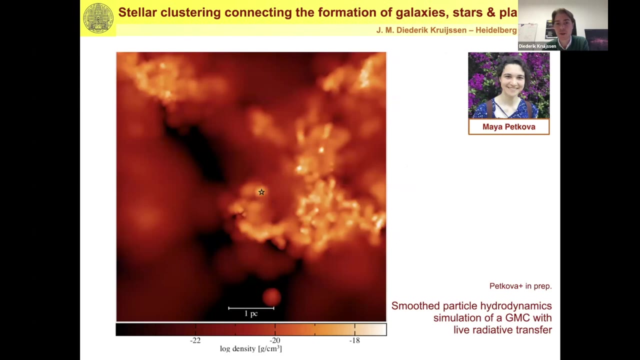 as a function of their separation from sigma Orionis, And what you see here is again: there's this dearth of massive disks as you get close to the massive star here, So that has led us to start thinking about how this could potentially be modeled. 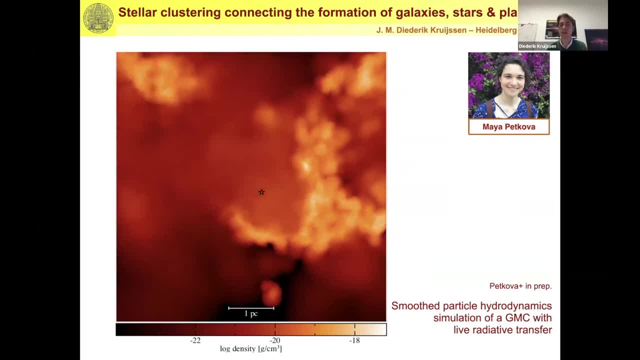 And this again is a very complicated problem. So this is just showing a little bit of preliminary work here. This is work by Maja Petkova here in Heidelberg, who has been developing a live radiative transfer scheme using voronoi tessellations that you can run live. 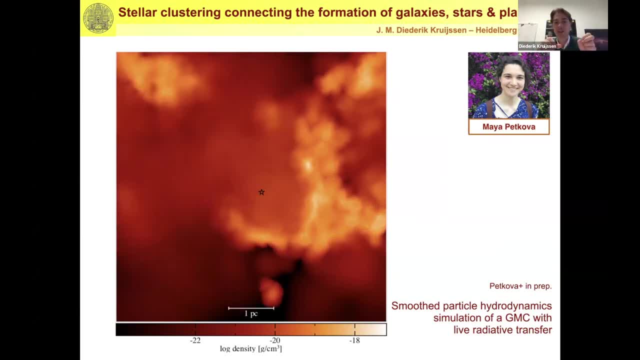 on smooth particle hydrodynamics And what you basically see is the moment you switch on this single ionizing source here in the middle, it very quickly ionizes the evacuated region here and starts to push this ionization front into the cloud And basically, with models like this, 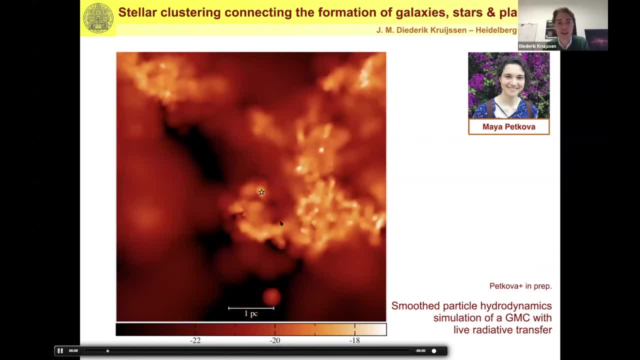 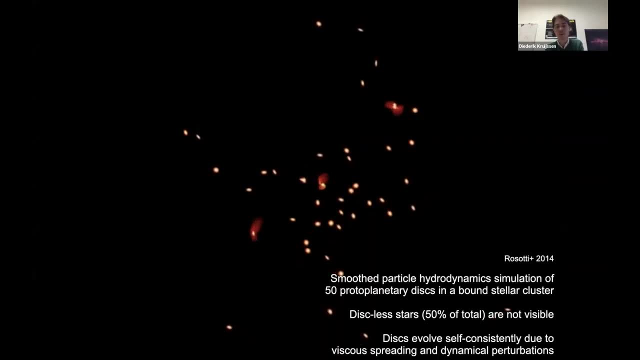 it becomes possible to start actually modeling the irradiation of the protoplanetary disks. So this is something we're currently working on, This aspect of the problem. The other side of the problem we have already modeled. So this is a stellar cluster of sort of trapezium size. 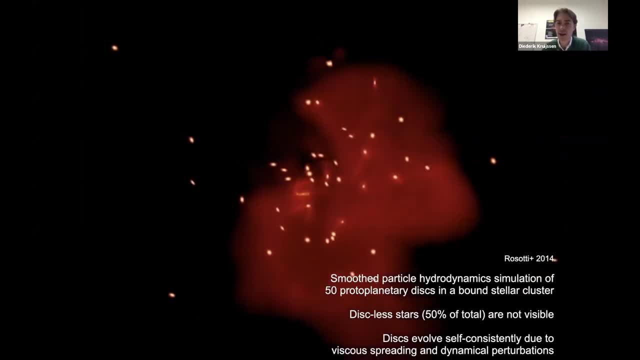 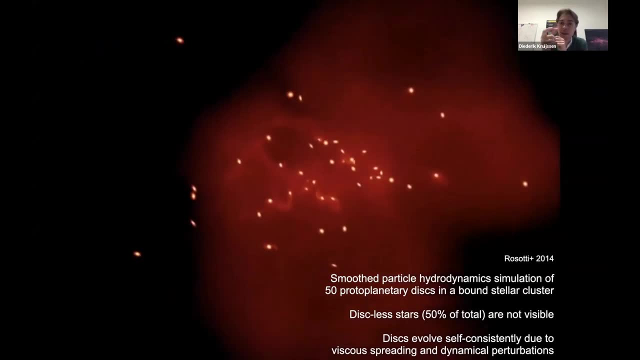 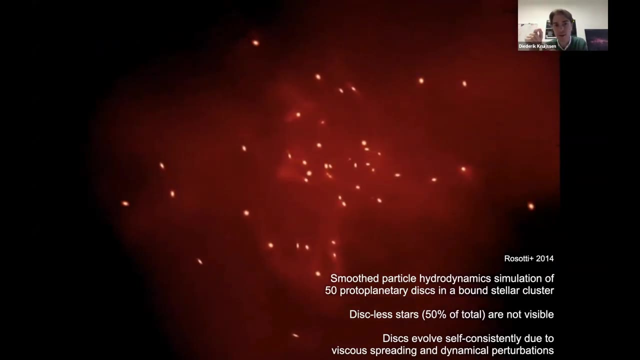 It's very small, but definitely trapezium density, And these are individual star particles that have single protoplanetary disks sitting around them And they're modeled in an N-body simulation And basically what you see here is those interactions between the stars drive these tidal tails throughout the cluster. 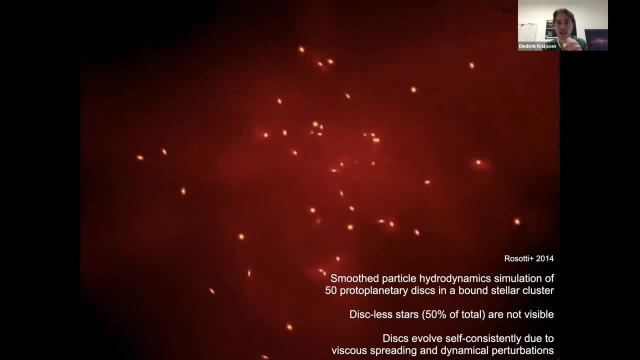 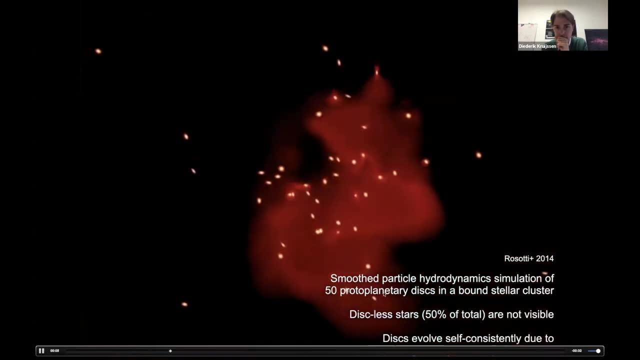 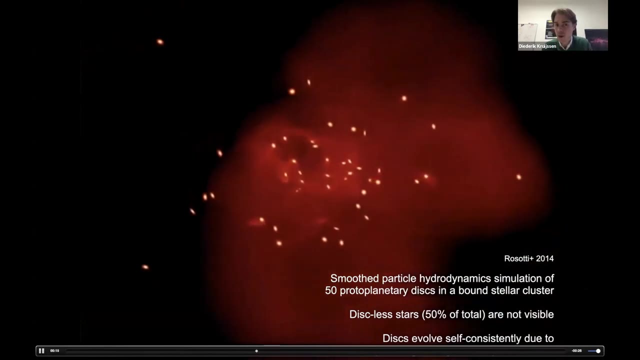 and start dispersing the protoplanetary disks. There are a couple of close encounters that really blow up the disk relatively close to the beginning of the movie. Yeah, here you can see them quite nicely, And this is a process that one might expect to happen. 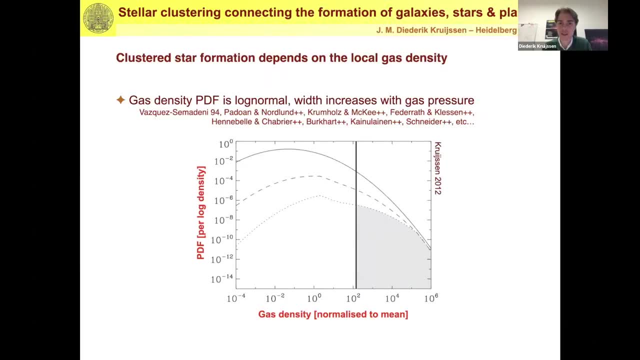 but obviously only in the very densest environments. So the question is now: if you look at those processes, when do they take place? under which conditions? which fraction of the stars that form have planetary systems or protoplanetary disks that actually are subjected to those conditions? 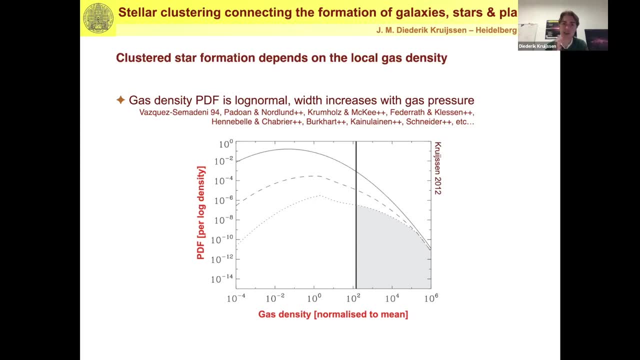 And to describe that you can use the gas density PDF which in the interstellar medium follows a nice log normal, and the width of that PDF increases with the gas pressure. So if you use that gas PDF, which is here the solid line, 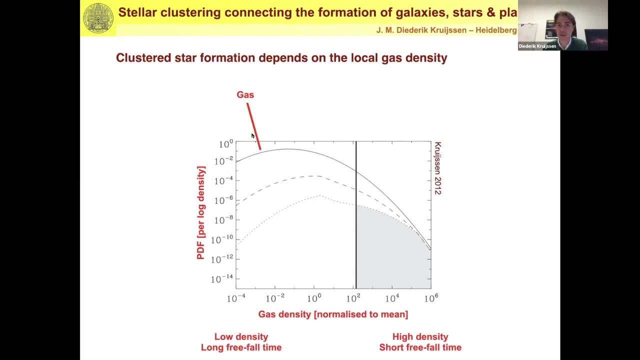 on the left what you have is low densities for long freefall times. On the right, you have high densities and short freefall times. So if you then let those pockets of gas form stars, then at the low end, because you have a long freefall time. 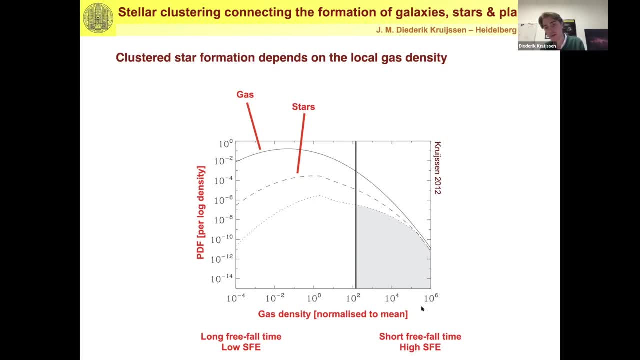 you will only form very few stars, but on the right, because you have a very short freefall time, you will form a lot of stars per unit time. So you get a high star formation efficiency on the right and a low star formation efficiency on the left. 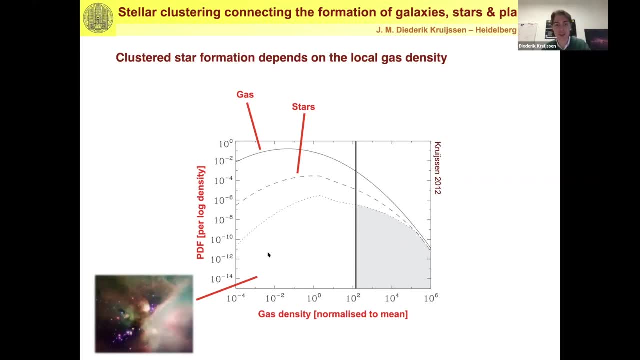 So basically, what you get is, at low gas densities you'll get stellar associations like the image you see here, and here on the right you'll get dense stellar clusters like protoglobular clusters. Now, this really is a critical ingredient. 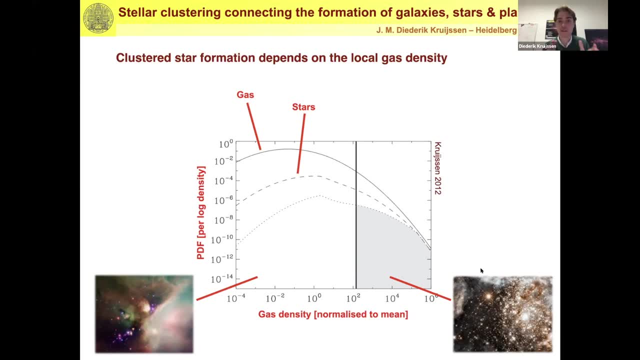 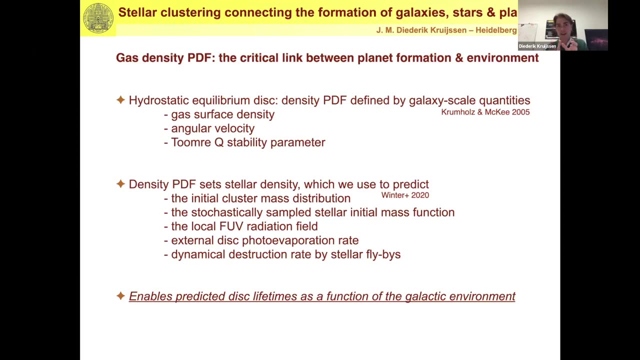 if you want to make a statistical prediction for what the environments are in which protoplanetary disks form and evolve. And the reason is that this PDF can be used to link basically between the galactic scale conditions and the small scale conditions. And the reason is that in a hydrostatic equilibrium disk, 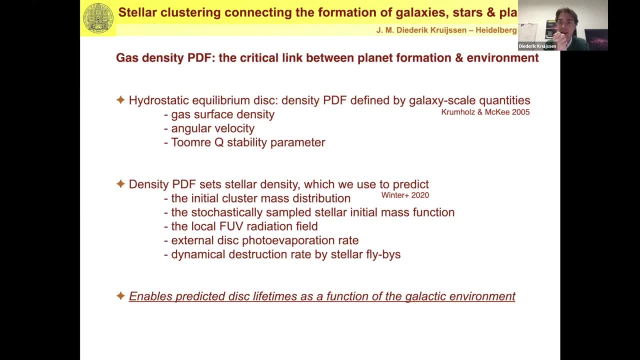 you can define the density PDF using galaxy scale quantities, basically just the gas surface density of your disk, how quickly it is rotating and how stable it is Galactic disk, not protoplanetary disk. Then that defines the PDF. but then within the PDF, using the PDF, 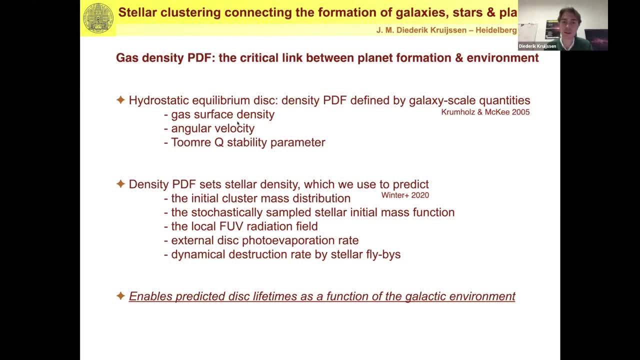 you can predict the stellar density and the stellar density you can use to predict the initial cluster mass distribution, how well stochastically sampled the initial mass function is. so, therefore, what your local far UV radiation field is going to be, what your disk evaporation, photo evaporation rate is going to be, 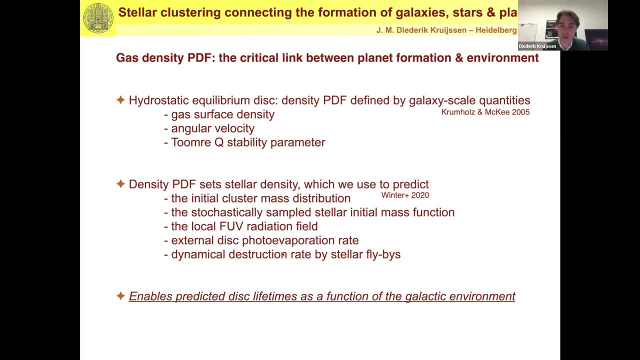 and also because you have the stellar density, what your dynamical destruction rate is by stellar flatness. So basically, what you can do with this is you can start to predict disk lifetimes as a function of this large scale galactic environment, And that's what we did here in this paper. 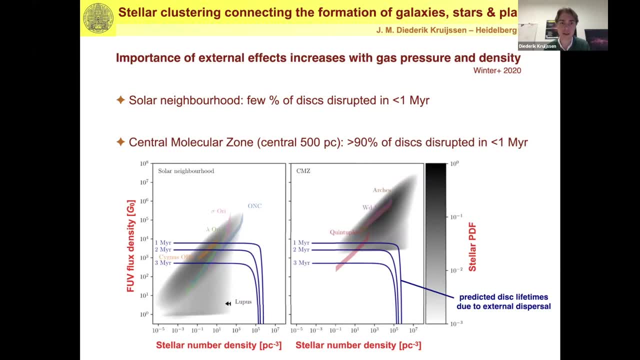 with Andrew Winter from early last year where basically we can, in the plane of far UV flux density versus stellar number density, we can predict where stars are forming. So we basically can take that 1D PDF of the density of the interstellar medium. 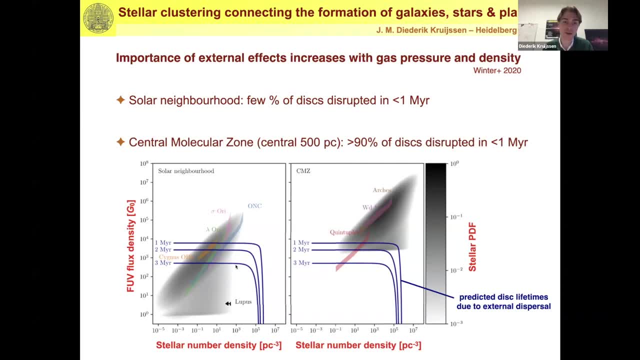 and turn it into this 2D PDF of what the formation environments of protoplanetary disks are. And that's the gray shaded histogram you see here. It's basically for solar neighborhood conditions where we expect stars and planetary systems to form, And now here over plotted for reference: 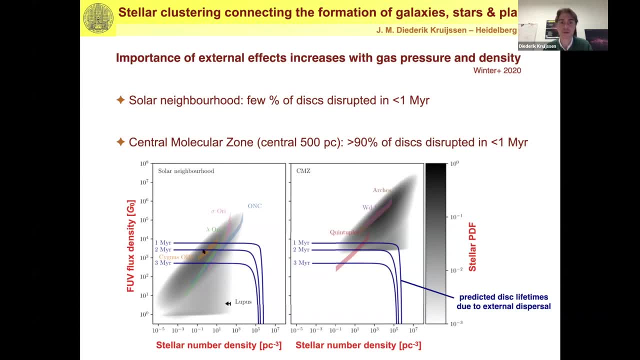 are a bunch of observed regions. So we see, actually we reproduce the observed regions pretty well And the blue lines are predicted disk lifetimes due to external disk dispersal And the horizontal part here is due to external photo evaporation. So if we have higher far UV strengths, 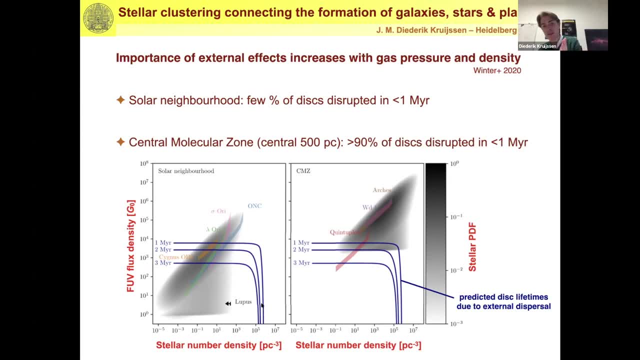 we get shorter disk lifetimes. And here the vertical part is from dynamical encounters with nearby stars. So we see basically that this part is rarely important for protoplanetary disks. In protoplanetary disks we really care about the photo evaporation. 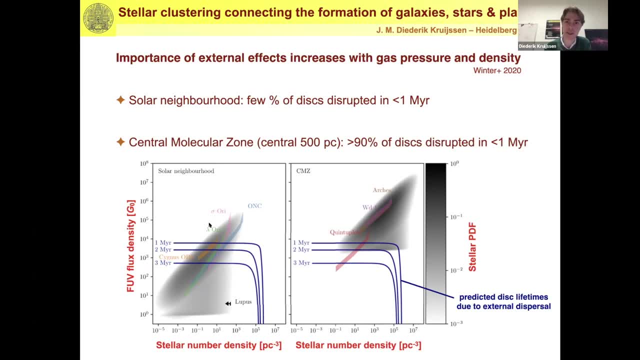 Now we see that in the solar neighborhood it's only a few percent of the disks that are actually disrupted within a mega year, So it's not that important. But if we now scale this to the conditions that are typical for the central molecular zone, 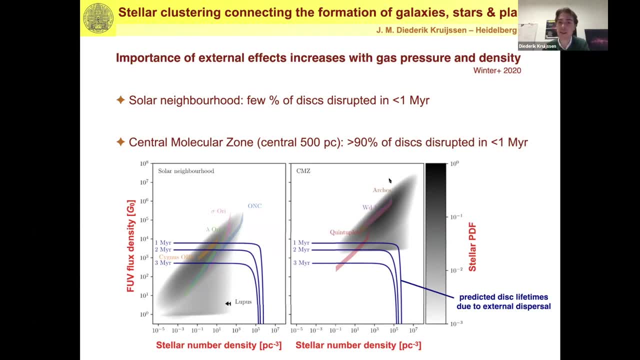 of the Milky Way. so near the galactic center, we see that, of the order, 90%, more than 90%, of the disks are actually disrupted by external photo evaporation in less than a mega year. And the reason that this is so important. 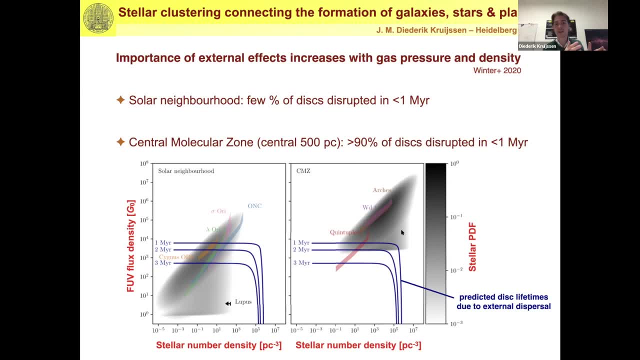 is that the conditions of the interstellar medium in the galactic center are quite similar to the conditions that the Milky Way interstellar medium experienced at high redshift. So the right-hand panel kind of gives us an idea of how most stars in the Milky Way actually formed. 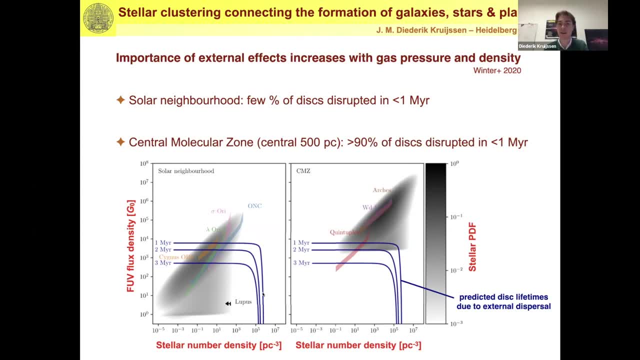 It's not what the solar neighborhood looks like at the present day. This is more what most stars in the Milky Way formed like, And I would bet that we probably- the solar system and us probably- could not have originated in such an environment. 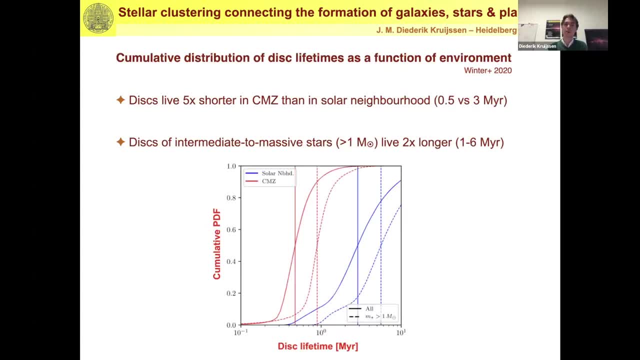 Maybe that is why we only formed now. So if we then look at what the disk lifetime PDFs are, we can be a bit more quantitative. We see that in the central molecular zone there's the red lines. here disks live about five times shorter. 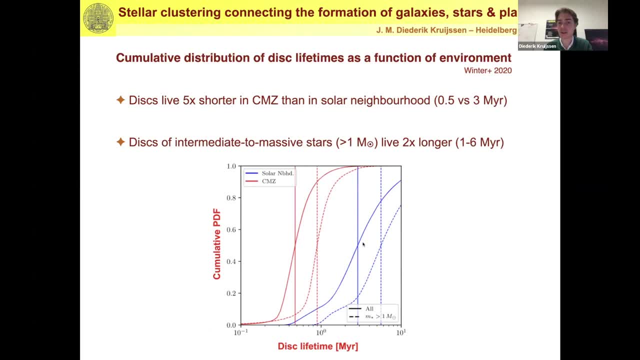 than in the solar neighborhood, And there is also a dependence on stellar mass. So the solid line here is for basically all the stars: If we restrict ourselves only to stars more massive than one solar mass, we see that the disks actually live a bit longer. 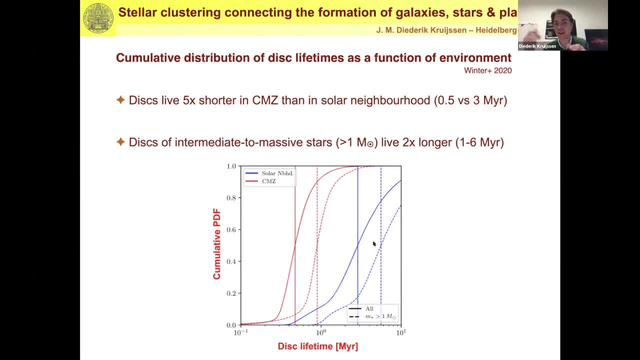 And it's because the binding energy of the star is larger, So it's harder to photo evaporate off the disk, basically. But what this means is that we get a really distinct imprint of stellar clustering on the protoplanetary disk- lifetime for most of the conditions of planet formation. 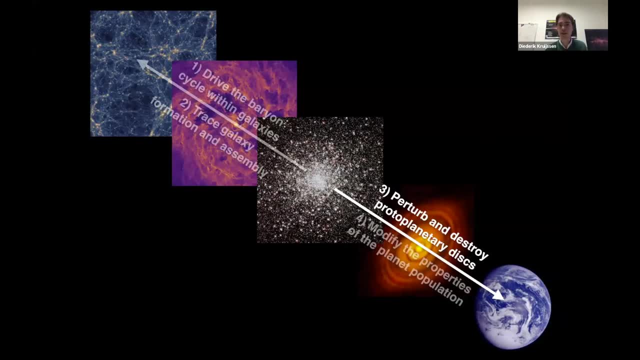 in the Milky Way's history. Now, of course, the question then is: does this actually affect the planet population or not? And this is an extremely important question, but very, very challenging, because most of the planets that we know have ages older than a giga year. 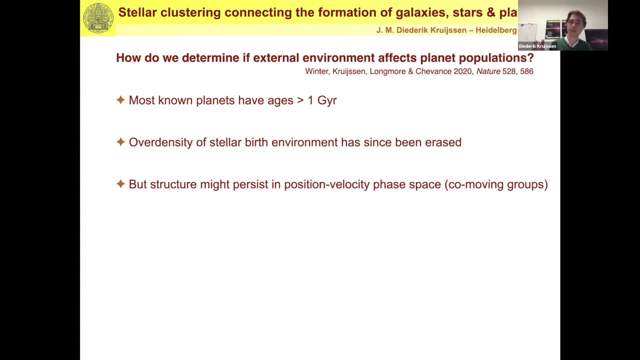 And what that means is that the overdensity that they formed in the overdensity of their stellar birth environment no longer exists. So, in order to answer this question, we can't just look for overdensities in physical space, But it might be possible that if structures have dispersed, 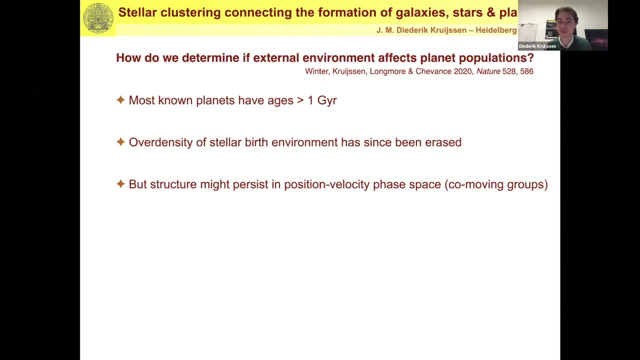 that they are still co-moving And that means that there might be structure in position, velocity, space, And with Gaia we've set out to test this. So we've, basically we've taken all known exoplanet host stars with known radial velocities. 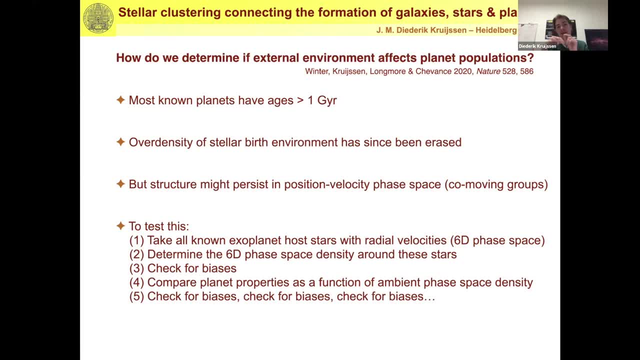 for which we had 60 phase space information, And we determined the 60 phase space density around those stars. We checked for biases, for instance dependence on host stellar mass and so on, And then we tried to compare the planet properties as a function of the ambient phase space density. 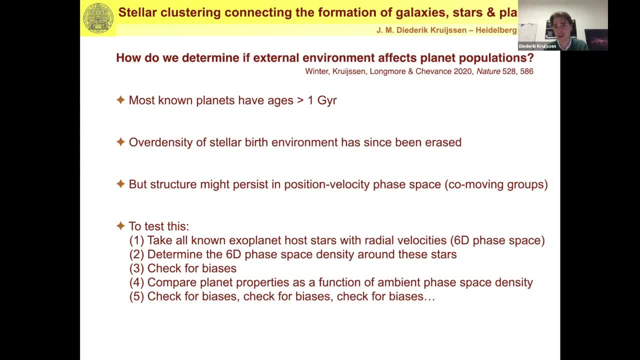 And I'm just going to reiterate that here. We kept checking for biases, and biases, and biases, And I'll come back to that numerous times because this is really important, right? The selection function of the exoplanet population is quite heterogeneous. 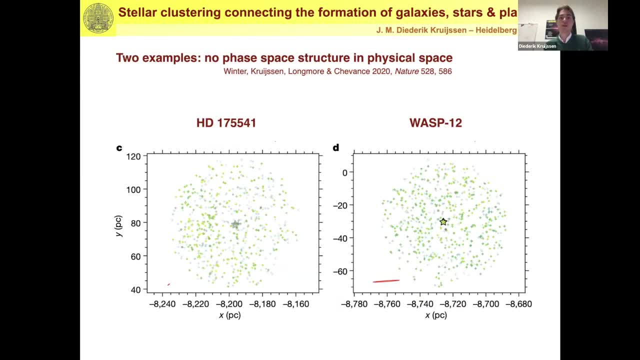 It's really important to be careful about this, So let me illustrate briefly how this works. So this is showing for two different planetary systems. So HD phone number and WASP-12 is showing what the physical space distribution is of stars in their vicinity. 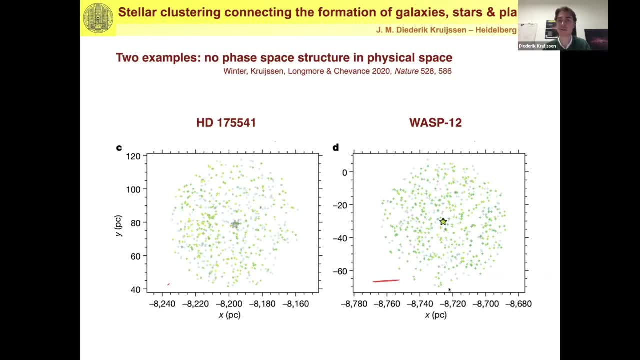 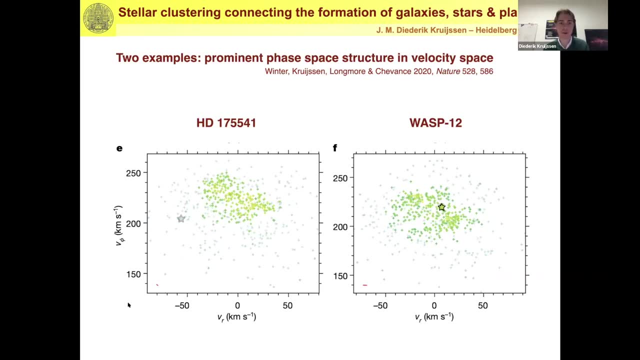 And you see immediately there is no structure here. This is just a flat density field. But if we now go to velocity space, so this is showing galactic radial velocity and galactic azimuthal velocity. there is phase space. There is phase space structure right. 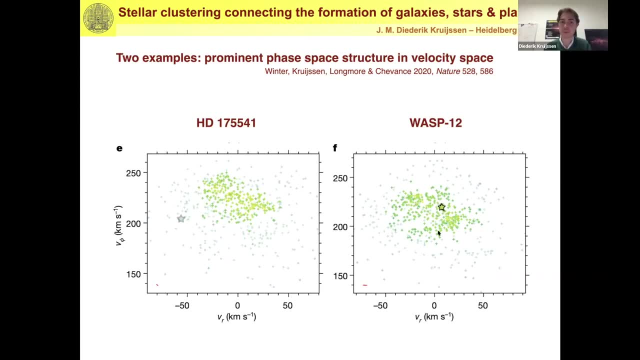 So there's a very nice overdensity here And there's another one here. So what we then do is, for each of those stars that you see here in the field of view, we calculate what the local phase space density is and we draw a histogram of that. 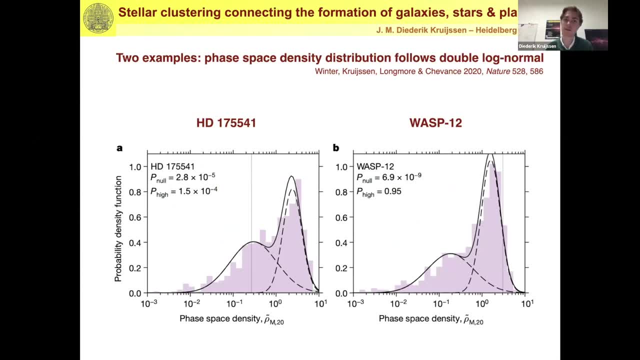 And what we found is that, for the vast majority of the stars for which we did this, the phase space density distribution in the immediate environment can be described by a double log normal. So what that means is there was a low density component, which I'll refer to as field. 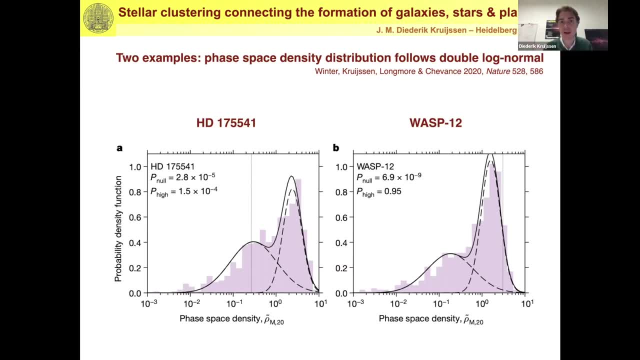 and there's a high density component, which I'll refer to as overdensity, And we carried out a Gaussian mixture model of these bimodal distributions to then assign a probability to each planetary system that it belongs to the field component or to the overdensity component. 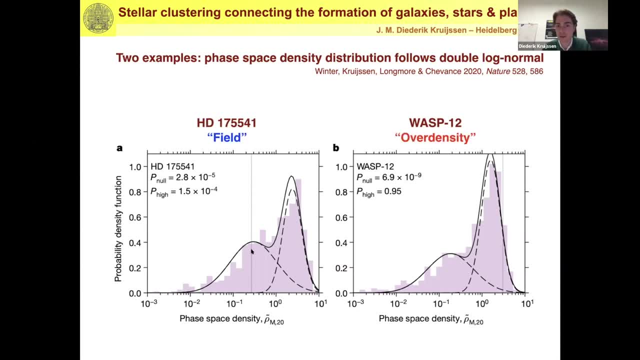 The one you see here on the left. so the vertical line indicates where the planetary system is sitting. the one here on the left has a very high probability. that's part of the low density component, whereas the one here on the right has a very high probability. 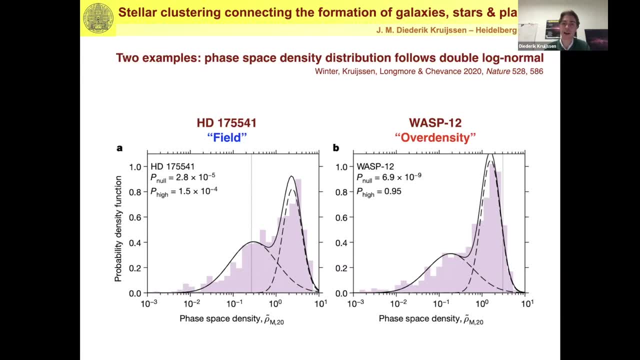 of being part of the overdensity So that we can then use to classify the observed planet population. Now, an important thing to add is this measures the current phase space density. We do not know if this reflects the birth environment of the planetary system. 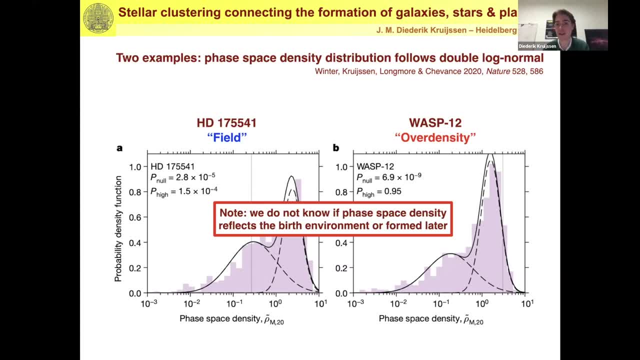 It might be possible that this formed later through resonances in the galaxy. We're sitting quite close to co-rotation here in the solar neighborhood, and Gaia has found overdensities that seem to be associated with galactic structure rather than birth structure. 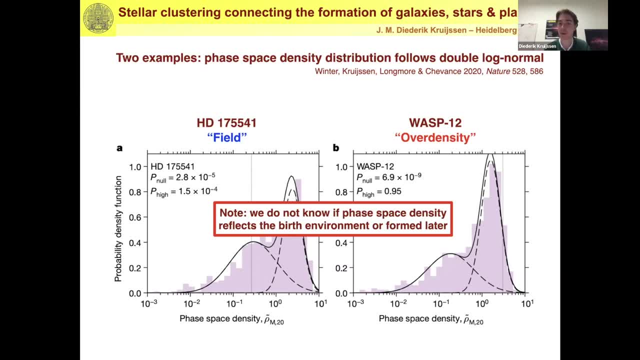 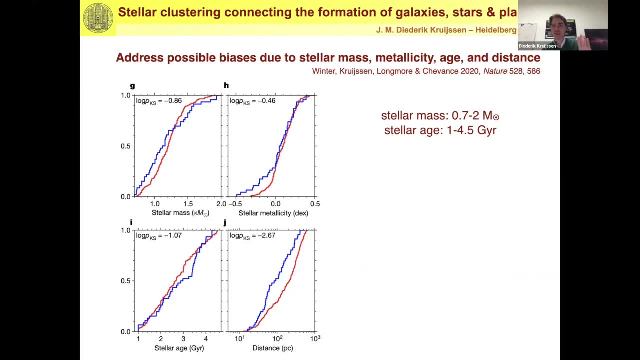 And I personally actually think it's related to that more than birth structure, but we can talk about that. Okay now, before I show you how the planet populations differ between overdensities in the field, I first want to check biases, because that is important. 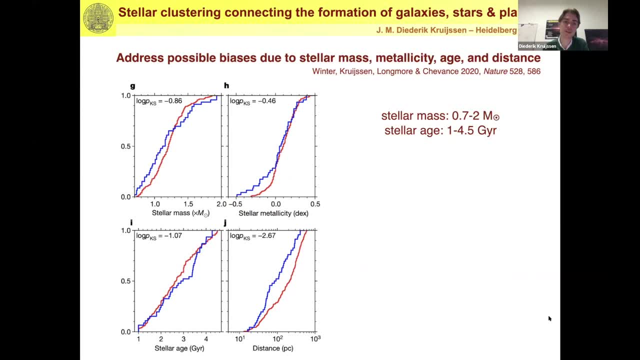 So what is shown here is the cumulative distribution function of the host stellar mass, the stellar metallicity, the stellar age and the distance for overdensities in the field And throughout the figures, overdensities are red and the field is in blue. 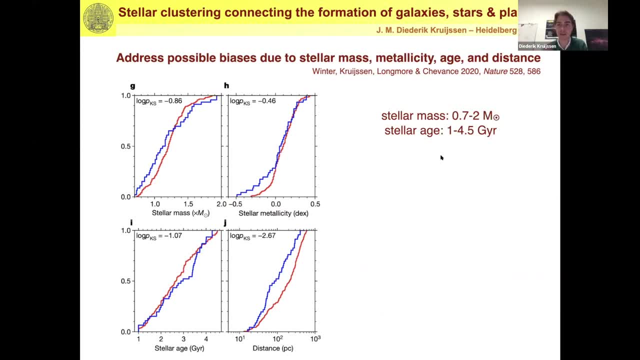 What we did is we applied stellar mass cuts and stellar age cuts to make them consistent across both samples And, as you see here, indeed, the stellar mass, metallicity and age are basically statistically indistinguishable. They're consistent with being drawn. 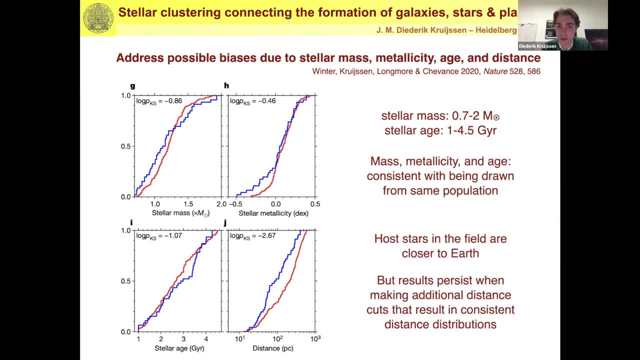 from the same population. This is not true for the distance. So you see that there is actually a significant difference here, It turns out. if you so we made an additional distance, cut at 300 parsecs, then the distributions are indistinguishable. 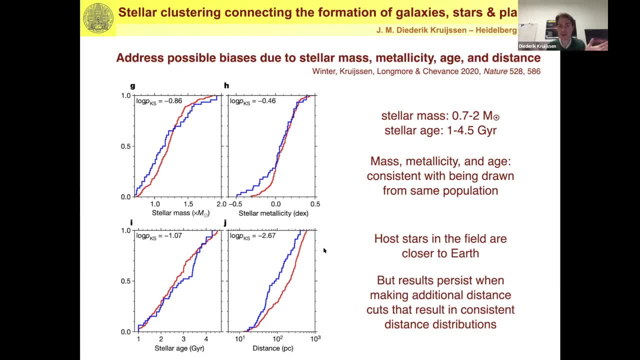 And it turns out our results that I'm about to show actually persist. So this distance difference is just there. It turns out overdensities are a little bit further away than pure field on average, but it does not actually affect the results, Okay. 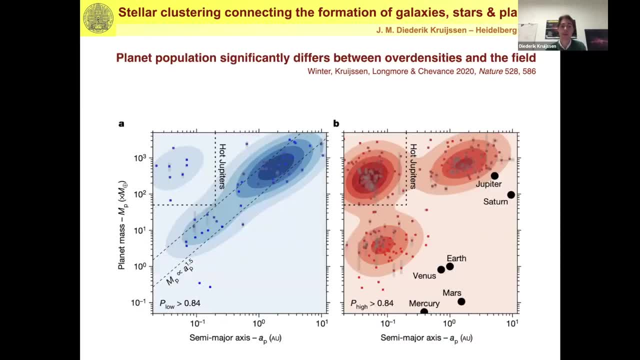 So the result is, in short, is this: So this is showing the planet mass on the y-axis as a function of the semi-major axis of which the planet is orbiting, And on the left I'm showing field systems, And on the right, 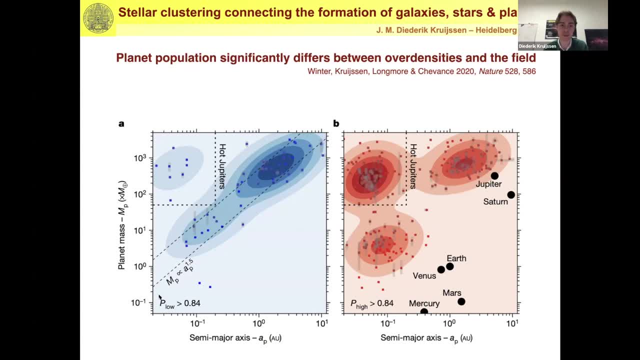 I'm showing systems in overdensities Here, defined through cuts in the Gaussian mixture model, p-value, which component the system belongs to. Now, the immediate obvious difference here is if you look at the hot Jupiter corner of the plot- is that there is a major difference. 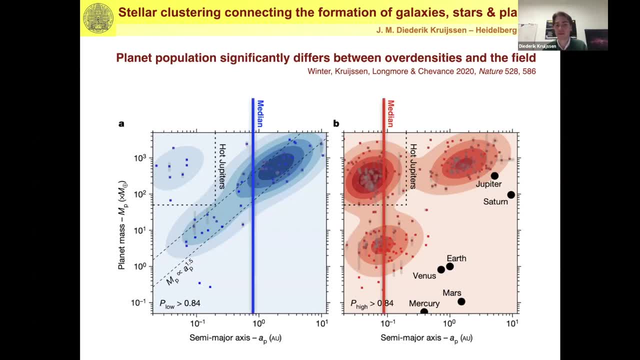 between both. But the first order. you can first quantify that just by looking at the median semi-major axis, which differs quite a bit, which differs by an order of magnitude between both samples. So in overdensities, the semi-major axis is a factor of 10 smaller. 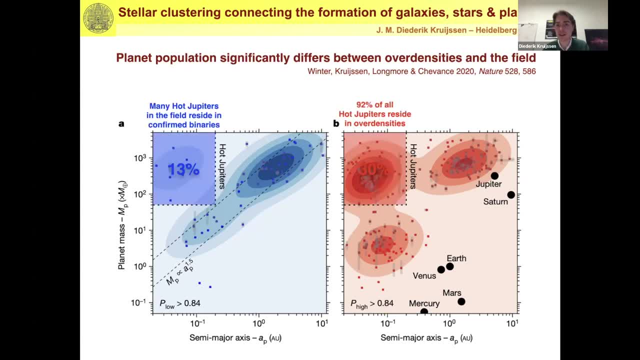 than in the field. But indeed then if we look also at the combination here in hot Jupiters, many, most of the hot Jupiters in the entire sample actually reside in overdensities- 92%. And then if we look at the few hot Jupiters, 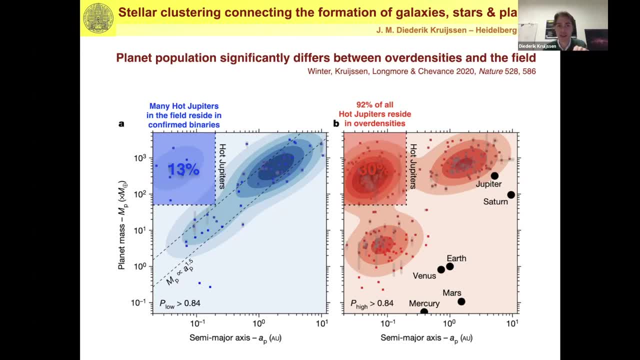 that actually reside in the field. many of them sit in confirmed binaries, So it seems that these might have been, might have become hot Jupiters because they were perturbed by binary, whereas on the ones on the right might have become hot Jupiters. 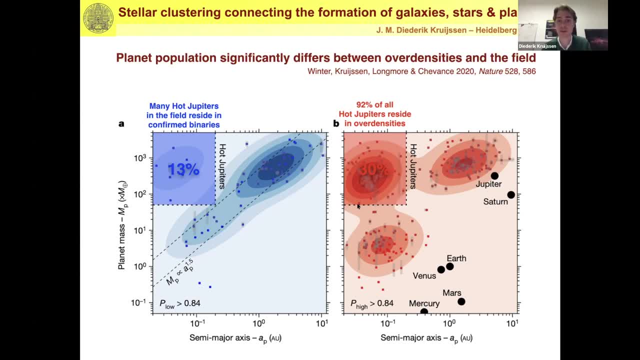 because they reside in overdensities, or at least that's the strong suggestion that's being made here. There's also a difference here, by the way, at the low mass end in the radius distribution, Although of course we can't see any planets here. 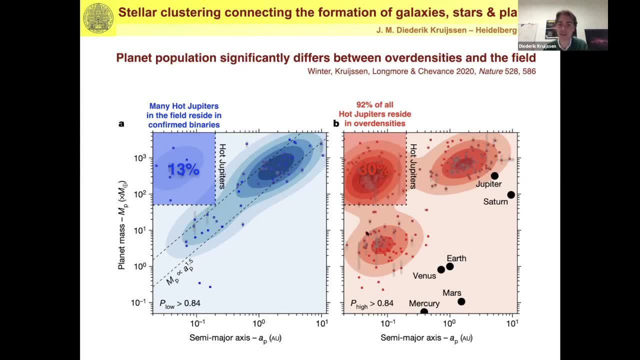 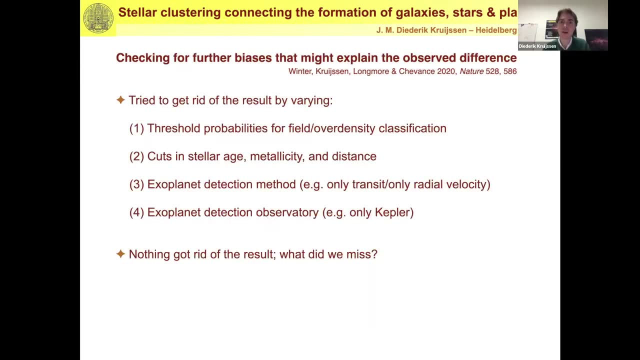 but there is a very distinct scattered population here, whereas this one seems to be well-behaved and follow this rough trend. So we spent a year trying to get rid of this result. We tried varying the threshold probabilities for the classification of field and overdensities. 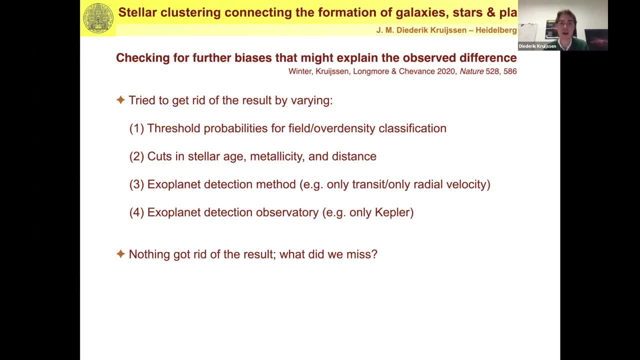 We tried all kinds of cuts in stellar age, metallicity and distance. We restricted exoplanet detection methods, only looking at transit detections or only radial velocity detections. We even restricted ourselves to only Kepler planets, et cetera, and we were not able to get rid of it. 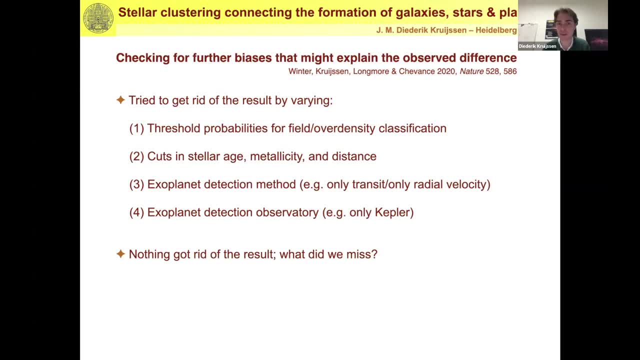 So if anyone has an idea of some bias that we should have checked, something that we might have missed, please tell me, because at some point we decided to just write it up and submit it, but it is still entirely possible that we missed something. 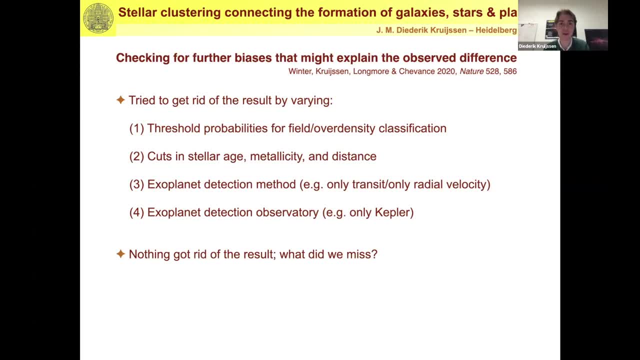 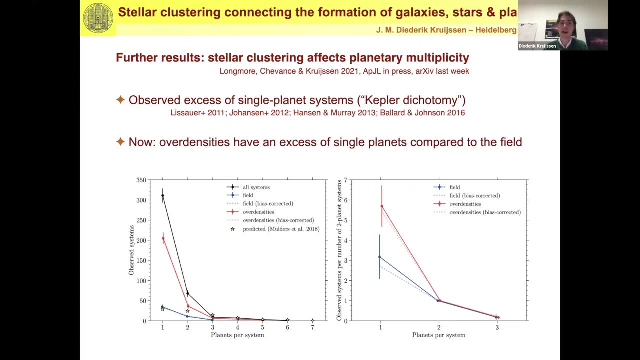 and we're still checking everything on a regular basis. But the result so far is that stellar clustering does indeed shape the properties of planetary systems, And this extends further. So we've had a set of follow-up papers where we looked into this further. 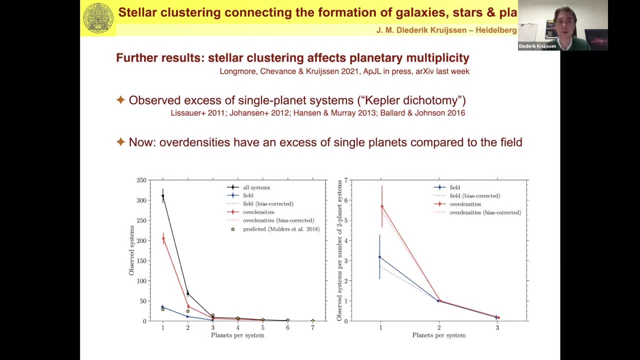 So one other result that we found here in a paper by Steve Longmore is that stellar clustering affects planetary multiplicity and there is a very well-known excess of single-planet systems in Kepler. It's called the Kepler dichotomy. It's basically 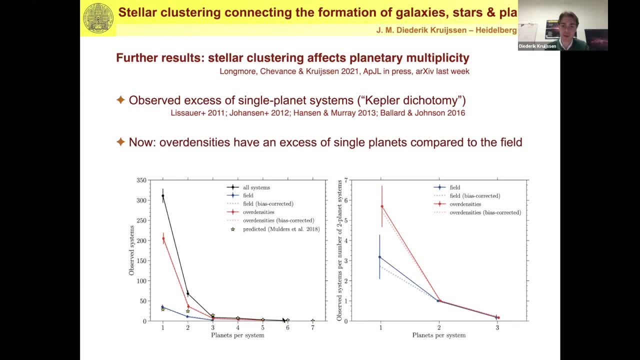 if you look at the multiplicity here, then simple models basically predict the yellow stars. and then Kepler finds this huge excess of single-planet systems. Now what we find is that that excess of single-planet systems is actually driven by overdensities. 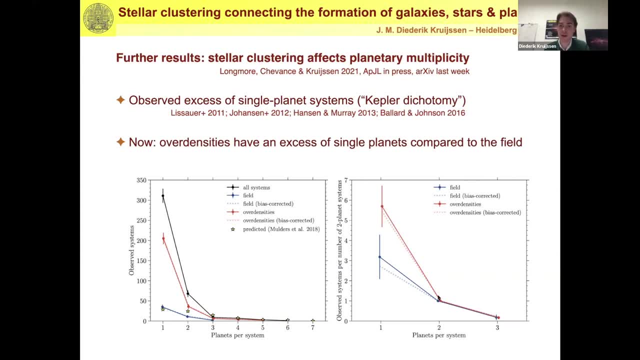 Sure, the field also has a slight excess of single-planet systems, but overdensities much more strongly so. So that is a suggestion that maybe overdensities play a role. so stellar clustering plays a role in driving this Kepler dichotomy. 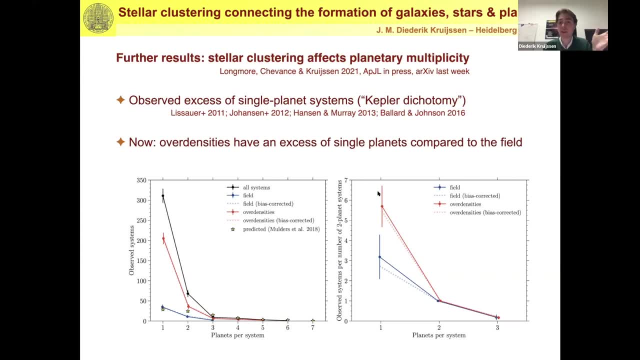 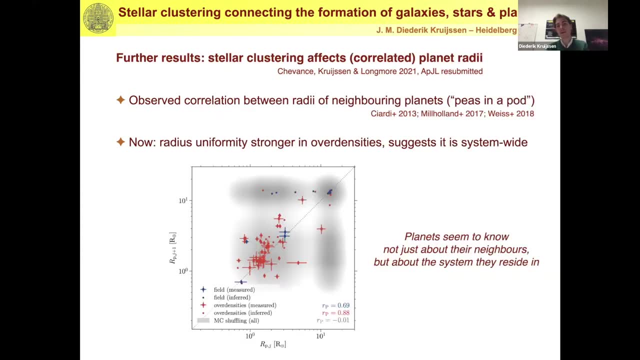 Basically, I would say maybe planetary systems are dynamically perturbed and that is why, actually, we get these single-planet systems Now. another main Kepler result is that similar, or that the planets have similar neighbors, So neighboring planets have similar properties. 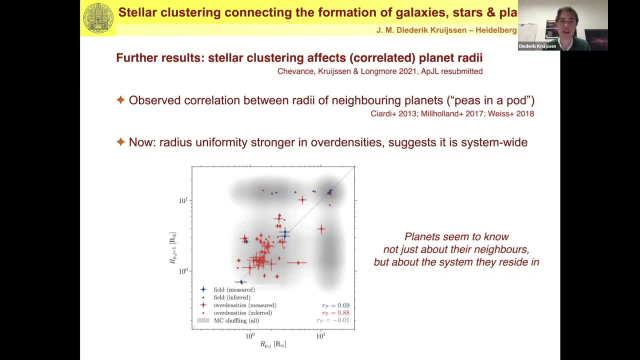 They have similar radii and they actually also have similar masses. And this behavior has been called a peas in a pod. And this uniformity of radii, where basically the radius of an inner planet is correlated to the radius of its outer neighbor. 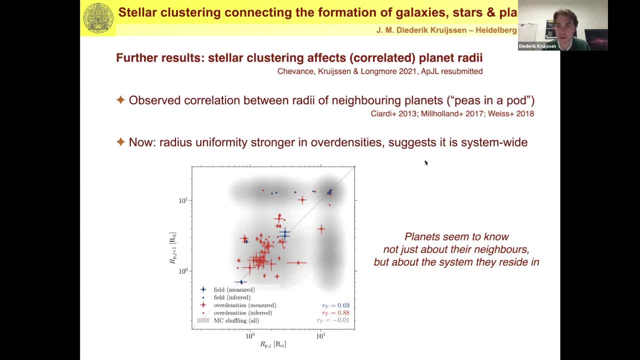 that correlation is actually a little bit stronger in overdensities. Now, if we go with the hypothesis that these systems have been perturbed and have been shuffled around, then it means that this uniformity of planet properties is not between neighbors but is actually system-wide right. 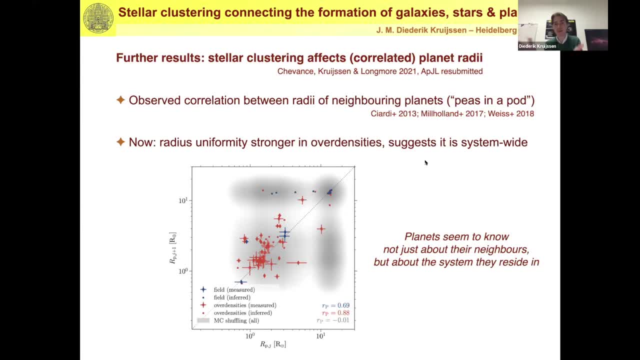 If you shuffle around the orbits and therefore change the neighboring order, then it means okay. if the correlation is actually a little bit stronger in overdensities, then it means we're actually correlated on a system-wide scale rather than just between neighbors. 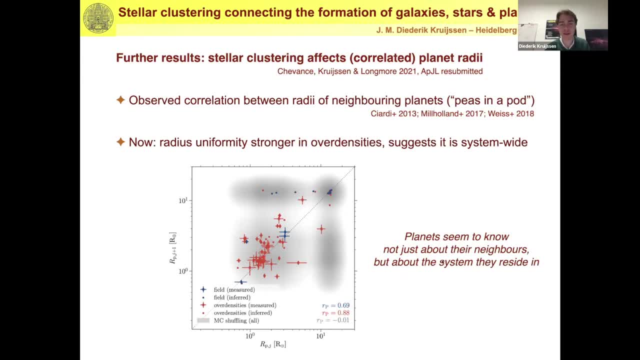 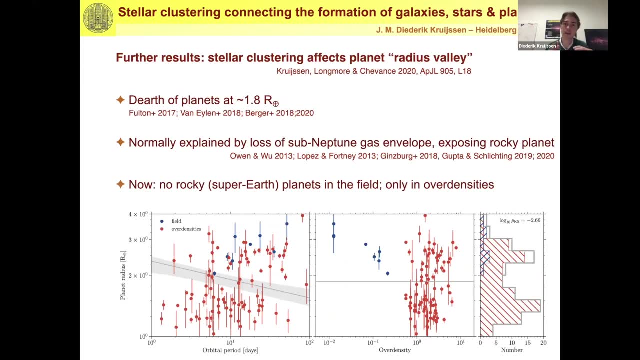 And that is interesting. So planets seem to know not just about their neighbors but actually about the system that they reside in. And then finally it actually has stellar clustering might actually affect sort of atmospheric properties of planets as well. So a third key Kepler result. 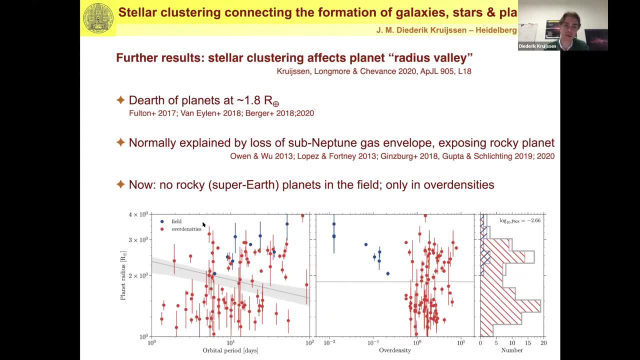 is that there is this radius valley, where above this sort of gap in radii you've got sub-Neptunes, which are very gas-rich hydrogen-helium envelopes, and below here we've got super-Earths that do not. 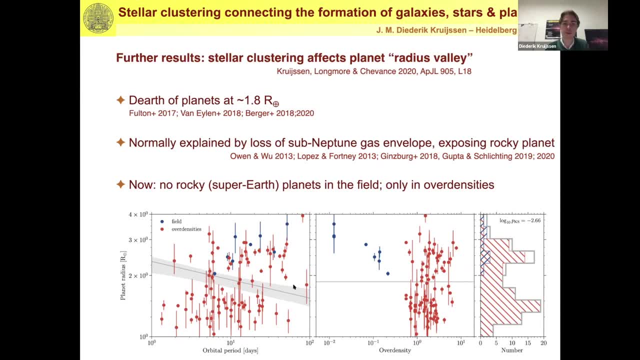 And there are various different hypotheses for what might be what might drive this radius valley, But typically the hypothesis is that basically this sub-Neptune gas envelope is lost and therefore the planet ends up below it, And ideas are things like evaporation from the single-house star. 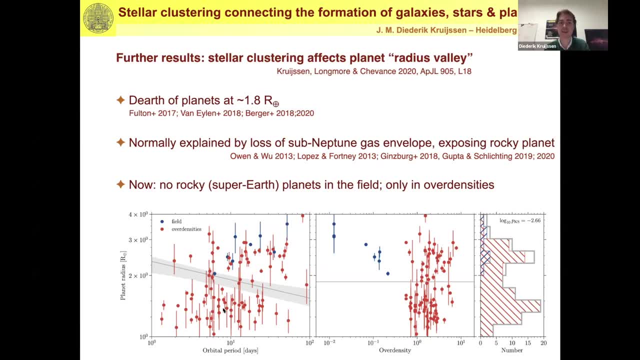 or basically heating from the core of the planet itself that slowly sheds the atmosphere. What we see here is that only overdensity planets are actually below the radius valley. In the field they're all above, which suggests that maybe overdensities that are clustering play a role. 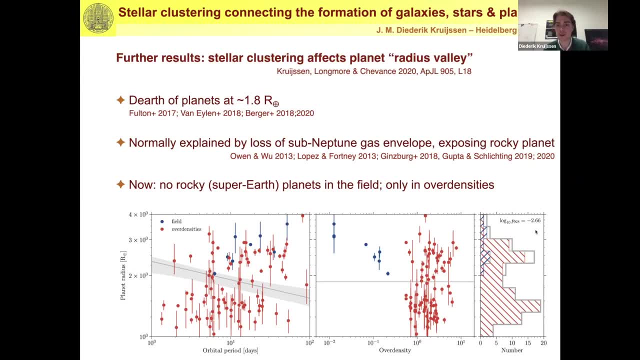 in helping planets get rid of their atmospheres. Now, of course, it's small numbers, but it is statistically significant. So it's still preliminary, but who knows what we'll find over the next year or two. Okay, That concludes what I wanted to say. 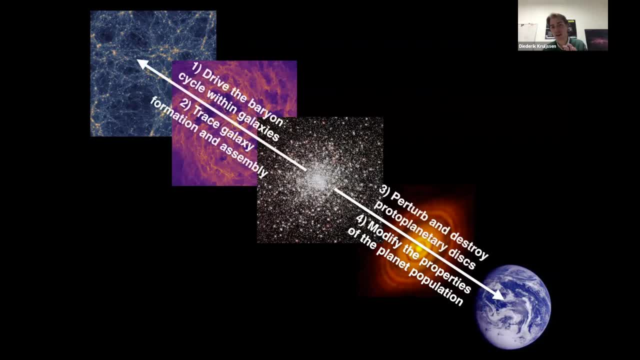 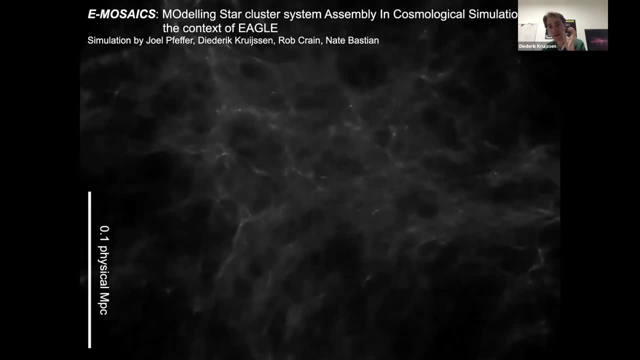 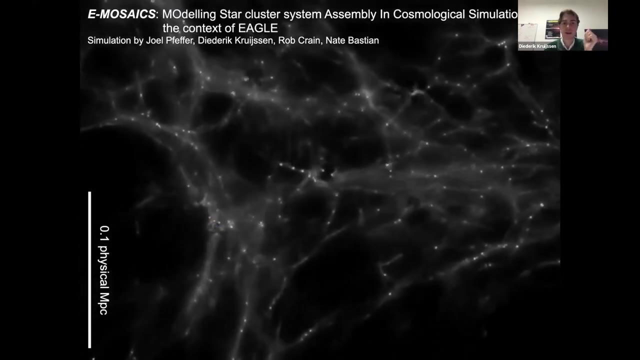 about the planets here, And I would like to zoom out very briefly to bring this all together, Because in EMAZEGS we can look at how the clustering of stars at birth varies as a function of redshift throughout cosmic history, And that is what I'm showing here. 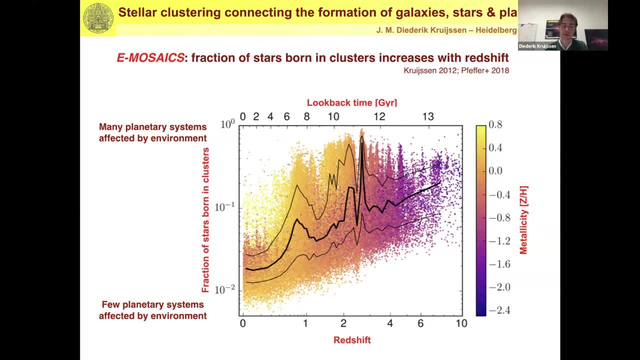 So this is showing what I mentioned when I was talking about EMAZEGS before. This is showing the fraction of stars born in clusters, the cluster formation efficiency as a function of redshift in one of our Milky Way mass zoom-in simulations. 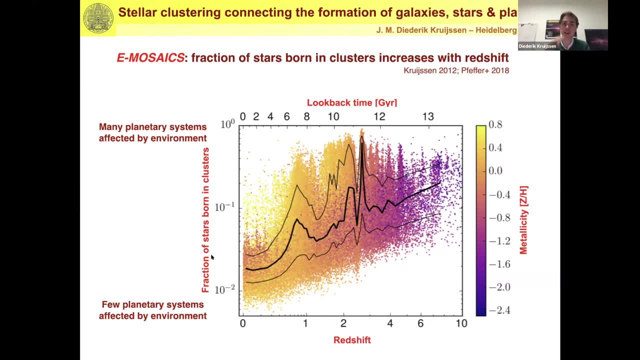 And this is a very consistent prediction, as the fraction of stars born in clusters increases with redshift, simply because the gas pressure and gas density is higher at higher redshift. What this means is that at higher redshift, many more planetary systems were affected by their environment. 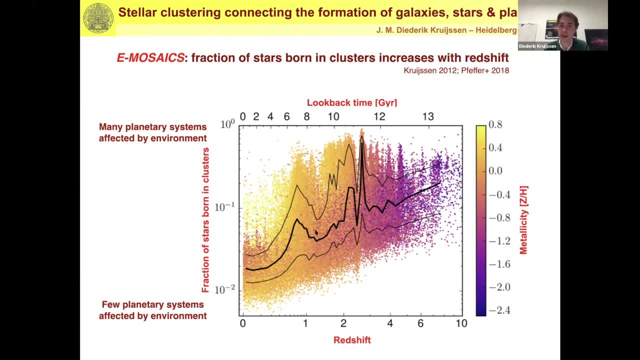 than at low redshift. One thing you might notice here is those spikes. Those spikes are galaxy mergers. These are galaxy mergers that increase the gas pressure within the galaxy and therefore drive a higher cluster formation efficiency And therefore, as a result of the results. 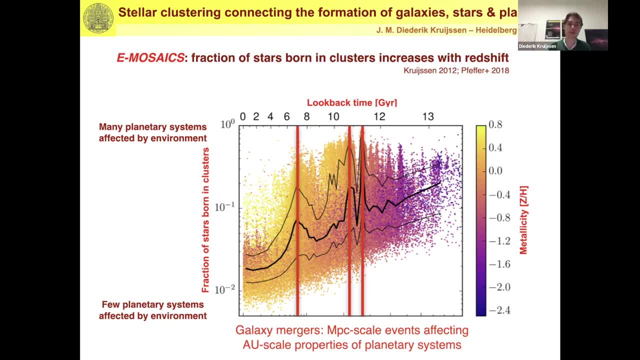 that I just showed, correspondingly more environmental perturbation of planetary systems. So these are really, these are mega parsec scale events that affect the AU scale properties of planetary systems, And I think that is an extremely exciting idea that these types of processes 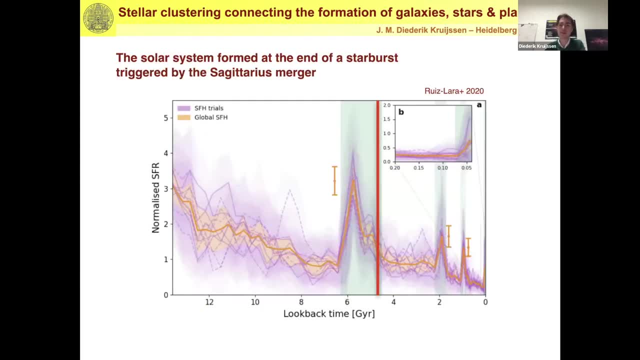 cross such a wide dynamic range And there is actually a recent result about the solar system here. This is showing the star formation history of the solar neighborhood. It turns out the solar system formed here shortly after a starburst that was triggered by the Sagittarius merger. 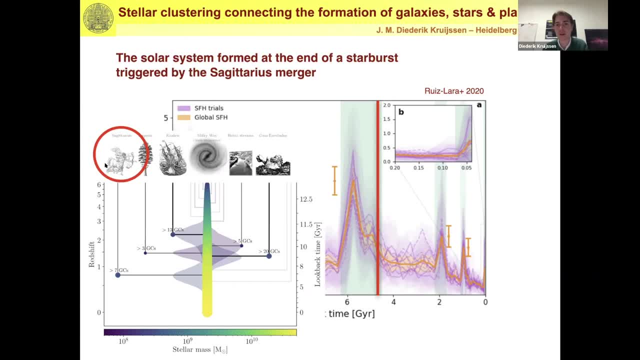 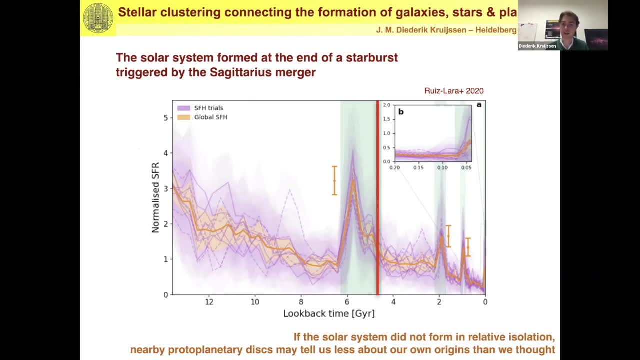 Right, This is the merger that we identified here in the merger tree earlier. So that's interesting. If the solar system did not form in relative isolation, then maybe nearby protoplanetary disks tell us less about our own origins than we might have thought. 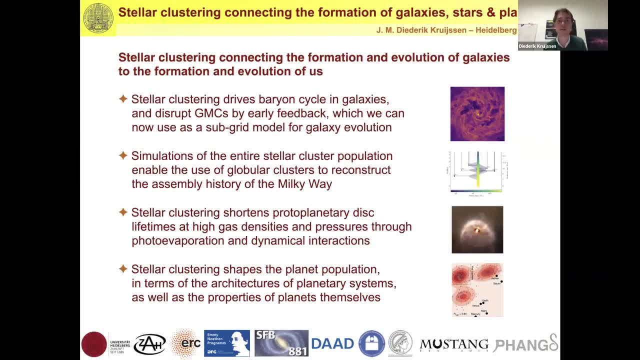 Maybe Okay With that, I would like to conclude. I apologize for going a little bit over. Basically, the theme of this talk is: to what extent does stellar clustering connect the formation and evolution of galaxies to the formation and evolution of us? 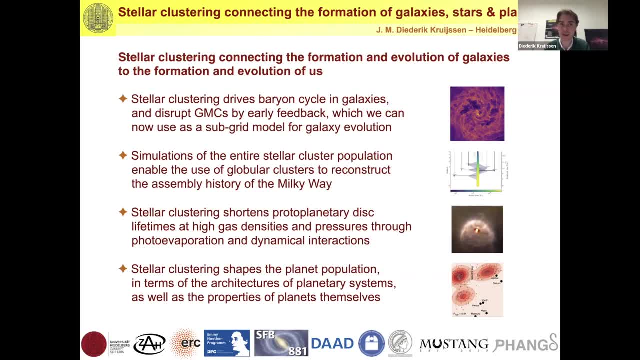 And I would argue that it does. Stellar clustering drives the baryon cycle in galaxies. It disrupts giant molecular clouds by early feedback And we can actually take that now from observations and use it as a subgrid model for galaxy evolution. And then, once we've described 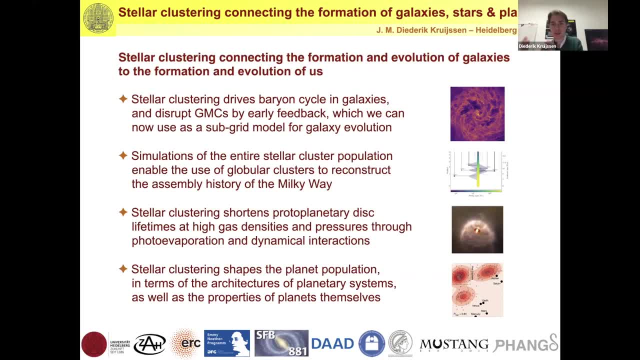 the interstellar medium. well, we can start using the simulations of the galaxies that we get to describe the stellar cluster population from high redshift till the present day and use those globular clusters to reconstruct the assembly history of the Milky Way And throughout that. 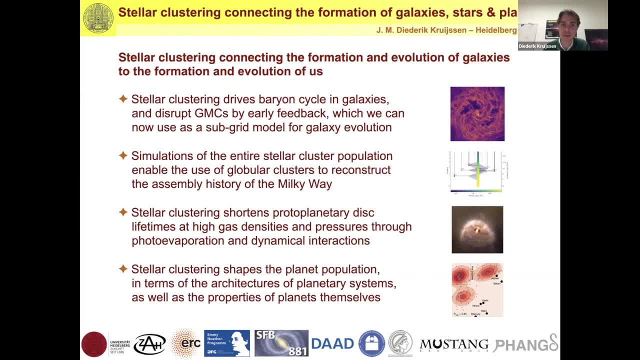 around those stars protoplanets and planetary disks formed, And their lifetimes are dependent on that degree of stellar clustering. especially at high gas densities and pressures, photo evaporation and dynamics truncate their lifetimes. Now, somewhat amusingly, it turns out. 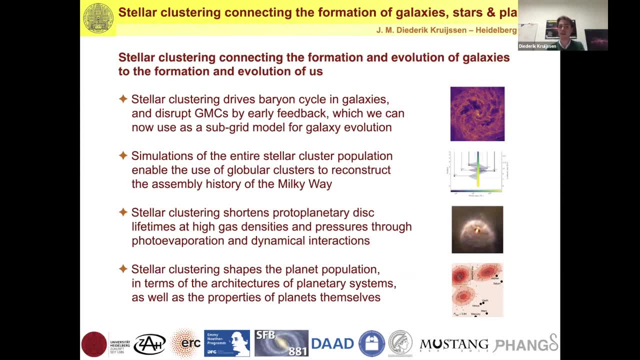 that the individual planet populations seem to be affected by this as well. They're shaped by stellar clustering to some degree. We don't understand why yet or how, but empirically the architectures of the planetary systems and the planet properties themselves are in line. 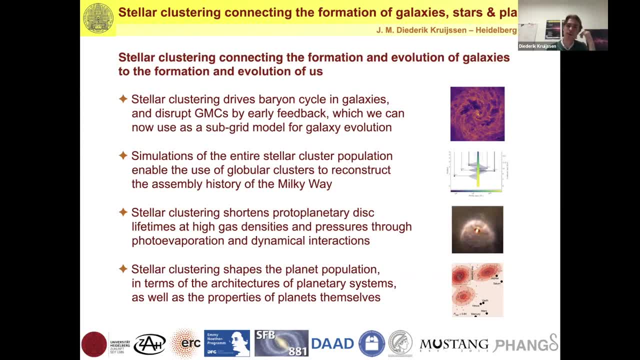 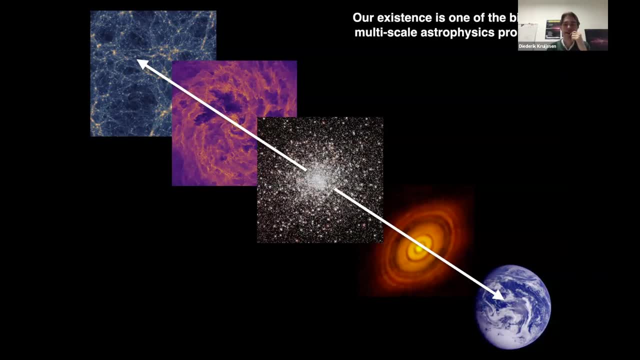 with the stellar clustering in their environment. So I started this talk by saying that our existence is one of the biggest multi-scale astrophysics problems And you know it's a real challenge to understand this, But I hope I have convinced you. 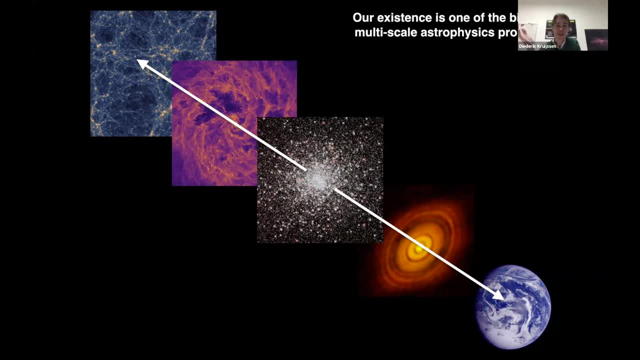 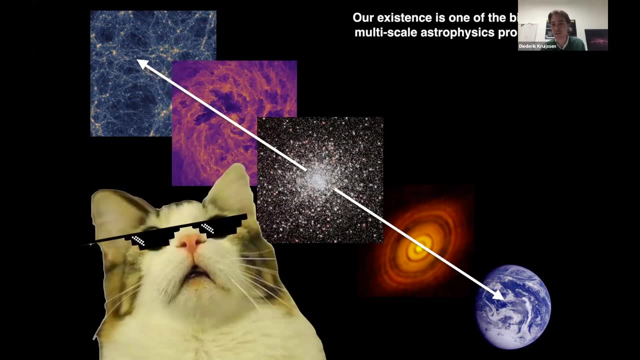 that this is starting to become a practical problem. We can actually start thinking about this, And that means that, when faced with this enormous challenge, I don't think we should look scared, but cool. We should relish the challenge and try and do. 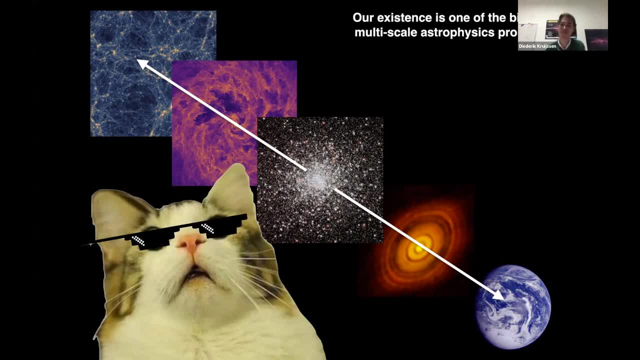 something with it. So thank you, Apologies again for running over. Well, thank you for a fantastically wide-ranging talk. We'll take maybe five minutes or so for questions now, And then we can go get lunch and Diedrich can run home. 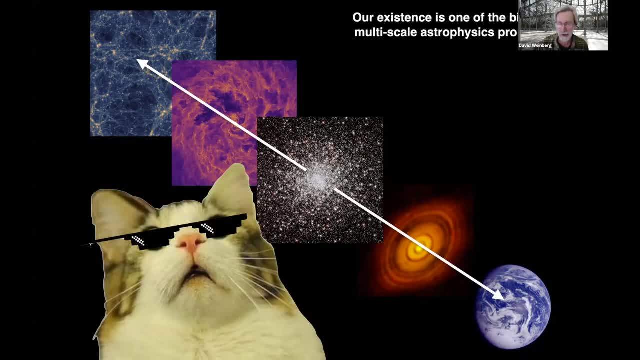 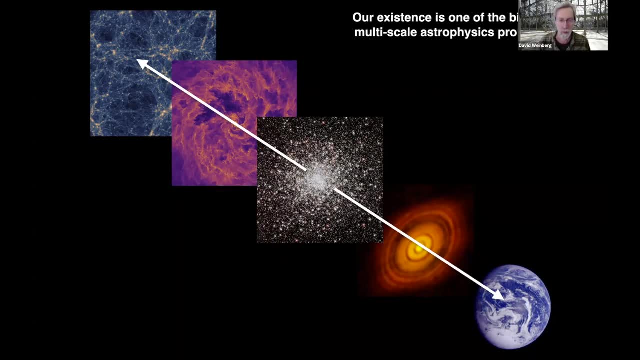 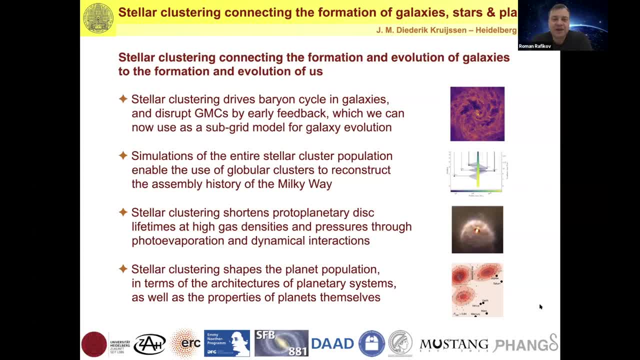 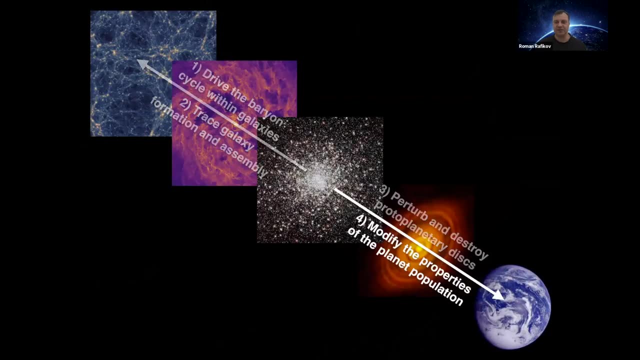 Very stimulating talk, Very provocative and interesting. I had a question about planets. Actually, this relation is over densities, So you seem to separate things into two kind of into binary categories by field and clusters. But how clustered are clusters Do you have? 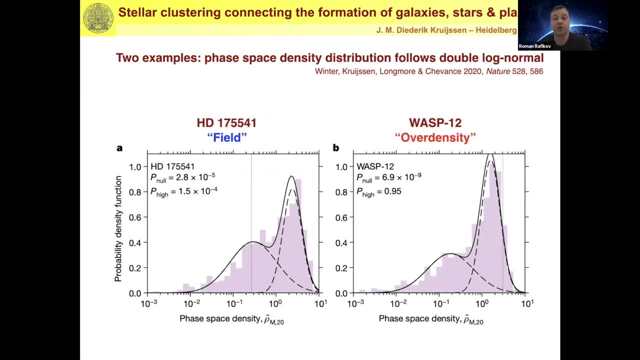 any correlation with cluster densities of all these parameters that you have shown, actually Multiplicity of planets, disk truncation and so on. Yeah, this is a really good question, And we the fundamental problem is is that Gaia is not necessarily complete. 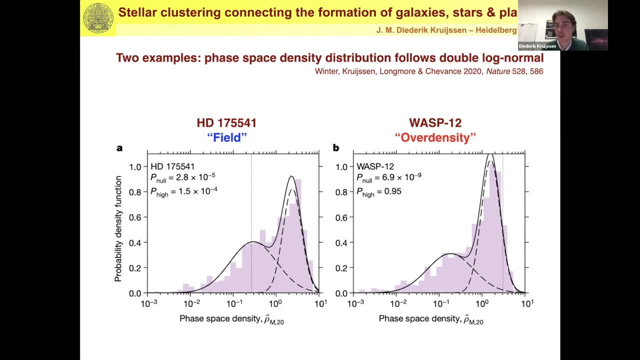 So when we calculate the phase space density here, we are dealing with a selection function that is not necessarily well described, And therefore what we've done here is we've actually here, on the x-axis, we always use the normalized phase space density. 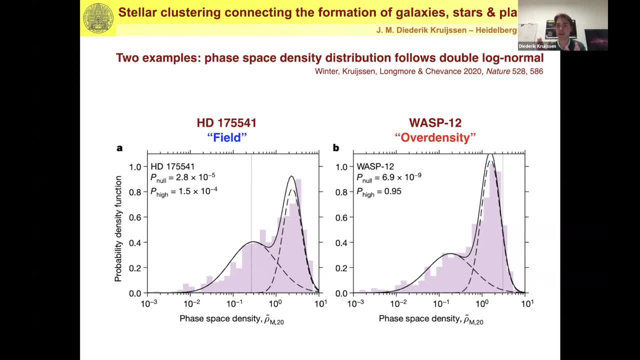 So we always normalize by the mean within the volume that we're considering. Now. that means you can do your decomposition, but you don't know what the meaning is of the phase space density in an absolute sense. Now, despite that, we've done what you just asked, because we just wanted to know, right? 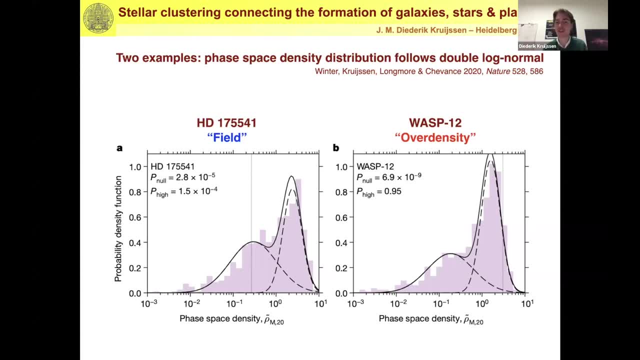 Okay, if we just let's say we pretend that everything is complete, then this, even this normalized phase space density, will have some meaning. Let's just use that. It turns out that we do not see. I don't think we have the statistical significance, like the sample size, to see trends with that number, at least not for the population at large. 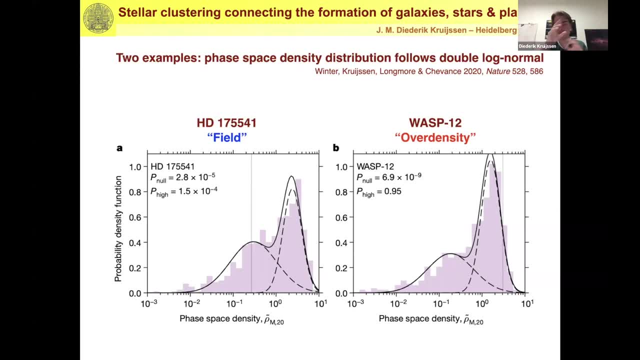 There the problem is. the initial problem is the heterogeneity. actually You've got many different types of planets. This is becoming a problem. What you can do is you can try to cut to specific planet types and see if then there is a trend with that number. 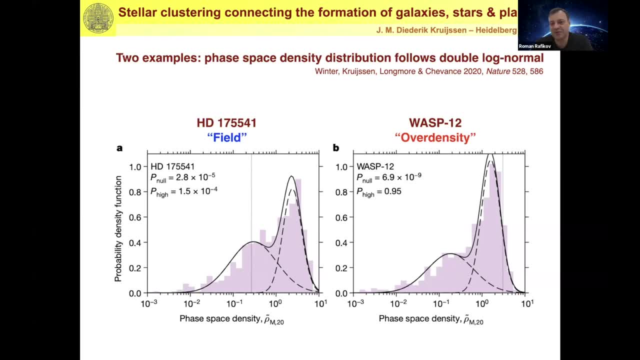 But yeah, then you run into the small sample size. Have you seen trends with hot Jupiters? I mean, the one thing you showed is very striking for hot Jupiters. Do you have any trend there? We have not looked at that yet. No, 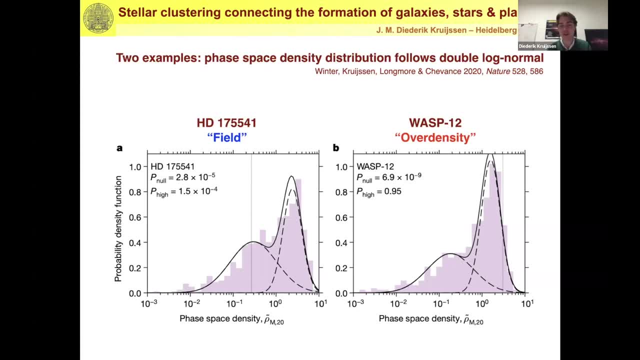 So I don't know that We have not made the cut of only looking at hot Jupiters and then trying to do all those things. No, it's basically. we're a small group of people and there is a very large number of things that you can do. 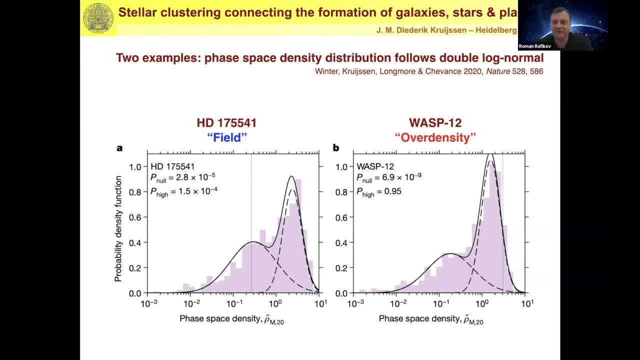 So, okay, this is a really good idea. I will try to look at this The next few days and actually ping you if I have an answer. Okay, great, Thank you. Thank you, Scott. So could you say a little more about what you think the physical origin of the, the dichotomy between the field and overdensity in phase space, is? 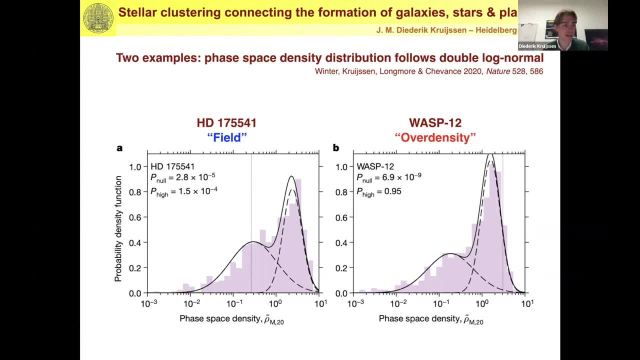 That's a really good question I've had with the team. we have had a long history of going back and forth between a lot of things here. The problem is that birth overdensities should disperse much faster, really, even in phase space, even as co-moving groups should disperse much faster than the ages of these planetary systems. 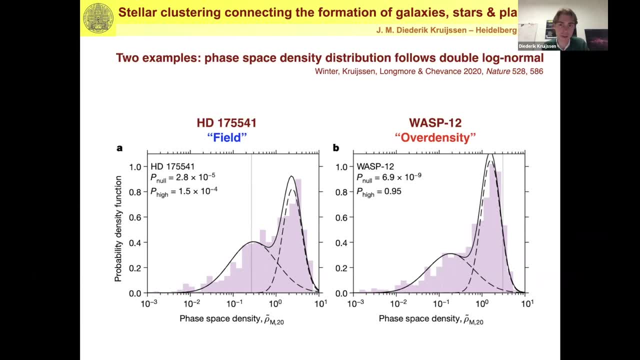 And indeed we've done a preliminary crossmatch of the planetary systems and their neighbors in our catalog in Gaia with chemical surveys, And if you look at the chemical abundances in these overdensities they actually fine. They're a bit smaller than just across the fields but it's definitely not a single chemical population.